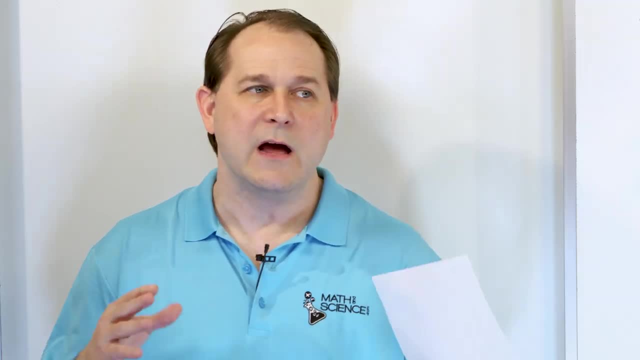 you're going to earn in interest, or how much debt you're going to pay in terms of interest on the loan. And that exponential function is very, very simple to understand, But it does take a little bit of talking about it for me to help you understand what it means, And I can tell you this: 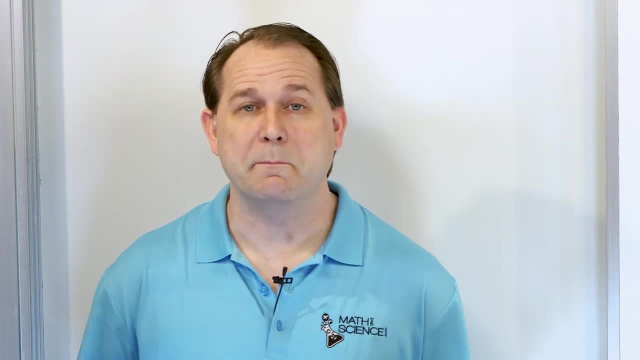 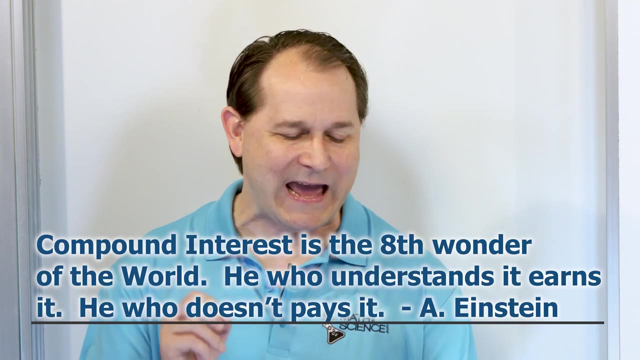 and you can probably understand this by listening to a quote from somebody you've probably heard before His name's: Albert Einstein. Einstein said the following thing: Compound interest is the eighth wonder of the world. He who understands it earns it, but he who doesn't. 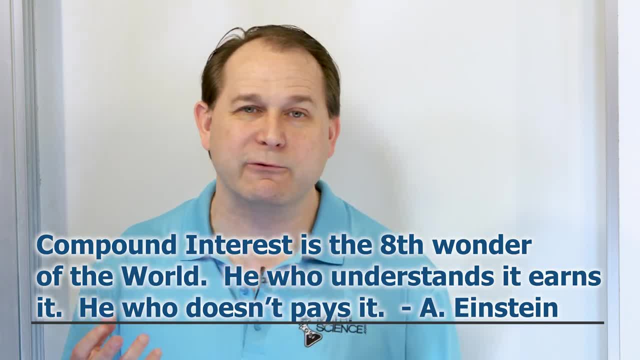 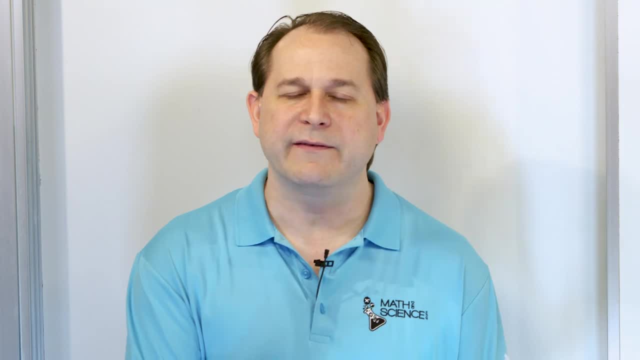 understand. it pays it, And what that means is really, really important for you to understand. compound interest governs how much money you're going to earn when you put money in the bank or when you invest money in a retirement account or just in the stock market to try to acquire. 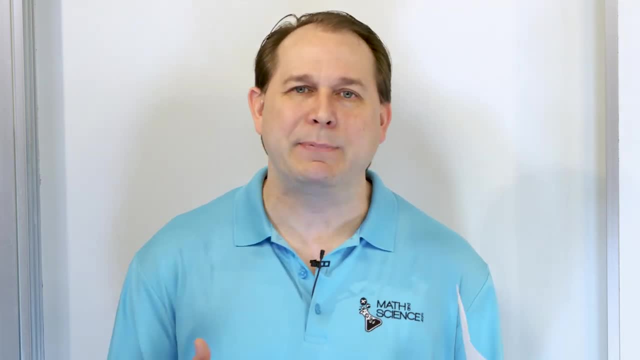 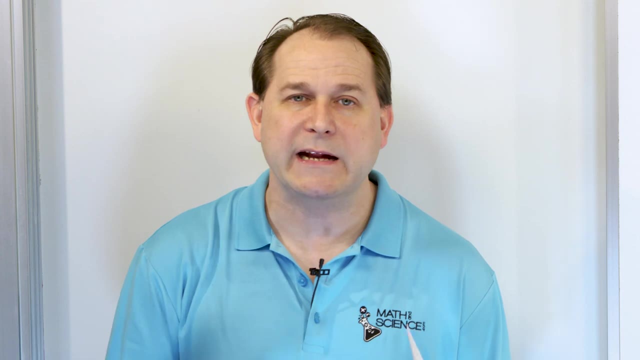 wealth. So that compound interest is an exponential function And we've been learning about exponential functions. You know the shape of that exponential function goes up very rapidly. So if you save money, it's the eighth wonder of the world because it gives you more and more and more money over. 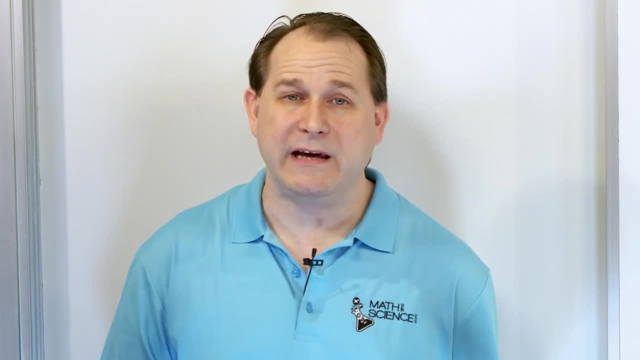 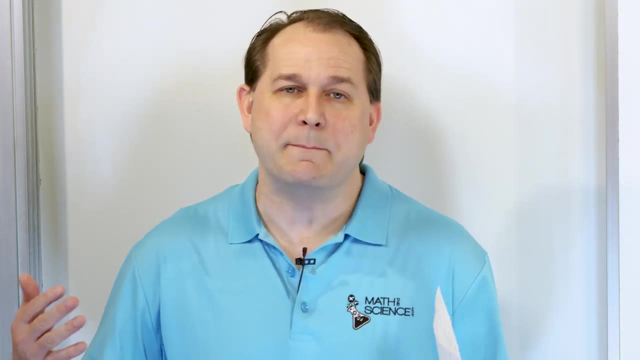 time. But he who doesn't understand it pays it. And what that means is, when you buy a house, you have a loan and that loan acquires, you have to pay interest on that loan and the amount of money you owe goes up and up and up, also exponentially with time. Anytime you buy a. 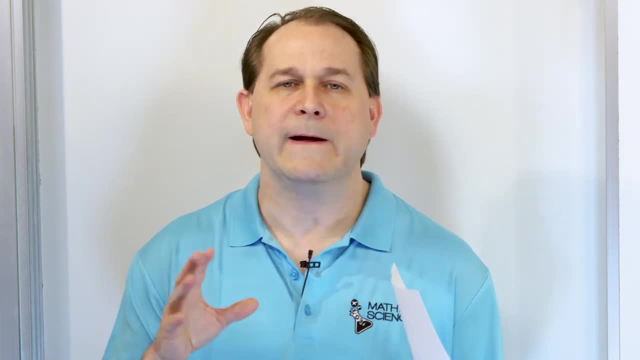 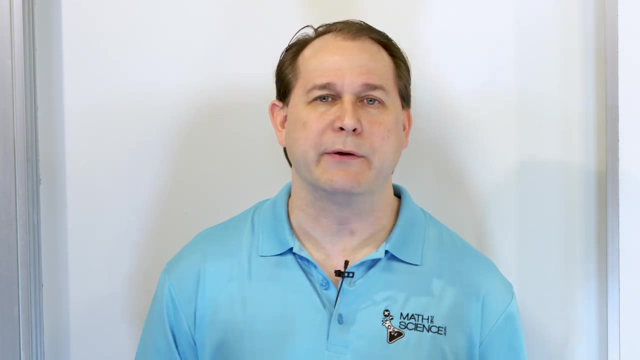 house and you take a loan for a car or a student loan for university, you have to pay interest, and that's exponential also. So it really is one of the most practical things you could possibly learn and one of the most important lessons here. Now we're going to start off by asking: I'm going to 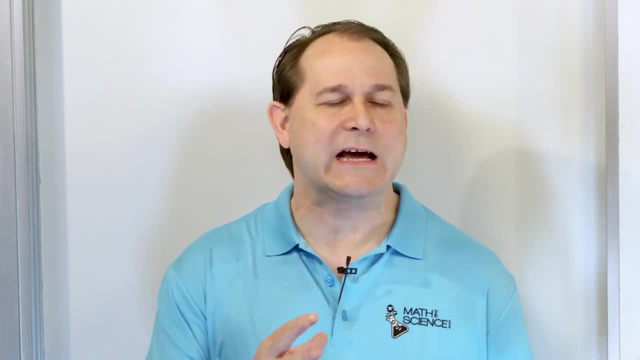 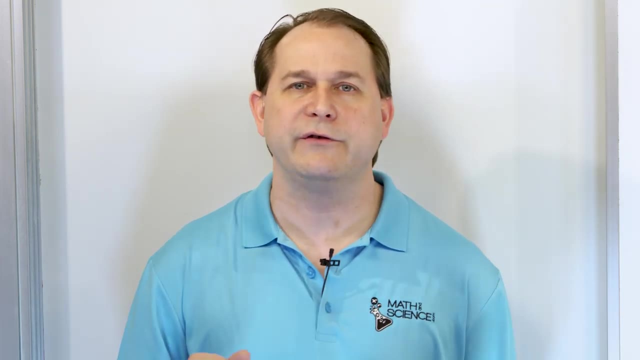 ask you a question and I'm going to demonstrate powerfully why compound interest and exponential growth of money is so important. I'm going to give you two choices. For 30 days over a month- 30 days- we're going to do the following options. I'm going to give you two options. Option A is 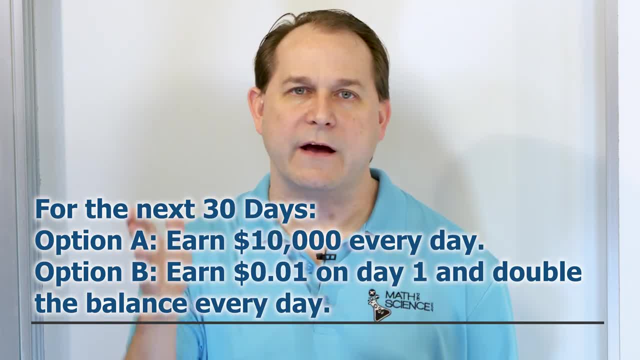 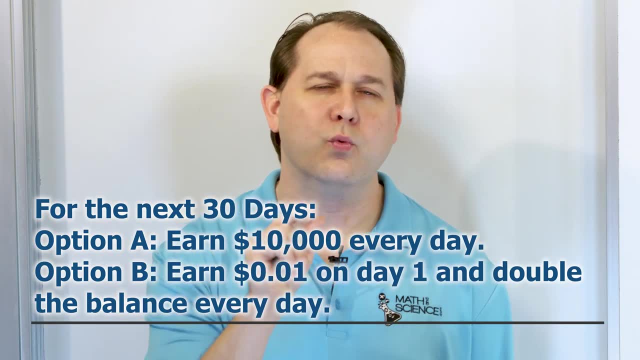 I'm going to give you $10,000 every single day. So $10,000, $20,000, $30,000, $40,000, that's how much money you're going to earn if you choose option A, Option B is, I'm going to give you one. 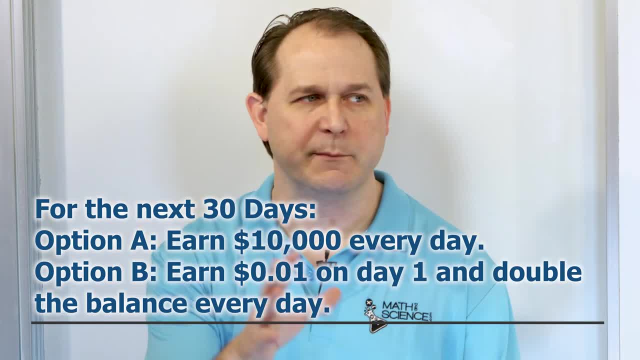 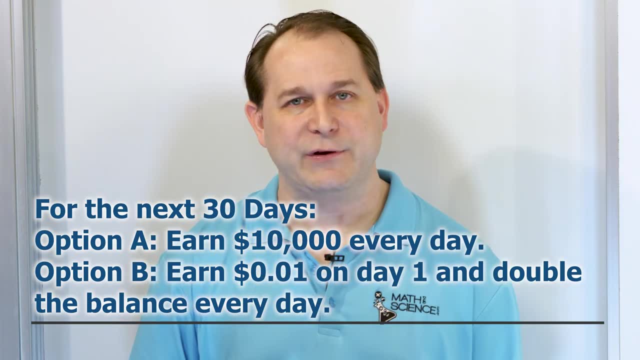 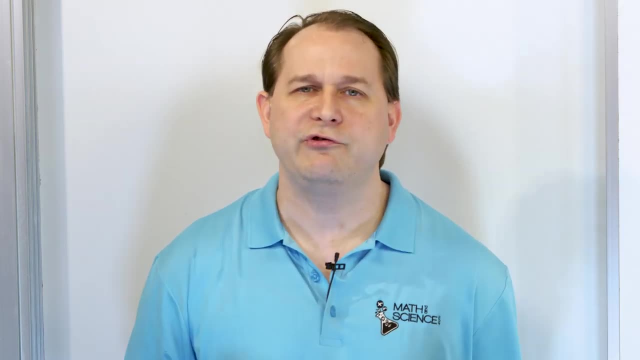 penny, which is one US cent, or you could pick some other currency. one cent, right, One tiny is double that every day, So it'd be one cent, Then the next day you get two cents, Then I would double again and I would give you four cents, and so on. So what would you choose? for 30 days just? 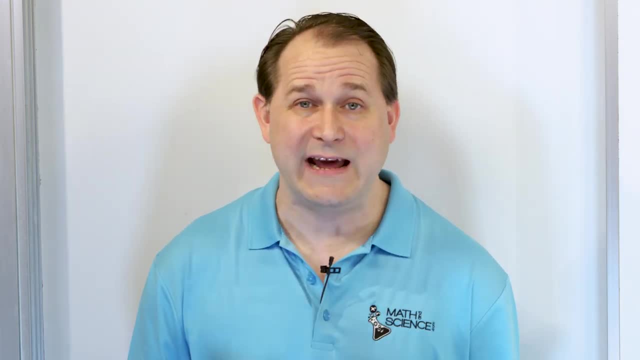 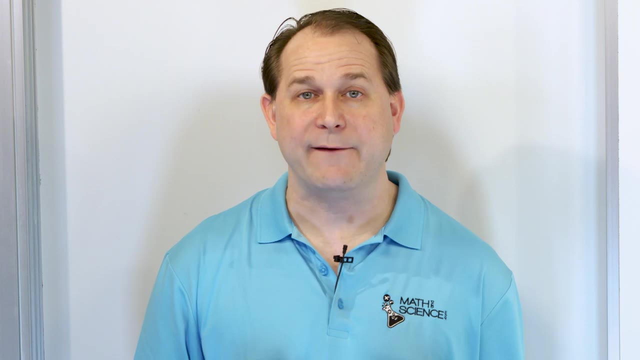 for one month. Would you pick the $10,000 every single day, And at the end of the 30 days you would have that much money, or would you pick to go with the one cent per day, And I will double that balance every day? only for 30 days, though. How much money do you think we're going to have? 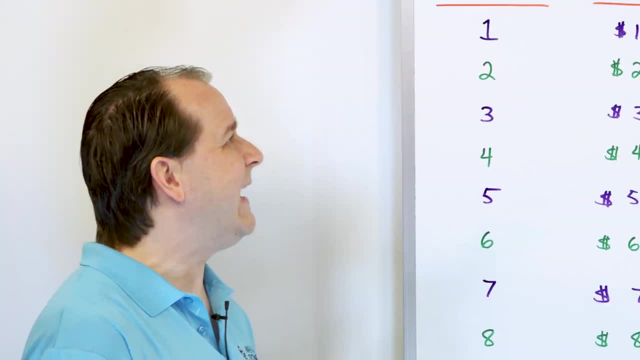 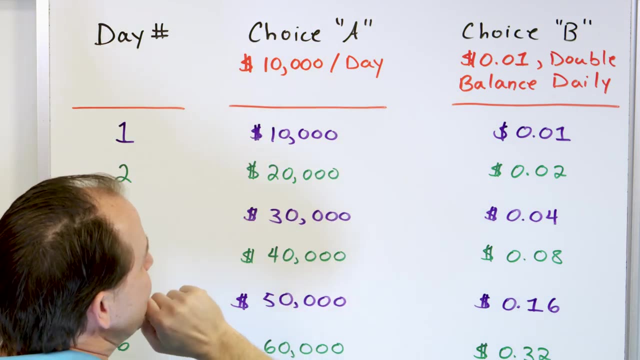 at the end of the month for each of those cases. All right, so here we go. Here's what the answer is. Here's day number one A is: I give you $10,000 a day. You start with $10,000 a day. Choice B is: I give you only one. 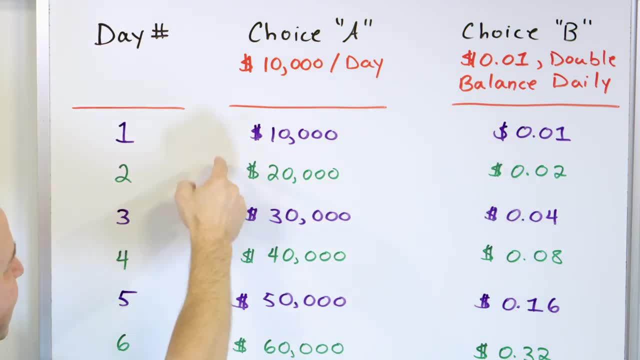 penny. But then on day number two, I give you another $10,000.. That's how this column works, right? But choice B: I double the previous balance. I double that and I give you two cents. All right, then we go to day three. Obviously, every day you go down this column it goes 10,000,. 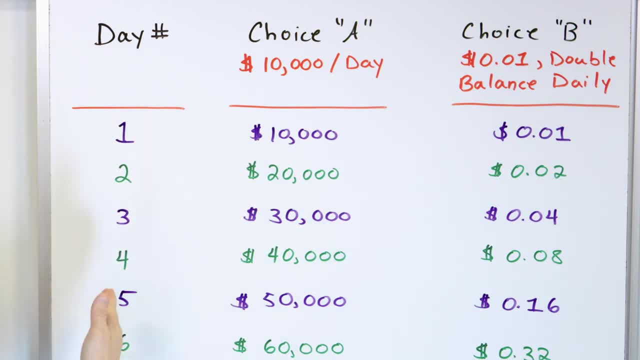 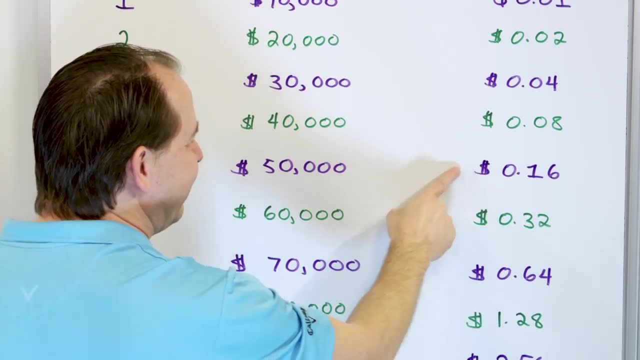 20,000,, 30,000, all the way down to $100,000 at the end of 10 days. Choice B: I keep doubling it: One cent, then two cents, four cents, eight cents Then 16 cents. You see, right here you'd have $50,000 and only 16 cents in this column. 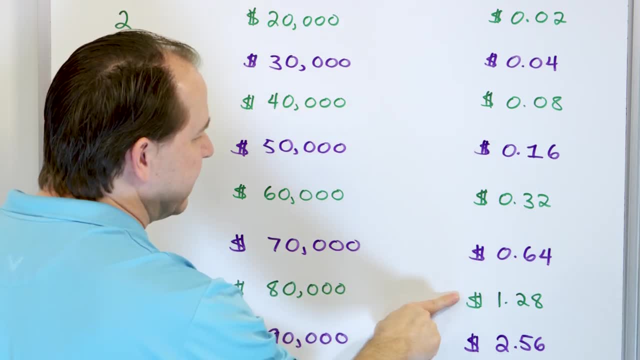 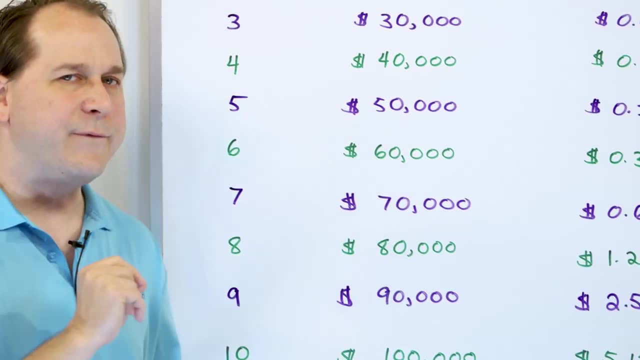 Let's keep on going. If you keep doubling, you get 32 cents, 64 cents, $1.28,, $2.56, $5.12.. In this column you would have $100,000.. So if you were going to stop this at 10 days, you would. 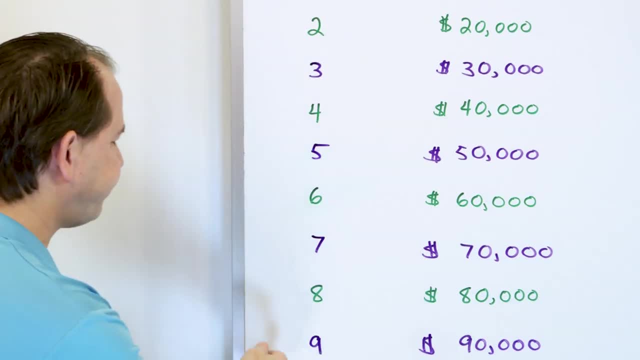 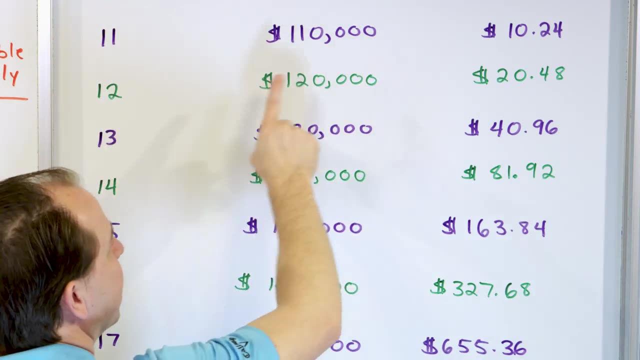 obviously want to take the $10,000 a day, but let's keep going. All right. what's going to happen on day number 11?? I'm going to have $110,000, but I doubled that $5.12 over here. 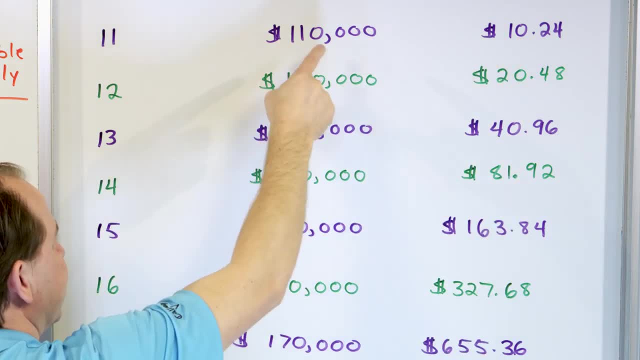 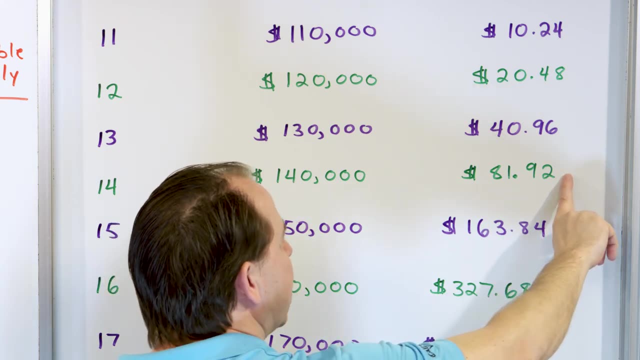 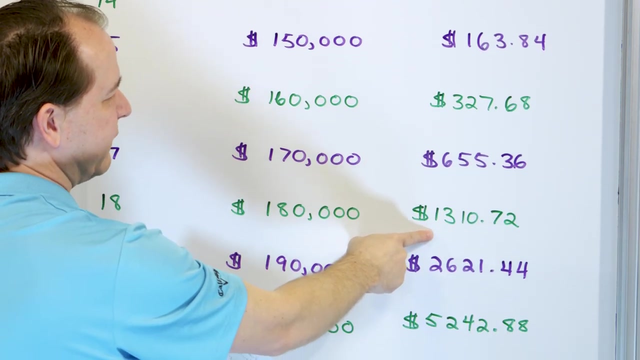 to get $10.24.. Now in this column I keep going down down $10,000 a day. but in this column I go from $10.24, $20.48, $40.96,, $81.92,, $163.84,, $3.27.68,, $6.55.36, $1,310.72, $2,621.44,. 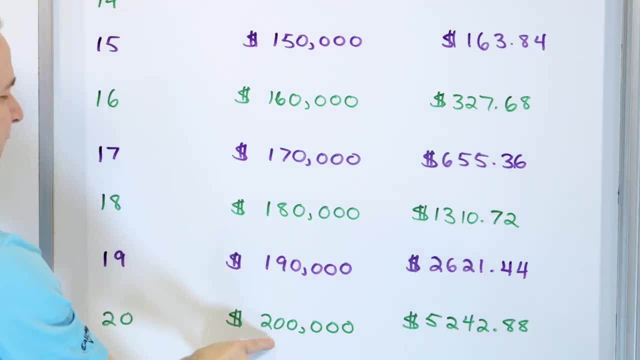 and then $5,242.88.. Still in this column I would have $200,000 compared to only about $5,000, after day 20.. So obviously, if you were going to go only to 20 days, you would want to take the. 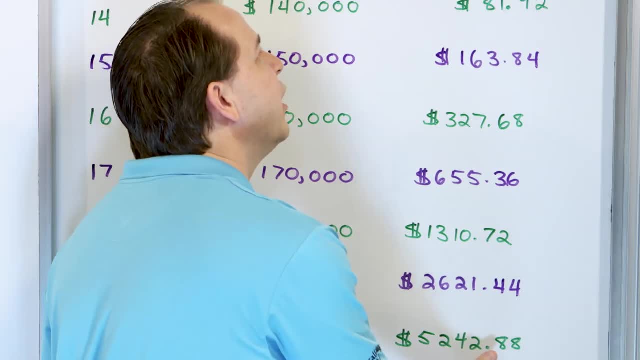 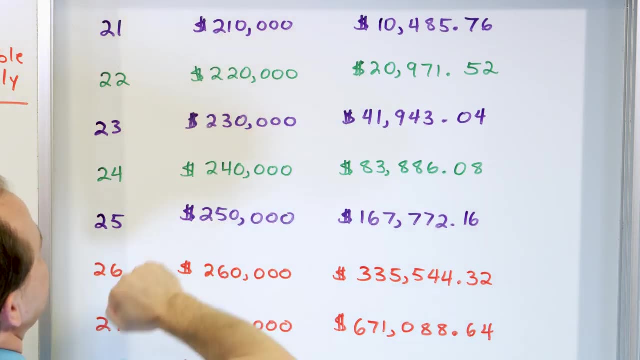 column A to get your $10,000 a day. Let's see what happens when we go into the tail end of the month here. Here's where we start seeing some interesting things going on: Day 21,. I have $210,000 here. 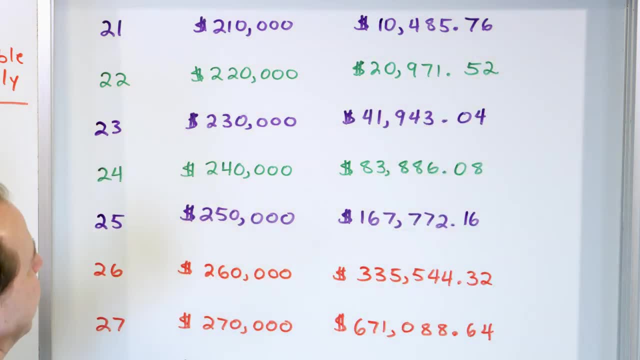 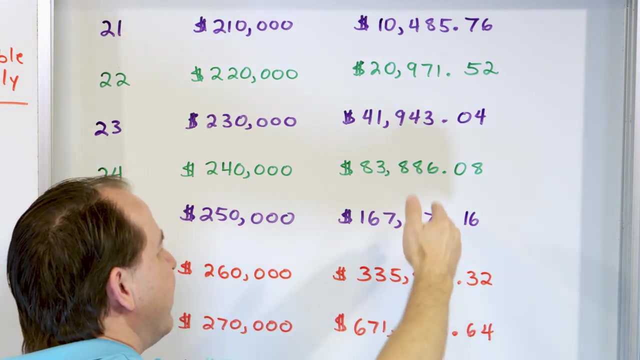 but in this column I've doubled that $5,000 to $10,485, and then I've doubled again to $20,000 and some change $41,000 and some change $83,000 and some change $57,000 and some change compared to the $250,000 I would have here. Here in red is where the right. 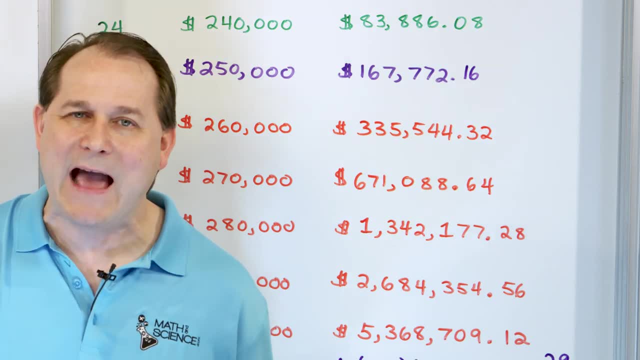 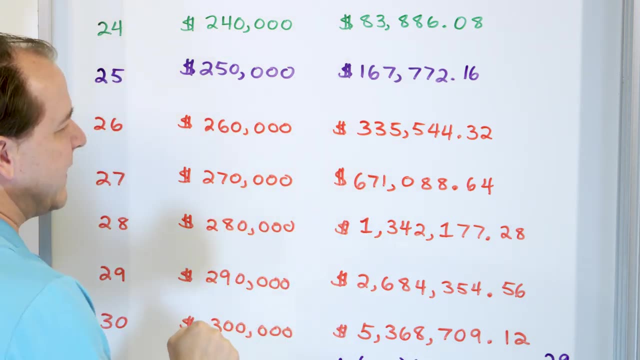 hand column starts to beat the other column. So actually, if you run this thing out to 30 days, what's going to happen is you're going to run through $300,000, $335,000, then $671,000. 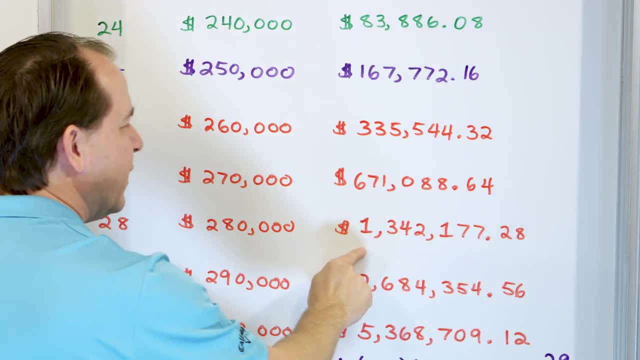 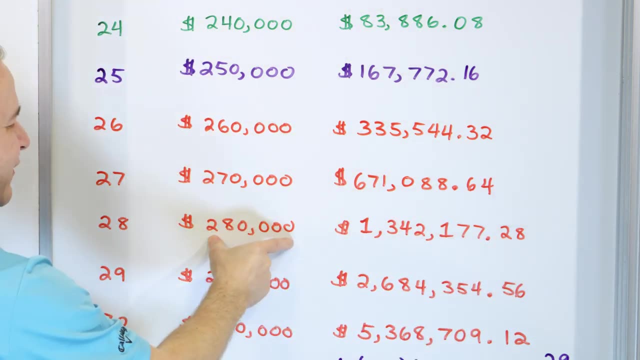 Here's where you hit $1,000,000 on day 28.. $1,342,177.28 on day 28,, as compared to just simply $280,000.. We double that, we get $2,684,354 and some change. and on day 30, we double that again to. 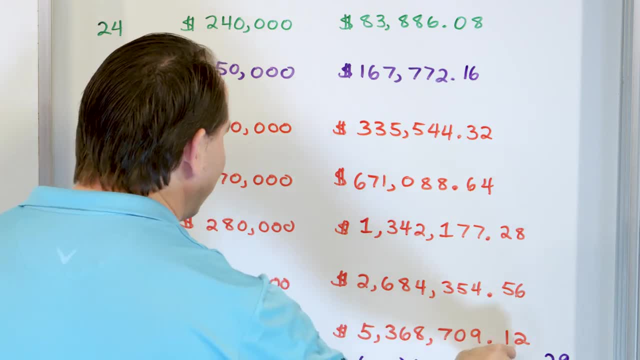 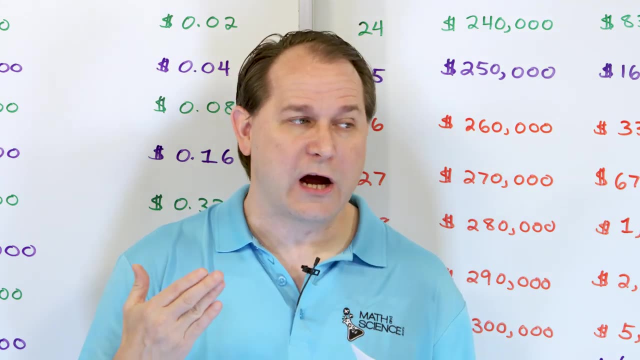 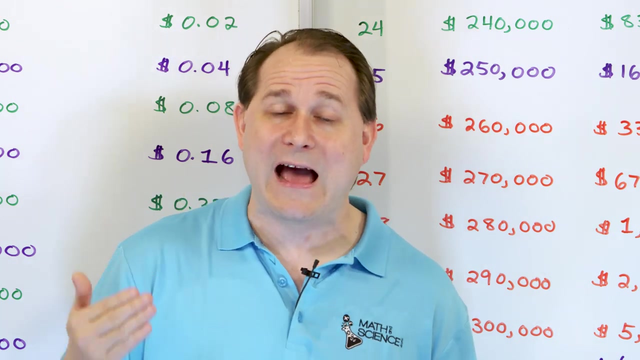 $5,368,709.12, as compared to $300,000.. It's incredible and it comes about because the right hand column. it isn't really obvious when you first look at it, but the column where I'm doubling every day is actually an exponential growth of money, Even though it 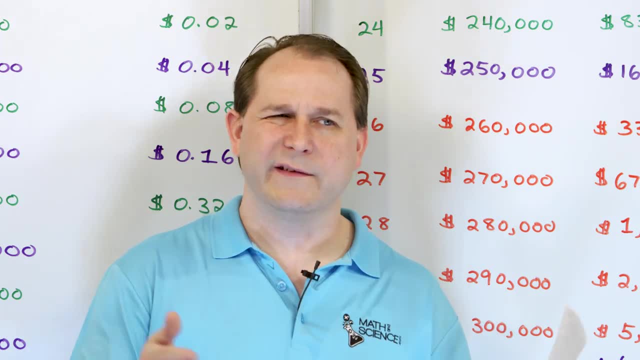 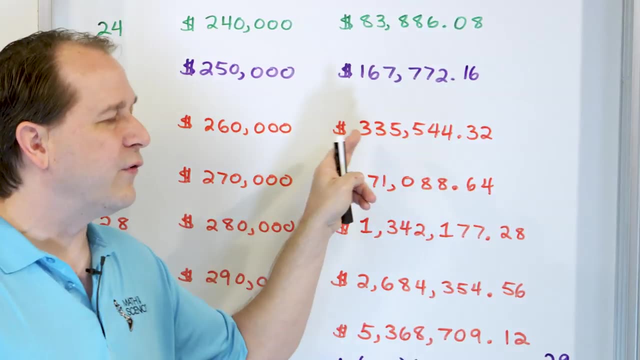 doesn't really seem like it at first. it seems like, well, who cares? One cent, two cent, four cent, whatever, I don't care about that. But really, when you get down to a certain critical number of days in the future, you overtake the linear function. This is a linear. 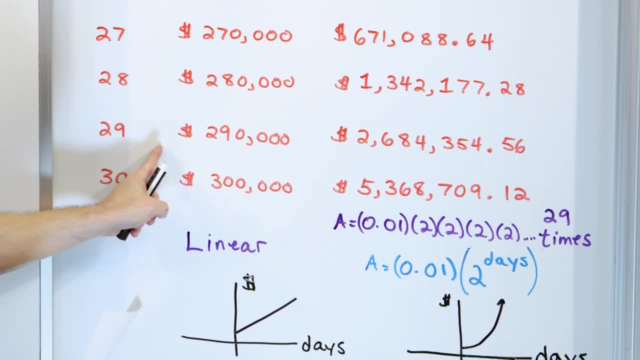 function because I'm gaining the same amount of dollars every day: $10,000,, $10,000, $10,000.. So this is a linear growth of money. If I graph it days versus dollars, there's just going to be a. 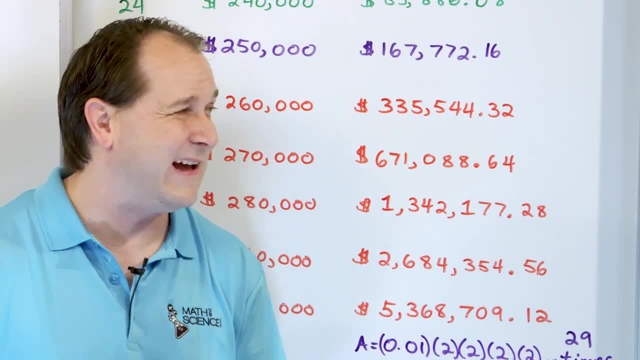 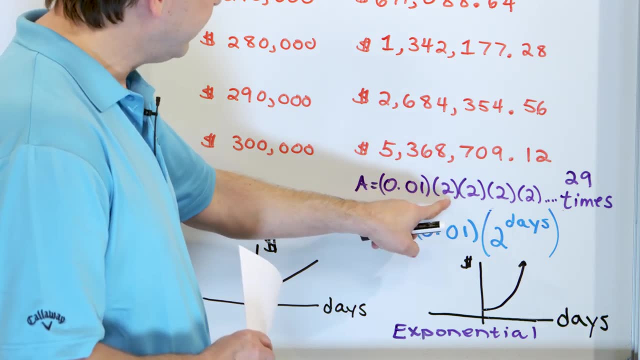 straight line because I'm gaining a constant number of dollars every day. But this column? notice what's happening. What I did is I took the one cent and on the first day I multiplied by two cents, And then the next day. after that I multiplied by two again, And then the next day. 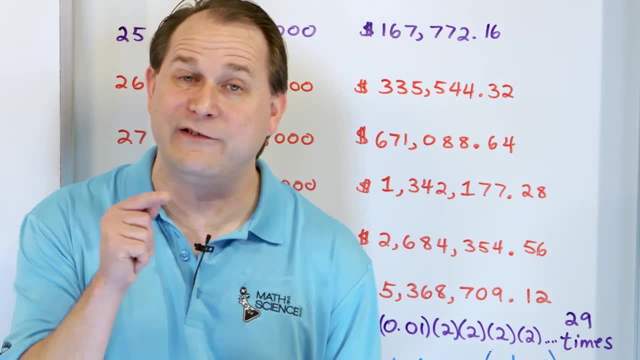 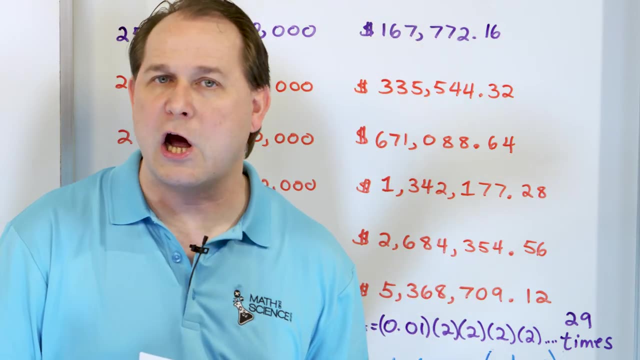 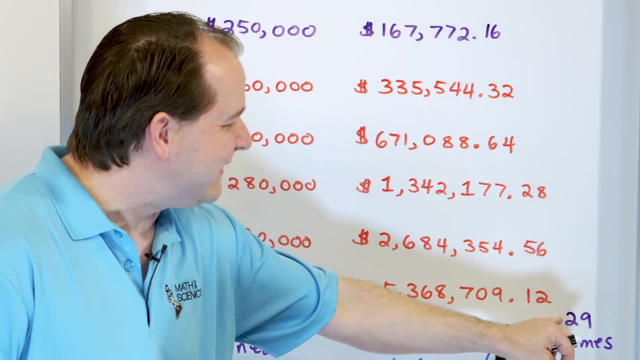 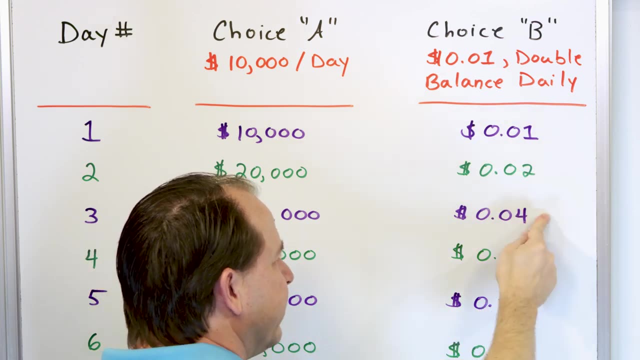 the right, Just times, two times two every day. And you do that 29 times, because on day one, the first doubling, when I multiplied by two, this was one doubling, then this was another doubling, and so on. So, even though there's a difference between the two, there's a difference. 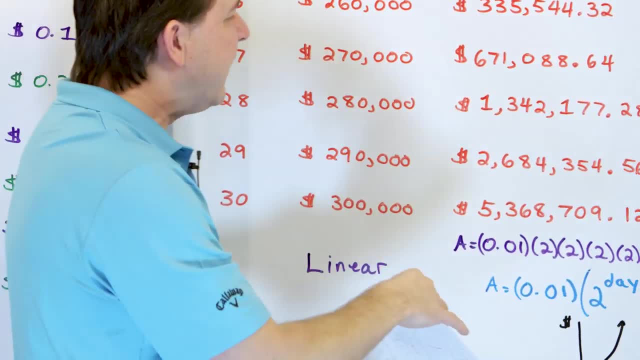 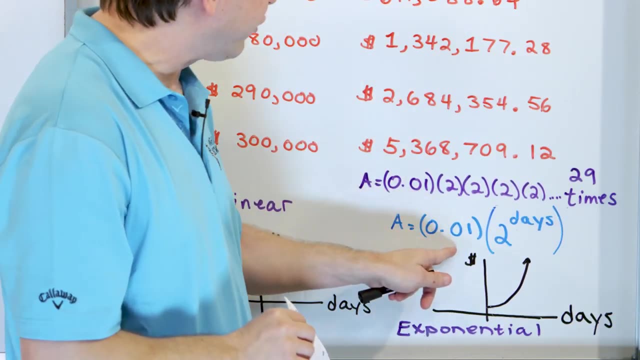 30 days. there's actually 29 doubling periods, And so if you multiply by two- 29 times- you will get the $5 million answer. okay, So in terms of when you look at what you have here, it's one cent. 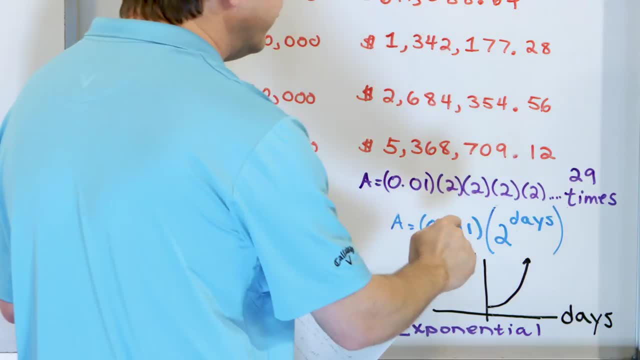 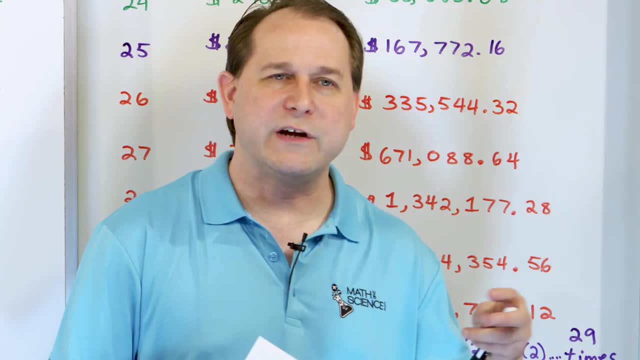 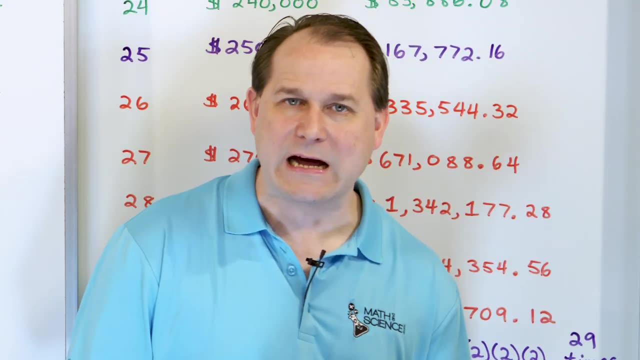 the second number. I'm multiplying by the second number, I'm multiplying by the second number. So if you don't want to do the times two times two, deal in your calculator. just grab a calculator, take two, raise it to the power of 29,, because that's how many doubling periods we had, And you 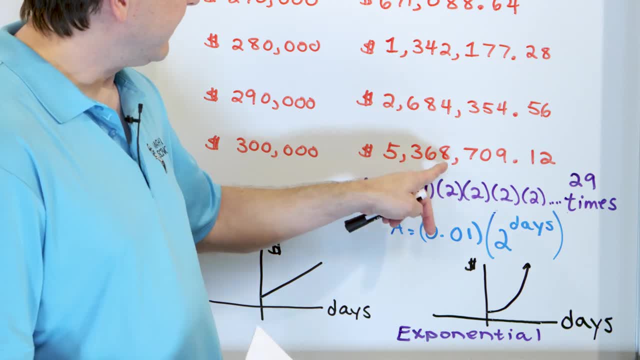 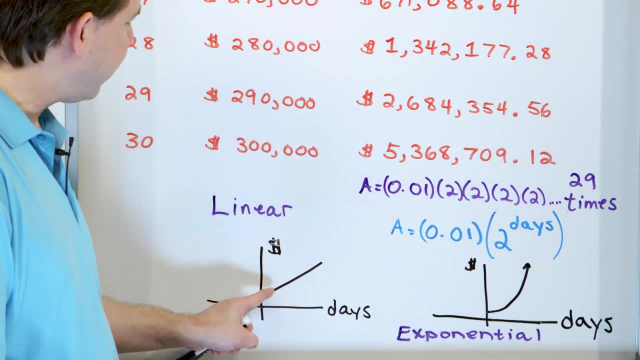 take the answer and multiply by one cent, You will get 5,368,709,12.. And if you were to plot the money that you get as a function of the days in comparison to the linear, it's going to look exactly like an exponential function In the beginning. here it grows very. 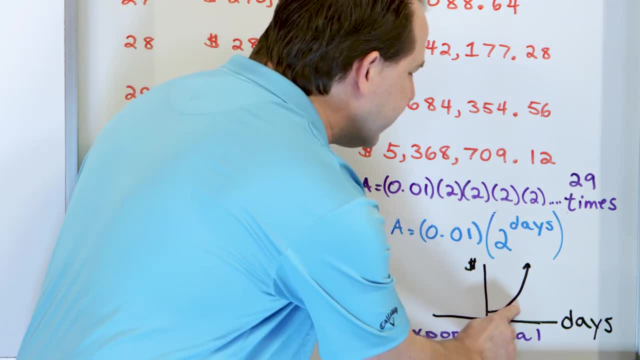 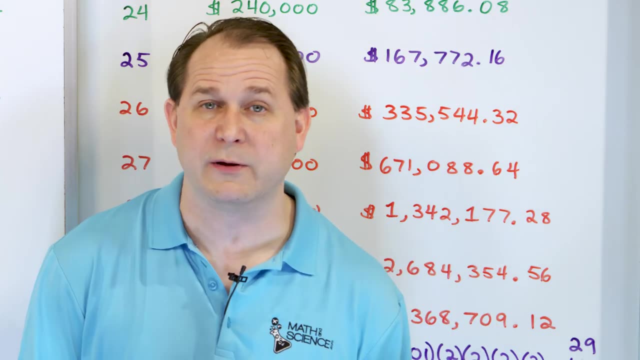 very slowly, which is what we saw. But then, once it hits a critical value, it starts to take off. And in those last what one, two, three, four, five days of the month is when you earn incredible amounts of money. So what does this mean? It doesn't mean. I'm trying to teach everybody. 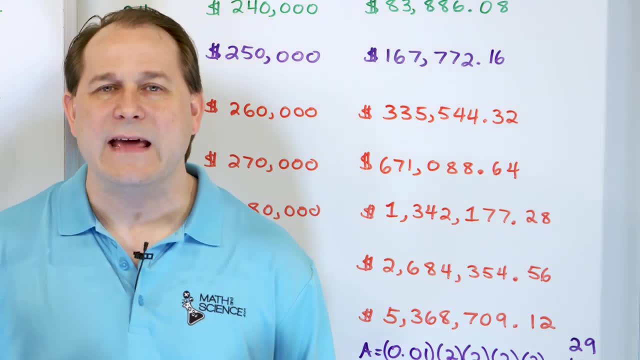 to be greedy. It's just that the number one question I get in math is: what is math useful for? Why do I care about math? When am I ever going to learn and use math in everyday life? That's what I get all the time, And here is your most practical. 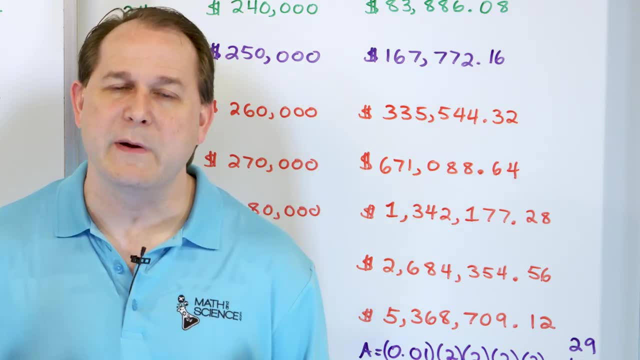 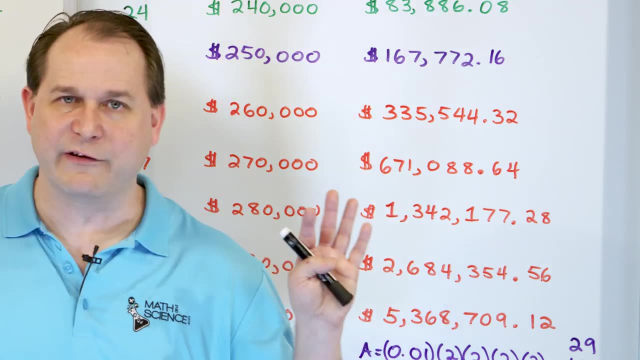 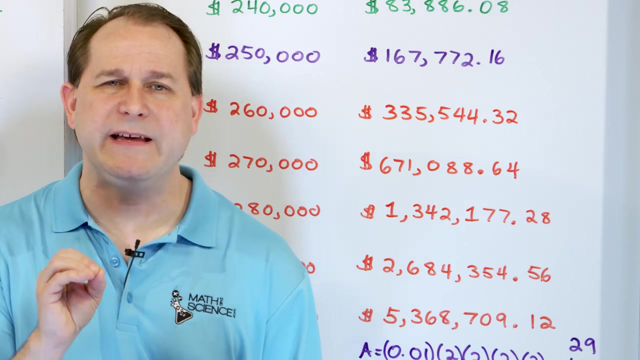 benefit and use of math in everyday life is your growth of money and your growth of debt is governed by an exponential function called compound interest. Now, this was a crazy compound interest, just for illustration purposes, But what I want to do now is I want to give you a more. 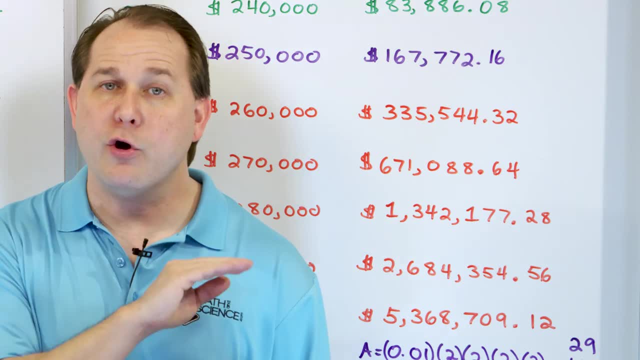 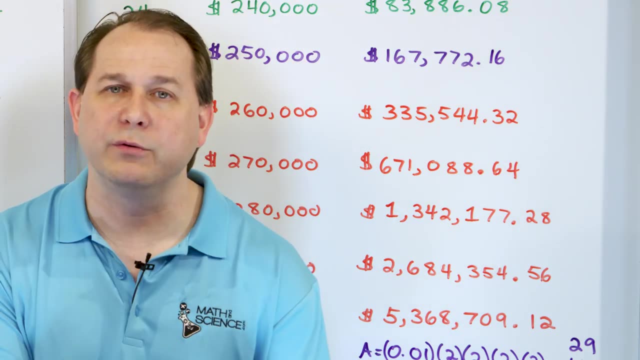 practical example to show you what the growth of money does over a realistic time period, with a realistic interest rate, And you will see this nice, beautiful exponential function. And then I want to go dive more into the math And I want to show you what the growth of money does over a 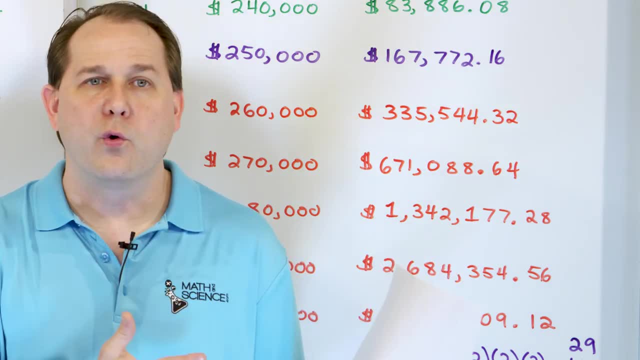 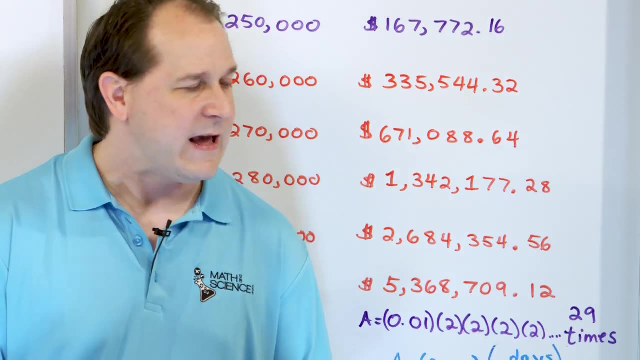 realistic time period with a realistic interest rate, And I want to solve a couple of problems and really show you what the formula is for compound interest and where it comes from, And also that you will then know and see that it is an exponential function Anytime you have an. 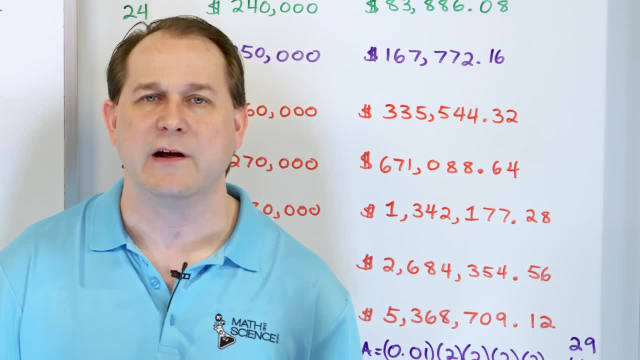 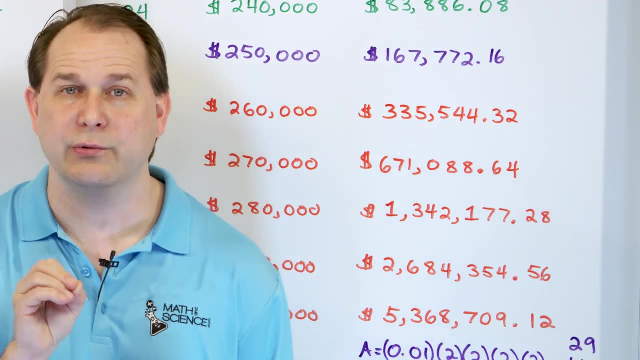 exponential function. you will always, always, beat a linear function, no matter what, as long as you give it enough time. So let's go off and do the computer demo. We're going to do a computer demo here where I'm going to show you what's going to happen to a growth of money. Let's pick an. 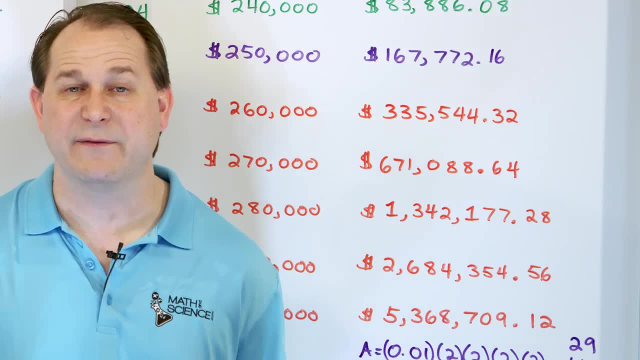 interest rate: 8% interest. Let's look over a period of time of, let's say, 40 years. Let's say you start working around 20 years old And then you go until you're about 40 more years. It's about: 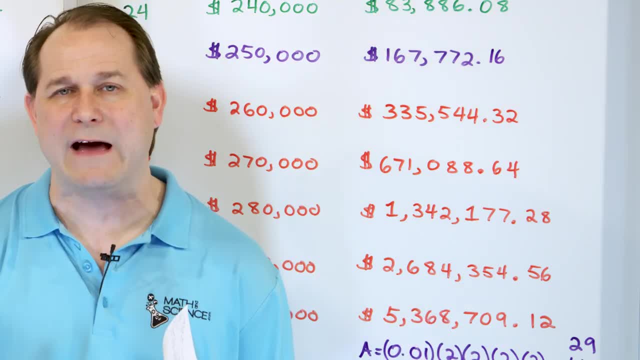 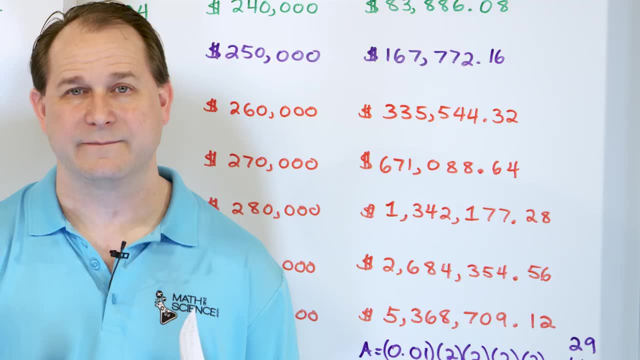 60 years old, when most people start to retire. Let's see how much money you'll have if you start saving early. a small amount of money with compound exponential growth of money in the form of interest. Hello, welcome back. So here is a website. It's a US government website called. 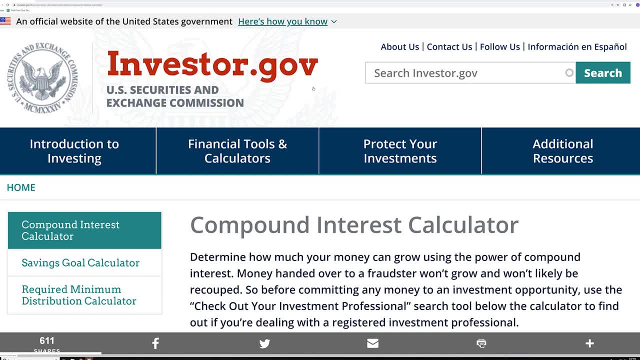 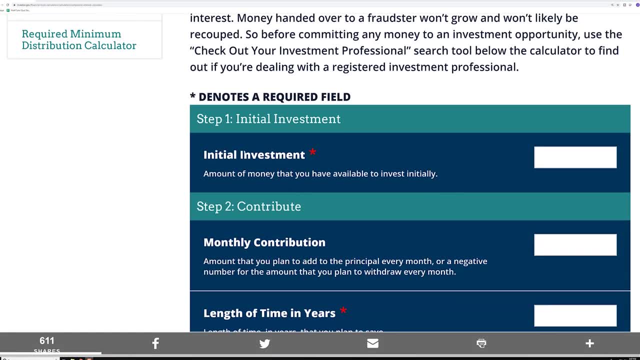 investorgov. It's free. Just go to investorgov. You can do everything. I'm about to show you here. What we're going to do is look at a realistic example. let's say you have an initial investment. Let's say that you're 20 years old. You have your first. 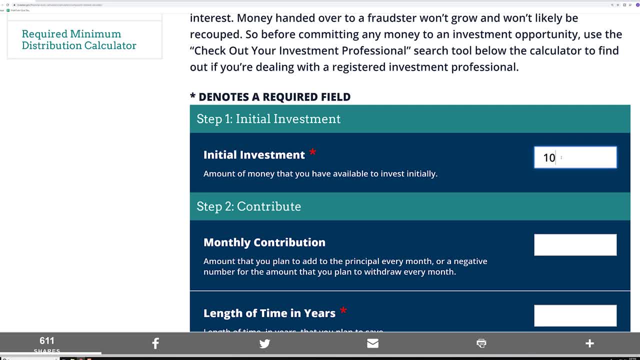 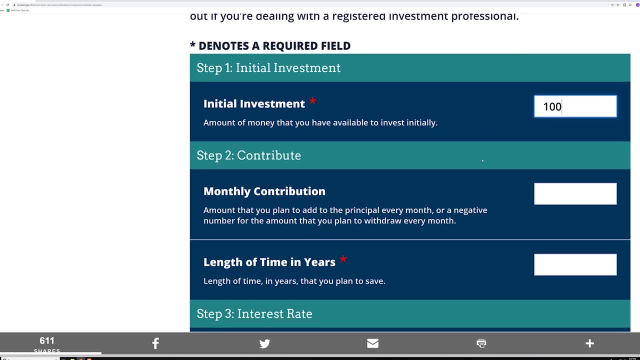 you know, I guess good job and you start to try to save some money. Let's say you start this account with $100 or 100, whatever currency that you have in your country, Let's say $100.. And let's say: every month you take your paycheck and you save $100 out of your paycheck. Now 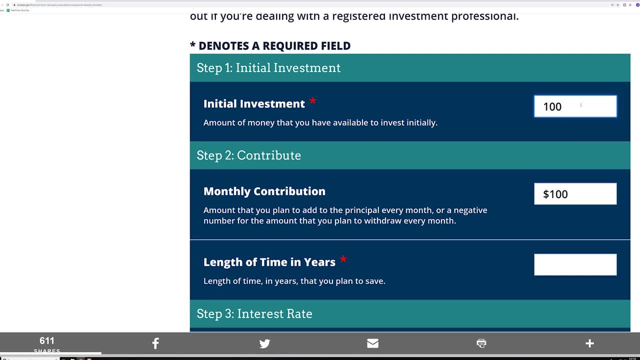 you might say $100 is a lot of money and it is a lot of money, but $100 is something like you know, a few dollars a day. It's like three. let's say $3 a day. There's 30 days in a month. That's like $3 a day, a little over $3 a day. It's like a coffee. 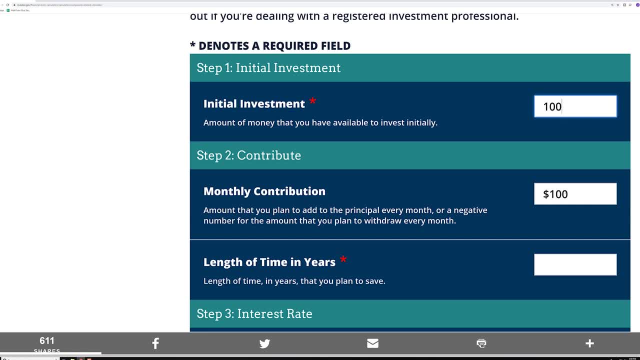 you know, stop getting your coffee, you know, once a day, All right, And so you save $100 a day. Now let's take a look from 20 years till most people retire at around 60 years old. So let's. 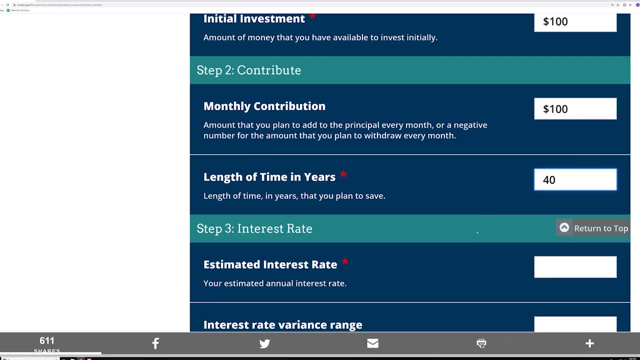 say that you save this and you do this every single month for 40 years. and your interest rate? let's take a look at and calculate it for an 8% interest rate Now, when you look at the US stock market, over the last 30 or 40 years, you've averaged about. 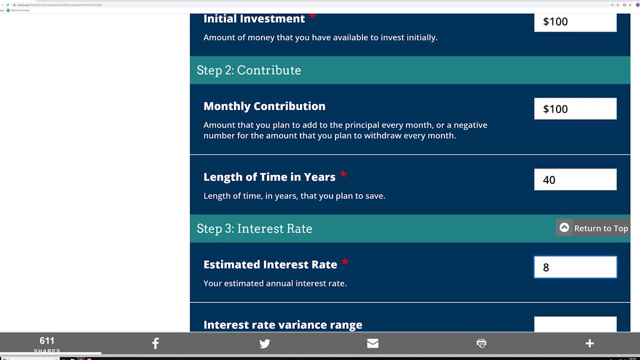 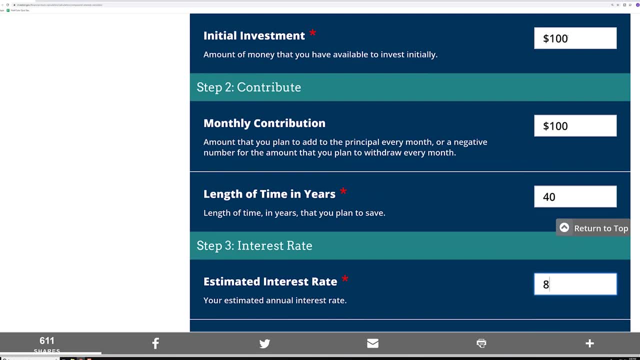 eight, seven to 8%. So you know, you may or may not agree with this number, but we're going to calculate based on 8% and that's pretty realistic based on history. Okay, That's all you got to do. You have an initial amount of money. how much money you're going? 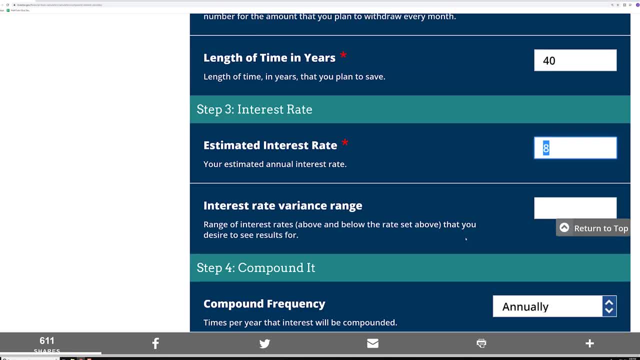 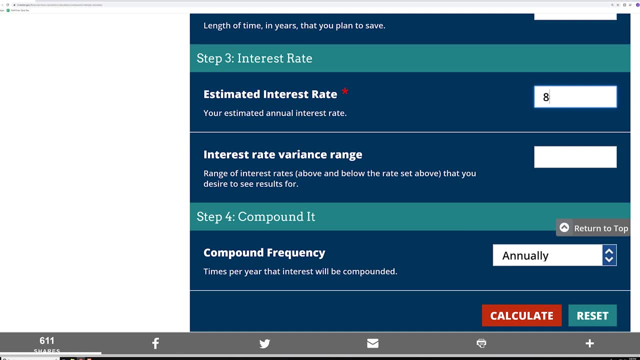 to put in every month how many years you're going to save it for and what is the interest rate, And we're going to compound it annually. That means we're going to calculate we're going to get 8% free money. That's the interest every single year on the money that we're putting in. 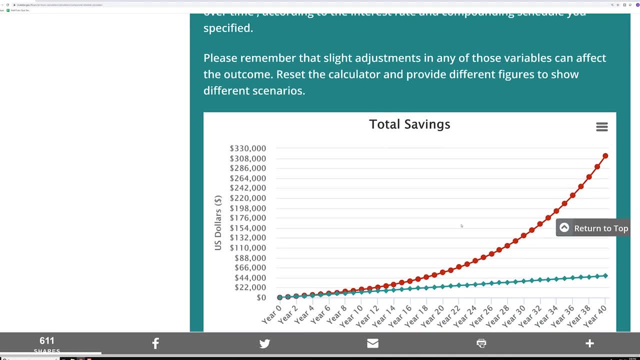 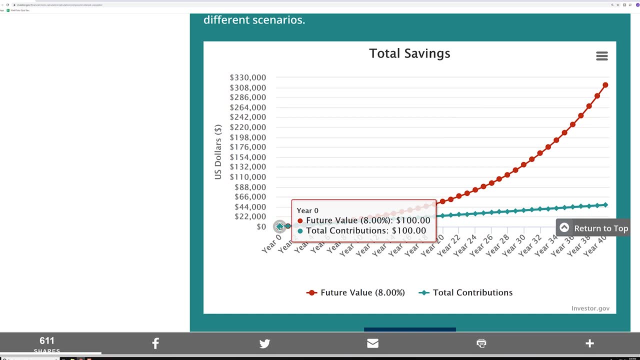 Let's calculate and see what the results are. All right, Let's take a look. Here is what the graph looks like. All right, On year you can see here: on year zero we saved $100 and the next year we actually. 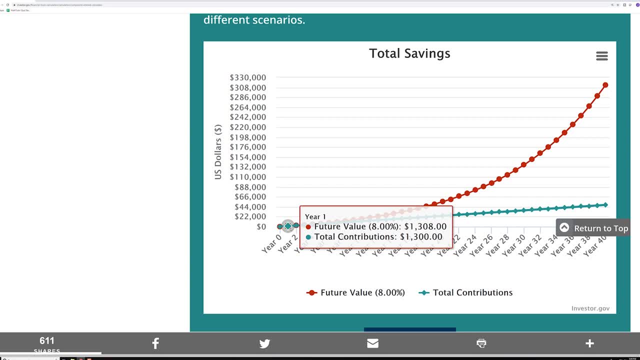 saved and we contributed $1,300.. We got a little bit of free money from the interest at $1,308. there You can see what's happening, though. As you go off and off and off into the years, the red curve is pulling away exponentially from the green curve. The green curve down here. 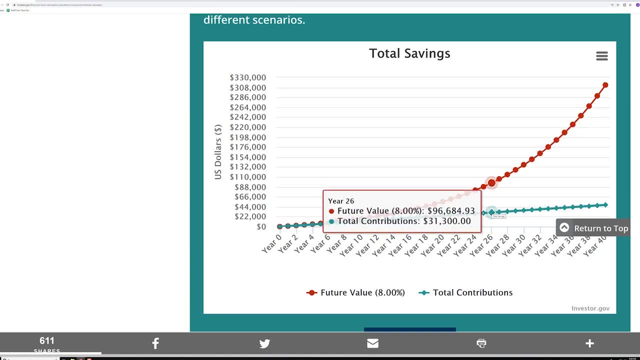 is the money that I'm putting in every month into that account. The $100, this green number is only the money I'm putting in every month. So I'm going to calculate that. I'm going to calculate that I'm putting in for my paycheck. The red money is all basically the free money I'm getting. 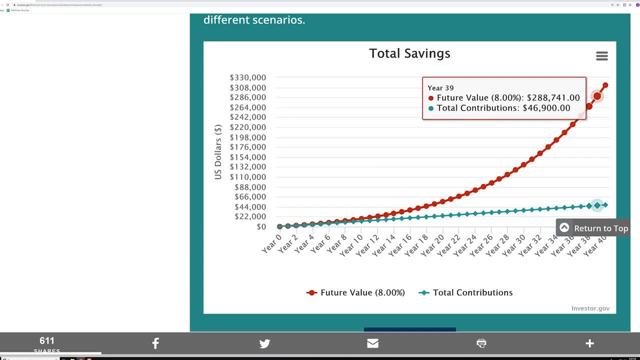 It's the total value of the growth of that money over time. So you can see after year 40, how much money do I have. I have $313,040 in this account, but I only actually put in $48,100.. So I earned. 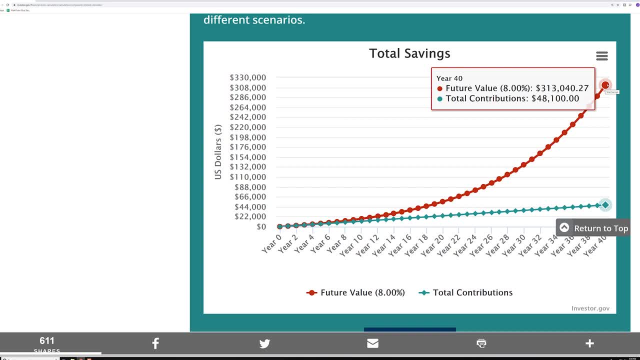 something like $250,000, something like that $260,000 totally, completely for free. But you see, in order to do that, there was many, many years here in the beginning where I didn't earn very much money, But after some critical amount of time it starts to pull away and starts to go. 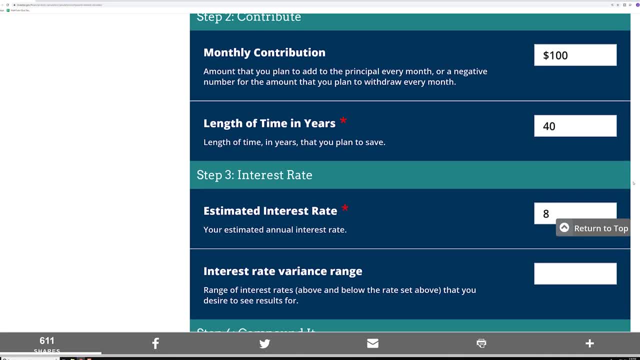 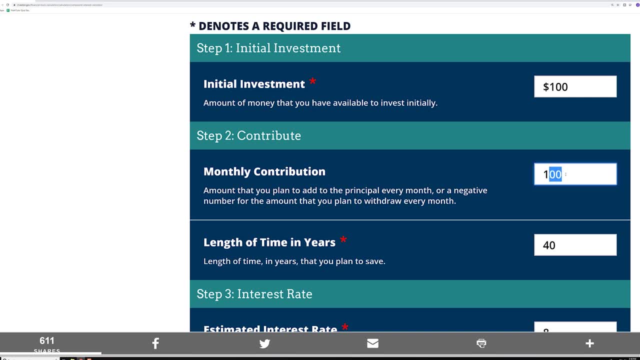 exponential on you All right Now, $100 a month is, you know, real money. you have to save, I agree with you. But whenever you get, you know, you go to university, you get a good job. I think it's. 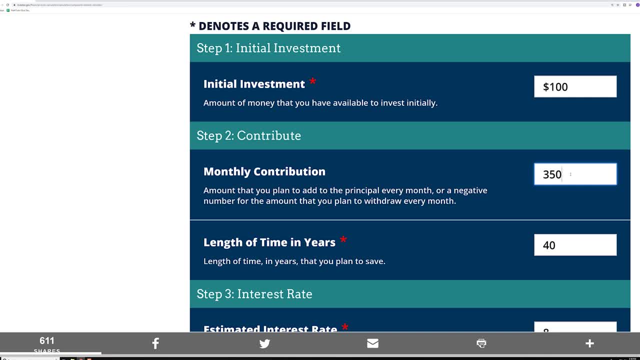 perfectly possible for most people to save around $350 a month. You might say that's impossible for me. Well, maybe it is, But $350 is what a new car costs. So instead of getting a new car and paying that monthly fee, you're going to have to save $350 a month. So you're going to have to save. 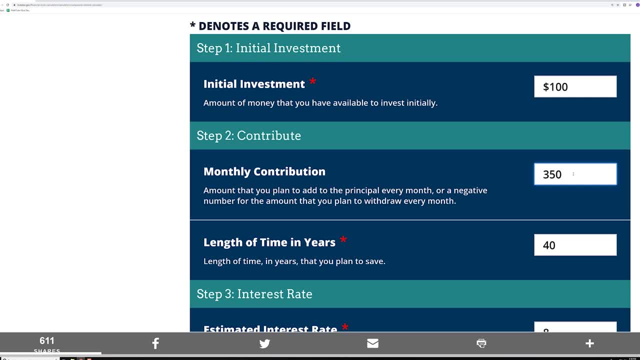 $350 in a new car. Maybe you get a used car, or maybe you just drive your car for a much longer period of time And instead of buying that new car, you just you take that money and you put it into this account. Let's see what would happen over 40 years. We start out with $100. We save. 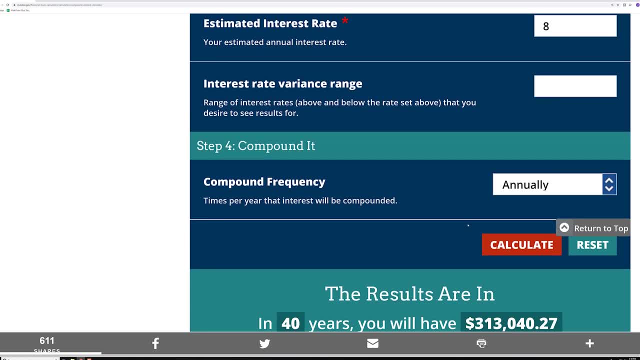 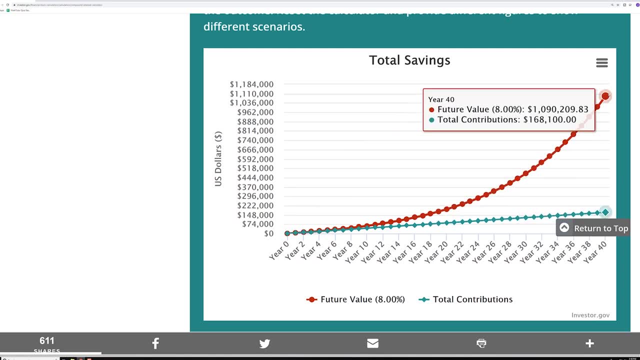 $350 every month for 40 years at this exact same interest rate. Let's recalculate it And what I have at the end of 40 years is now, instead of $300,000, it comes out to $1,090,209.. 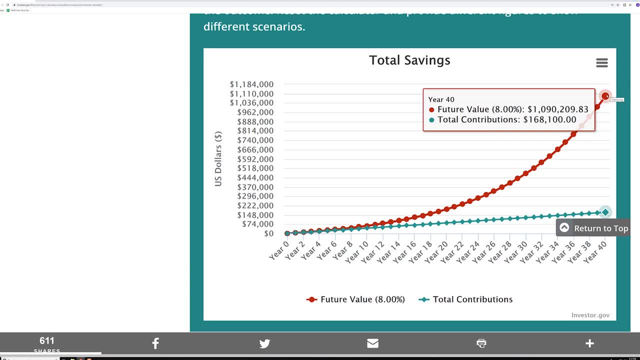 But the amazing thing is look at how much money I put in. I only put in $168,100.. So I save that $350 every month And yes, it was a challenge to save that money, But I put in $168,000. But I got. 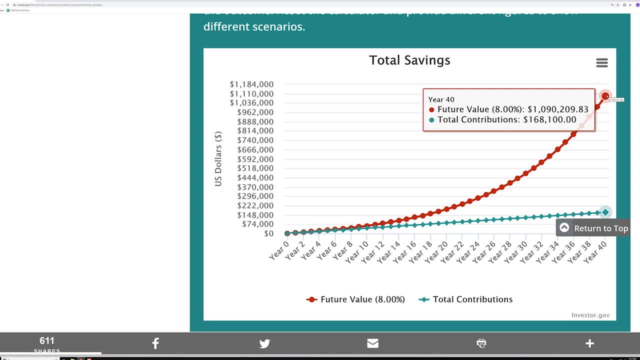 basically $850,000 for free. by doing that, This red curve is the exponential growth curve of all the free money that has come into my pocket by saving early and saving as much as I possibly could. And then you know, the green line is: 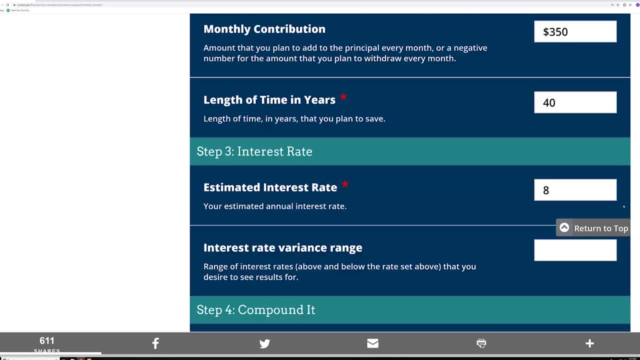 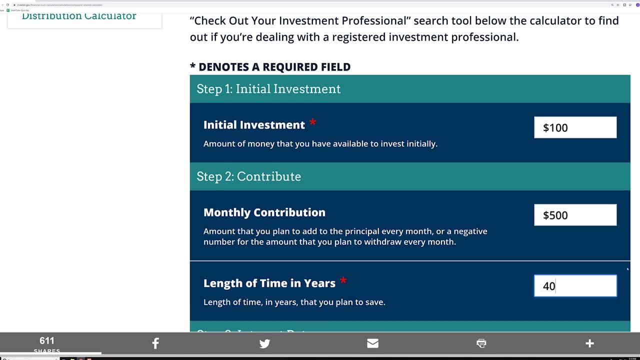 is just the money that I've put in. Now I know probably some of you are curious, So let's go ahead and do something, probably at the upper end of what you know some people can do. Let's say you could save $500 a month If you're married. you both have a job, you save some money And 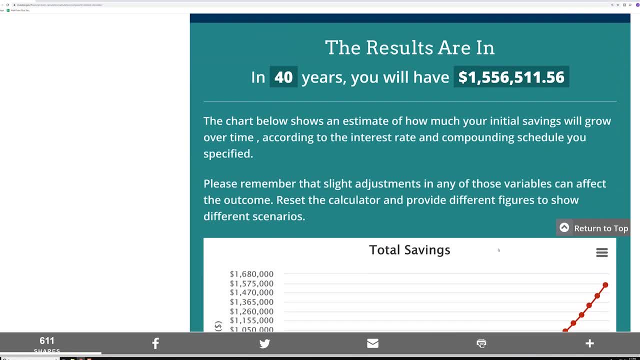 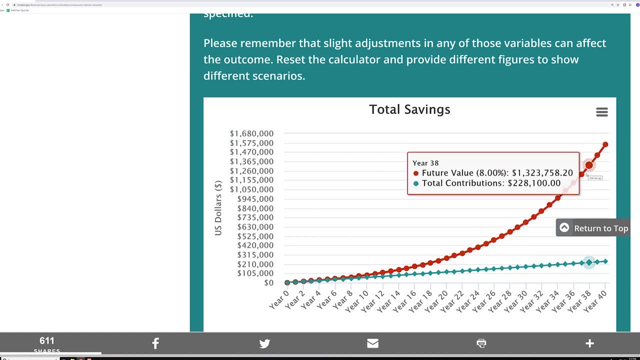 after, say, $500 a month, and you recalculate that at the end of that 40 years, you're going to have $1,556,000.. So we can play this game all day. I don't want to continue playing this game. I want. 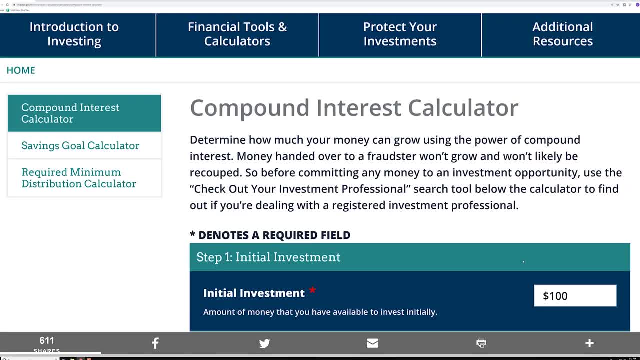 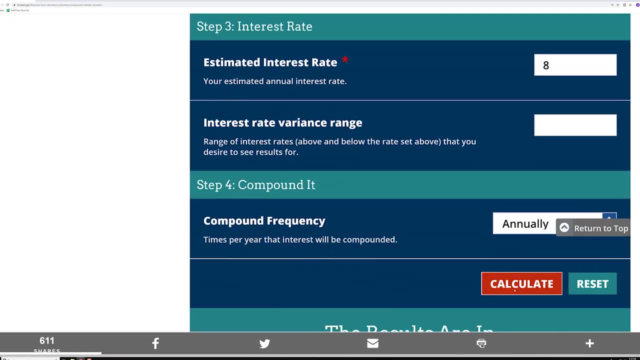 you to go to Investorgov and type these numbers in here. The point is is: maybe you can save $500., Maybe you can't. Maybe you can only save $50 a month. All right, let's see what happens. if you save $50 a month, What do you get at the end of that? 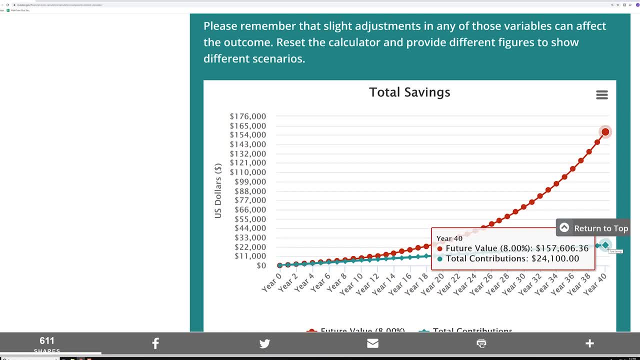 At the end of 40 years I only put in $24,100. But this account is worth $157,600 by saving $50 a month. That's something like $2 a day, $1.80 a day or something like that. to save that much money. 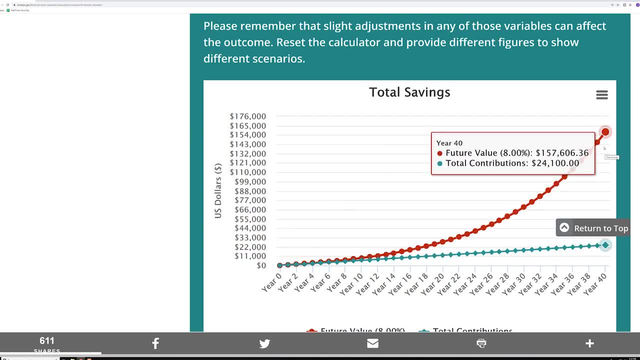 This is the power of compound interest. It's the power of the exponential function, And you can see that it does look like an exponential function. So what I want to do now is go back to the board and dive into where this curve comes from and how to solve problems that deal with. 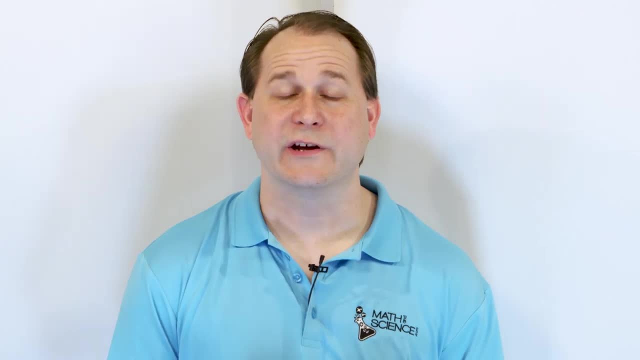 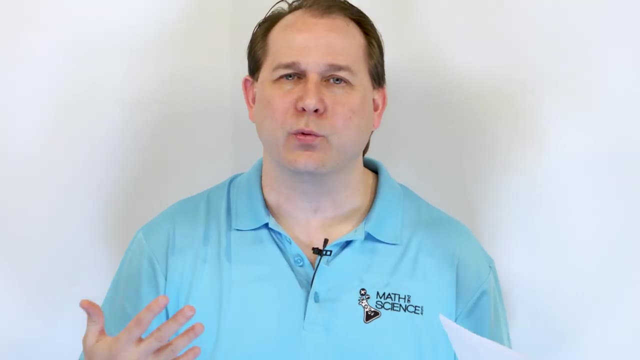 compound interest. All right, I hope you've enjoyed the computer demo and understand that the shape of the curve when you invest money at some sort of annual interest rate actually follows an exponential curve. Now why does it follow an exponential curve? That's what we want. 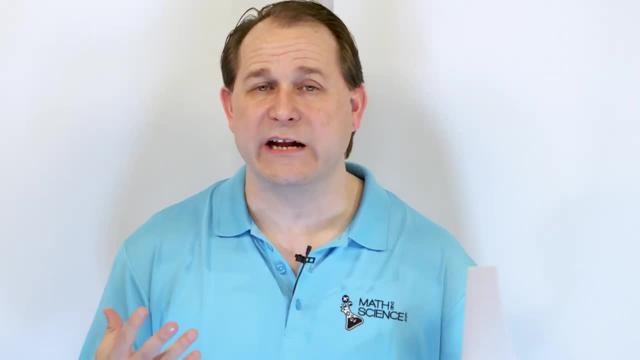 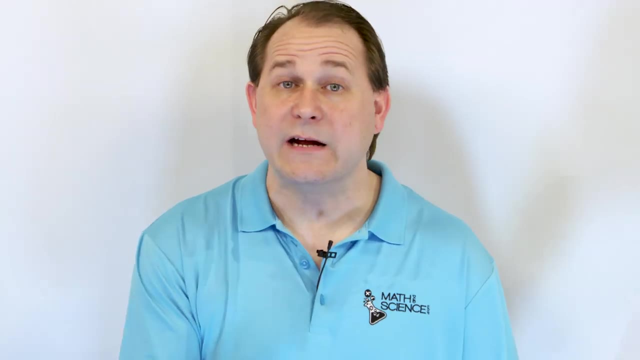 to talk about now. Why is it an exponential function? In words, in a nutshell, this is an exponential function. This is the reason why, Let's say, you start on day one with some money- $100.. On day number two, 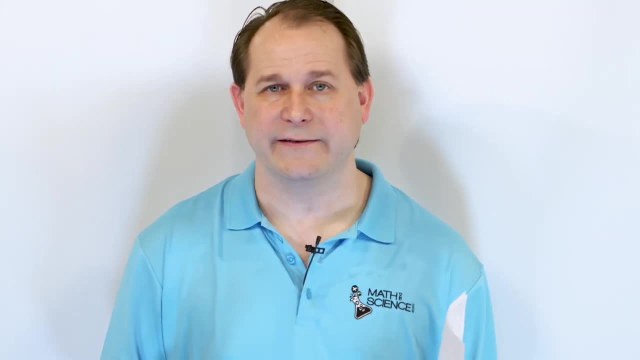 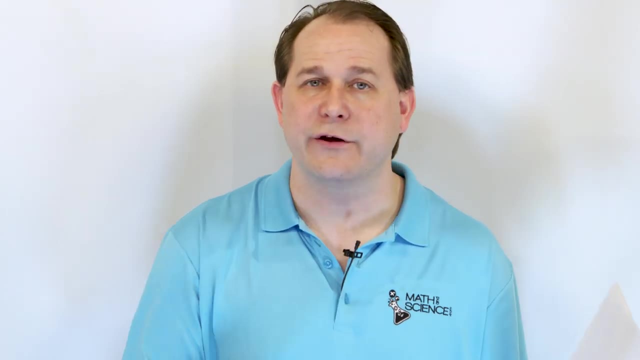 let's say you earn some interest, very small amount, let's say 8%. So now I have more money than I did on day one, because I earned a little bit of money. But on day three I again earn, let's say another 8%. But that 8% is calculated based on what I had on day two. So every time you compound, that's what it's called. when you calculate the amount of money you get, it's called compounding right? So when you calculate the new amount of money I have, it's always based on the previous amount that I had. So I started with some number, I gained a little bit, but when I calculate 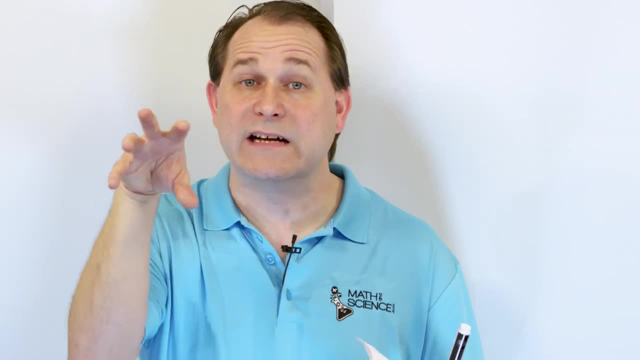 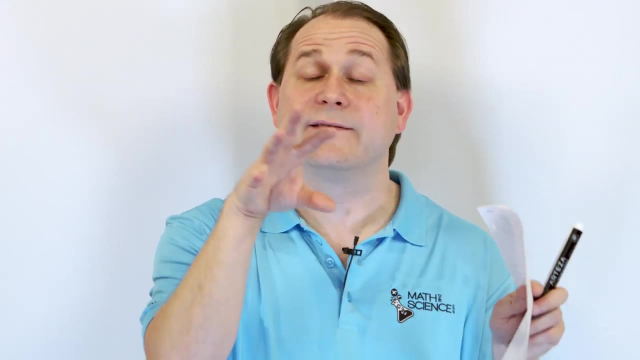 the next amount of money. it's a percentage of what I have on day number two, which is already more money than day one. So now I have even more money. But then the next time I calculate the interest, I calculate it based on the latest balance, which is even more money. So you see. 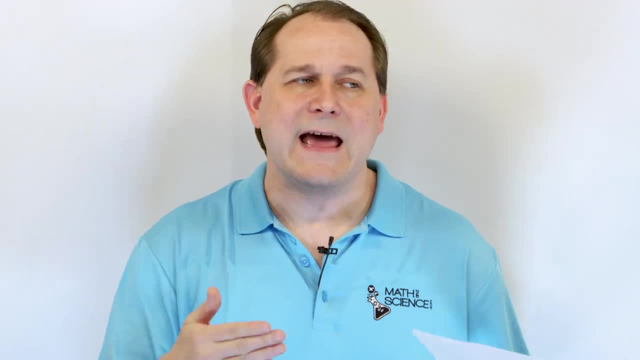 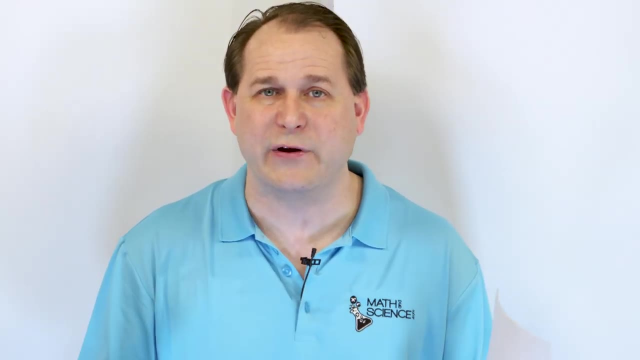 what's happening is every day I'm earning more money, or every year I'm earning more money and I'm calculating the free money I'm getting based on the amount of money I had the previous period, which also had free money. So 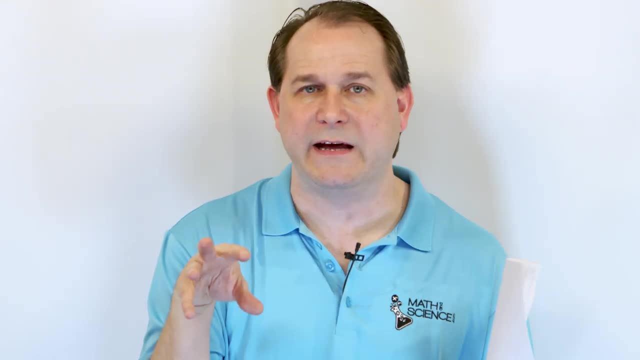 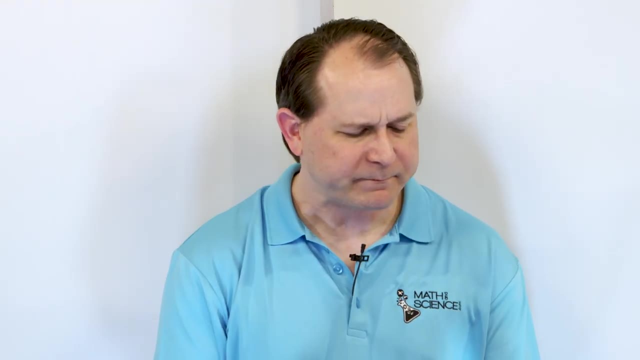 every day I'm gaining money and I'm calculating the amount of free money I'm getting based on the free money I had yesterday. So it snowballs and it kind of gets out of control and that's why it goes up like that. So we have to define some terms. The money that you start with is called 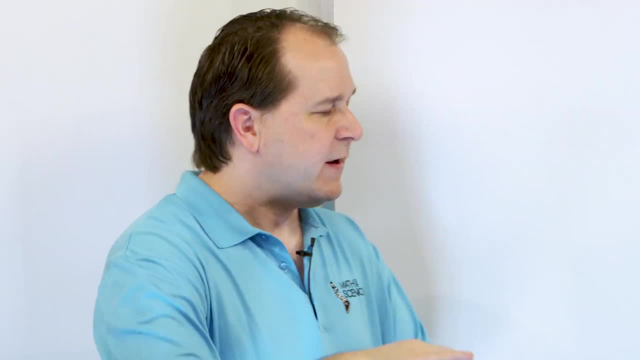 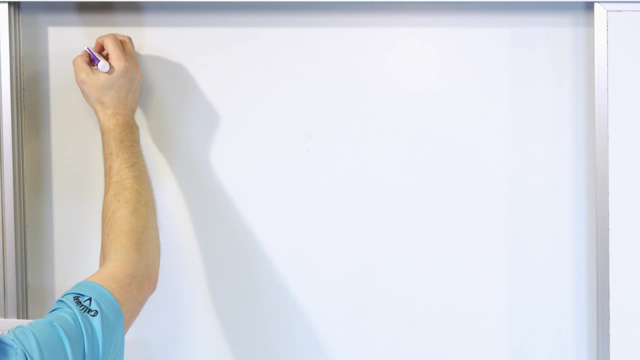 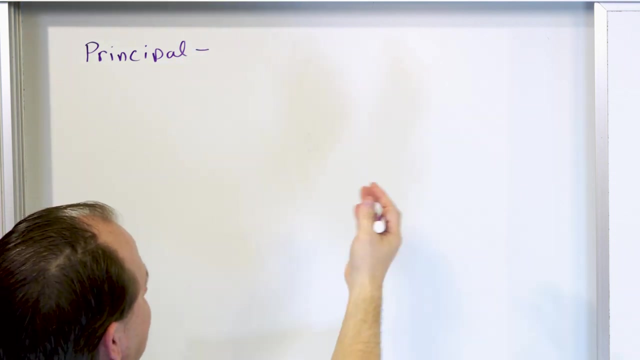 the principle: That's how much money I start on day number one. So I'm going to write a few terms down and we're going to talk and derive specifically why this thing is an exponential function. So the principle: that's just how much money I start with. Let's say I start 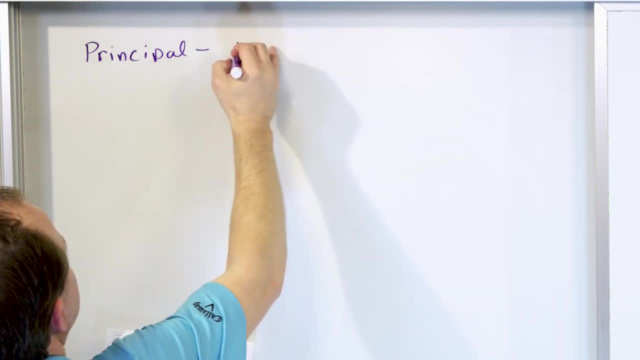 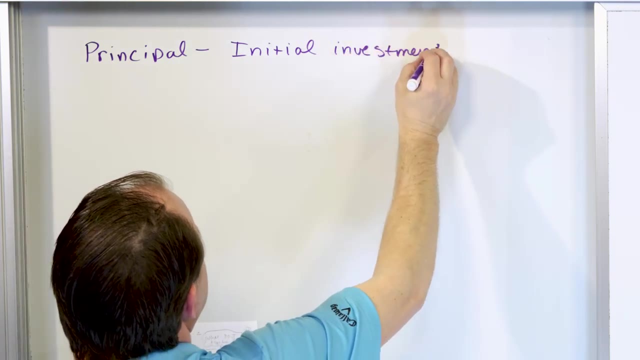 with $1,000, and I'm going to put it in the bank and I'm going to earn some interest on it. So this is the initial investment. It's just how much money I put in myself. Okay, And let's say: 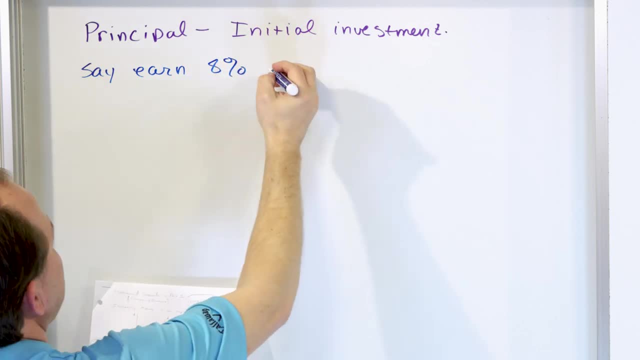 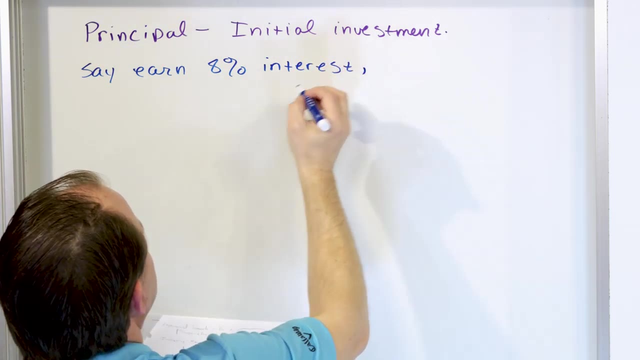 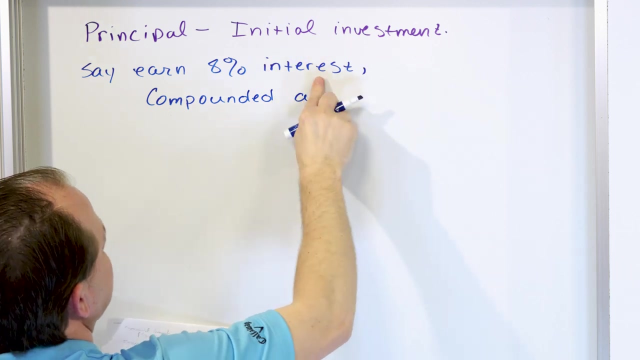 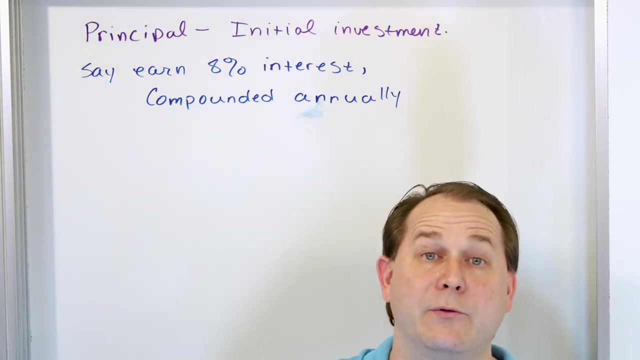 I have 8% interest. Now we have to talk about something else which is called, let's say, that it's compounded annually- Whoops, Annually. You're going to start to see something where it talks about compounding annually or compounding quarterly or other kinds of compounding. Don't. 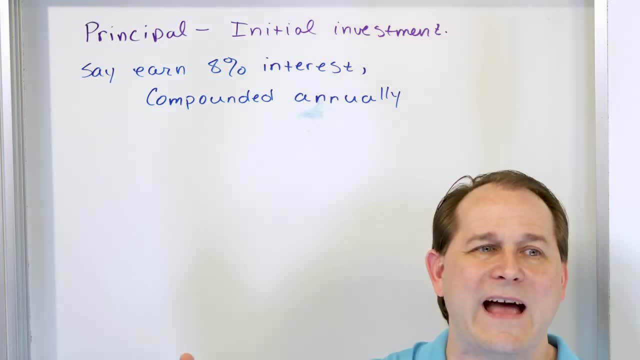 get so worried about it. Compounding annually is going to be compounded annually. Don't get so worried about it. Compounding annually just means that's when the free money comes in. It's every year. So every year I get 8%, And then the next year I get 8% of what I had from the previous. 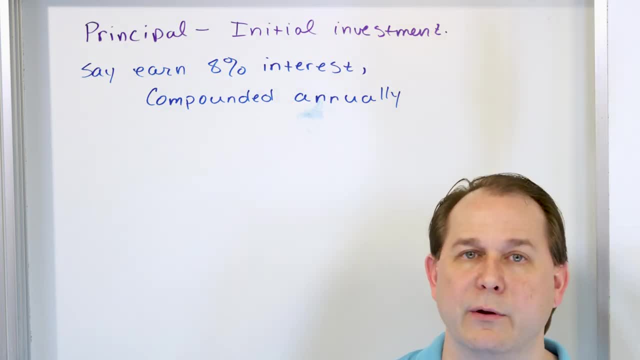 year And then the next year, I get 8% of what I then have on my most latest balance. So I'm growing every year but I'm gaining 8% on the latest balance in my account. So the compounded 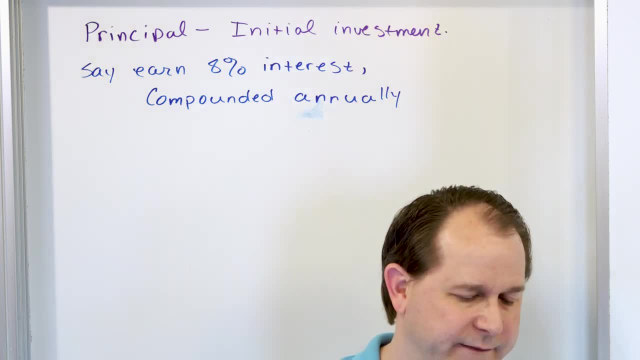 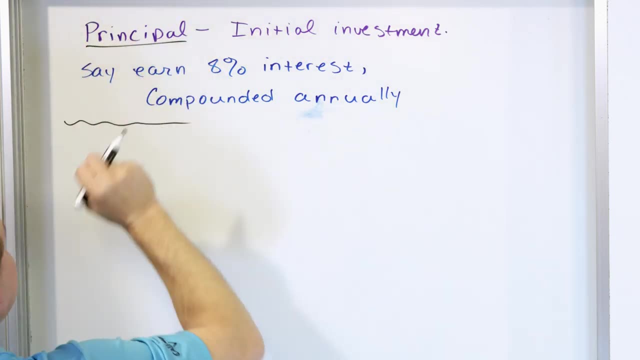 annually means that's happening every year, one time per year. That's all that that means. Okay, So how would we calculate how much money I actually have in the bank if I invest some amount called the principal initial investment? But let's just pretend, just for this example, that it 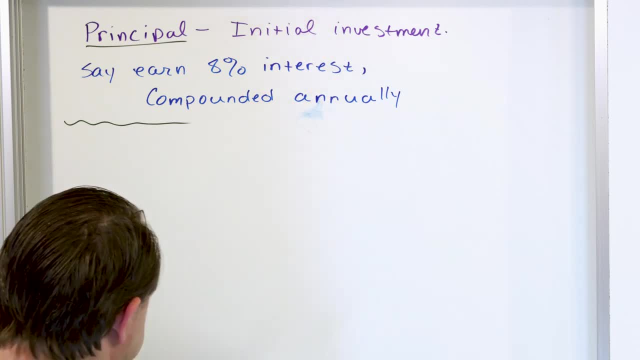 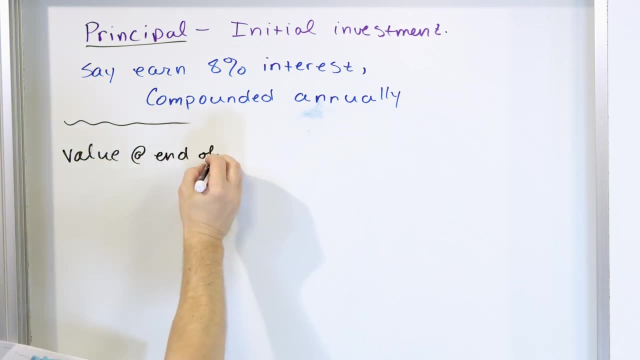 earns 8% compounded every single year, which means annually. Okay, So what we have then is the value at end of the year is going to equal the following thing. It's going to be- Let me write it all down then I'll explain it to you. It's going to be 1 times the value at beginning. 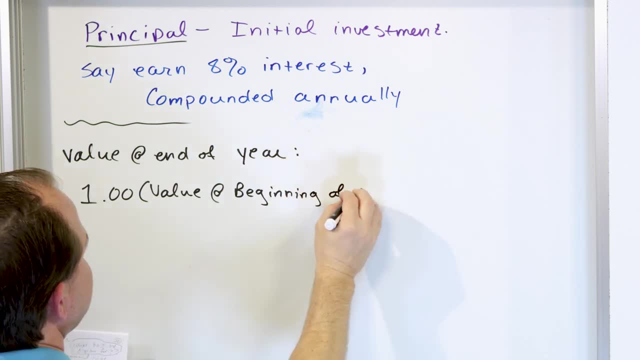 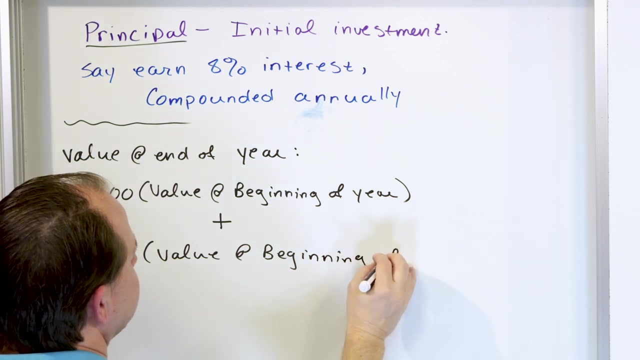 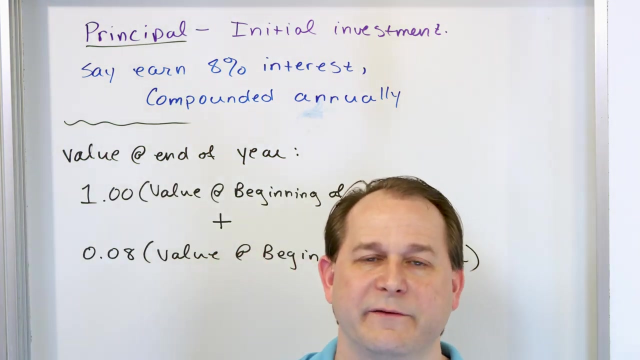 of year, Okay, Plus it's going to be 0.08 of the value at the beginning of year, All right. So basically, what happens is every year I earn 8%, But I still have the initial investment I put in. I still have the principal. So what happens is the money I have. 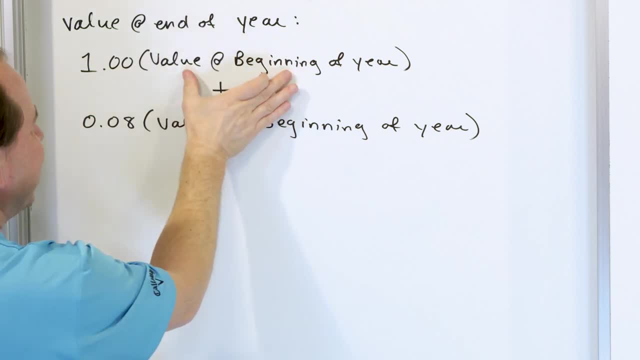 at the end of year. number one is 1 times the principal. The value at the beginning of the year is just my principal. It's 1 times that. That's just the principal value, But I'm going to add to that 8%. Now when you deal with. 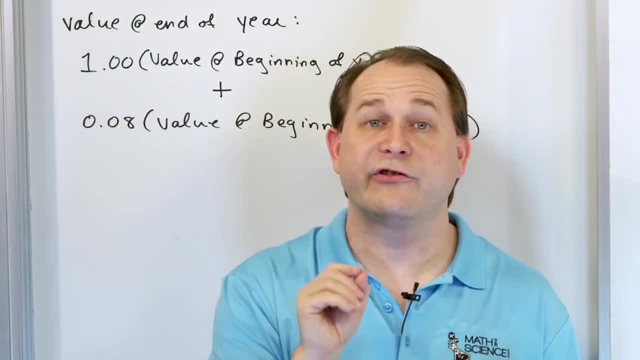 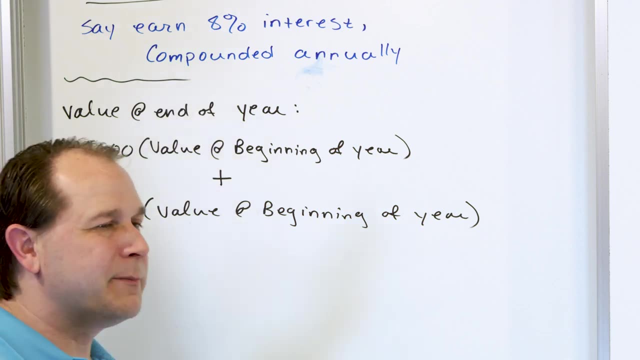 percentages. in math you never, ever write a percent symbol, You just convert the percent to a decimal. So 8% as a decimal just means you move the decimal point two spots Because, remember, percent means per 100.. So you're dividing by 100.. So this 8% means it's 0.08.. So you're adding to. 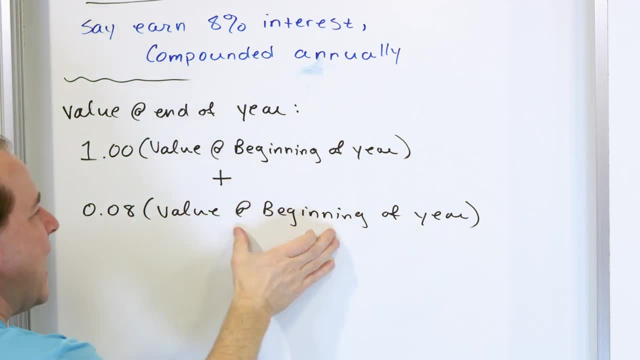 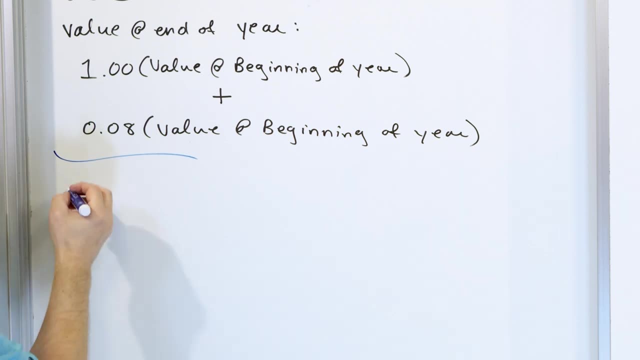 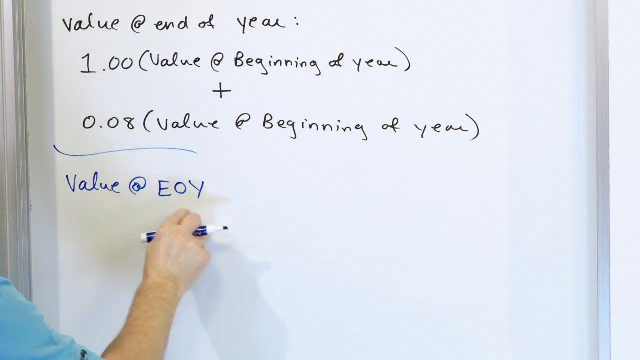 it. This is the free money, 0.08 times the principal, which is the value at the beginning of the year. Okay, So if I want to kind of write this a little bit neatly, then I would say value at. I'm going to call this end of year. This is E-O-Y end of year is going to then. 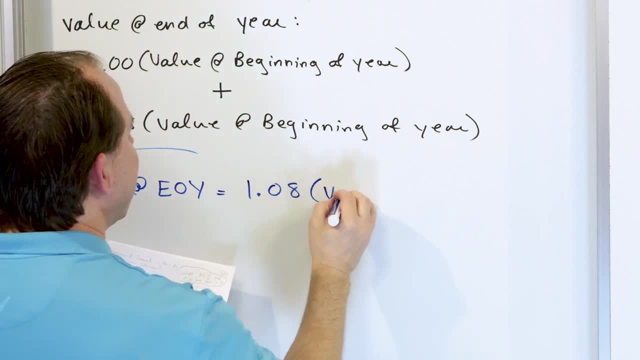 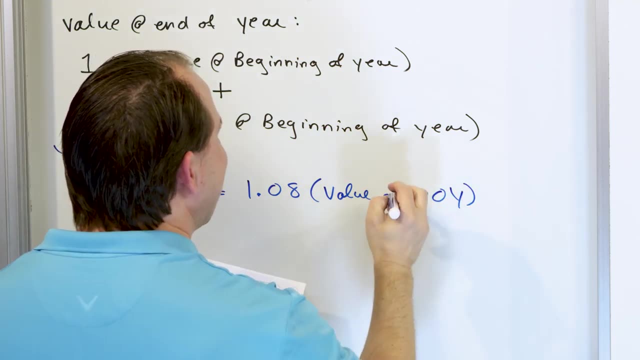 be equal to 1.08 times value at the beginning of the year. If I can write the word, the word at Okay: Beginning of year, end of year. So what's happening here? The value at the end of 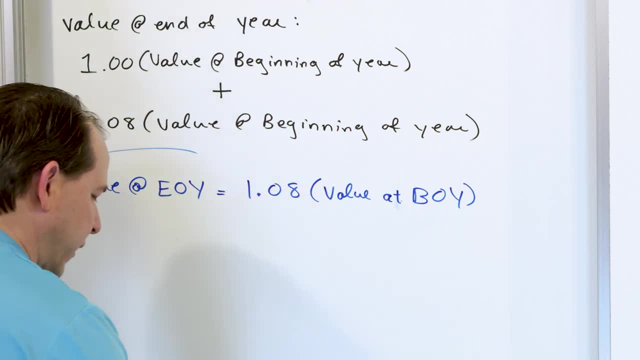 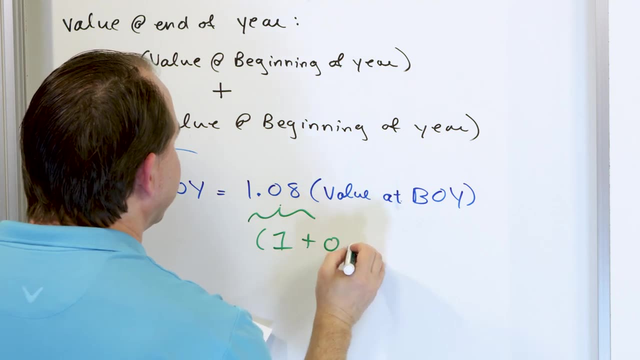 year one is 1.08.. A lot of students wonder where the 1.08 comes from. All this means 1.08, remember- is just simply 1 plus 0.08.. That's what that means. So 1 plus 0.08.. So the reason we multiply: 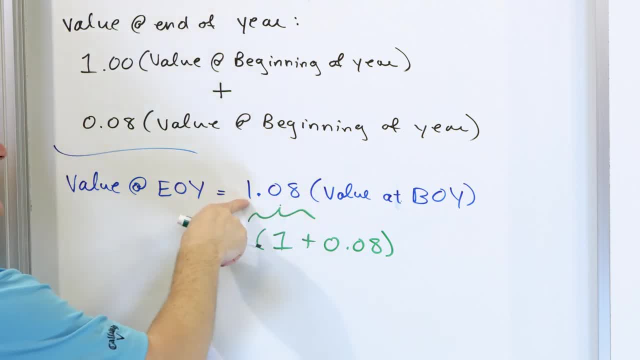 by 1.08 is because the 1 means the 1 times. this is this number. That means that's how much money I started with. The 0.08 is the free money. Again, that's times this. Now you can look at this as algebra and you can factor out the value. 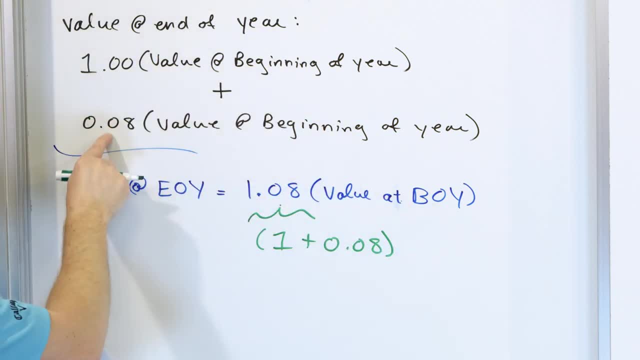 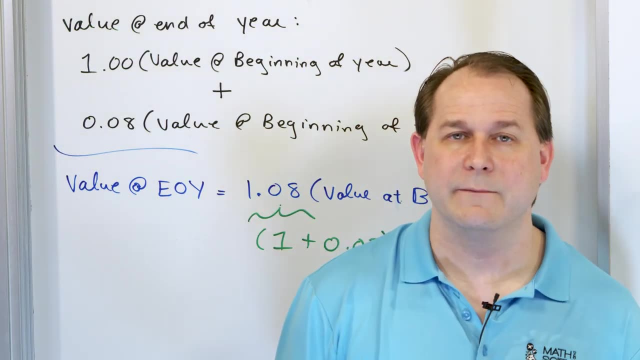 at the beginning of the year, pull it out and then you're going to basically be able to add these together and it's going to be 1.08.. So the actual free money is just 0.08 times my initial investment, but I can add to that what I started with. So ultimately the number you're multiplying. 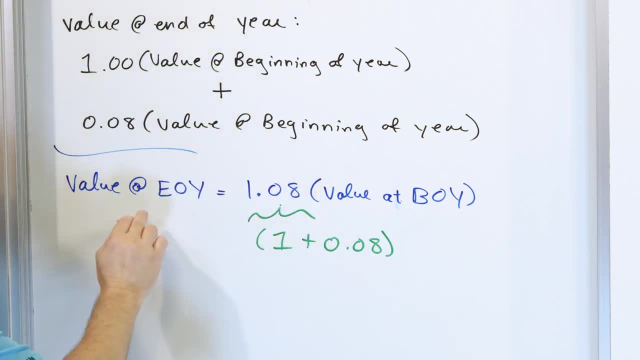 by is 1.08.. This is going to be the amount of money I have at the very beginning of year number two. All right, So a chart is Worth a thousand words, All right. So I think it's very, very important that we write a chart. 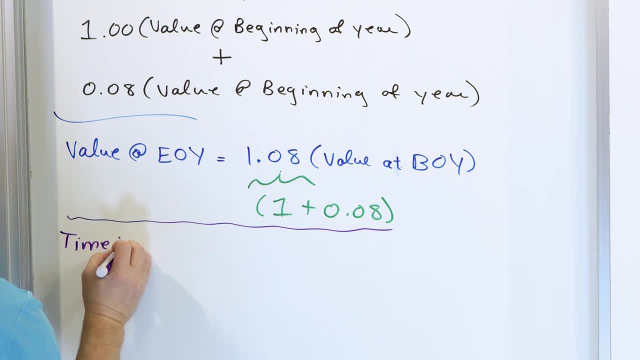 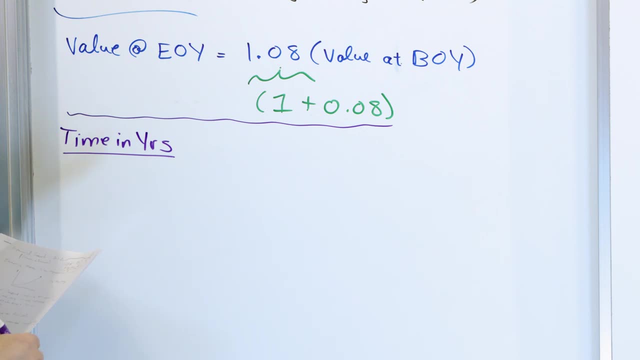 So here is the time in years. This is compounded annually. So this calculation of getting the free money, it's only happening every single year, right? So let's say that I'm at the beginning of the year, I'm sorry at the year zero, right? And then I have year number one, year number two. 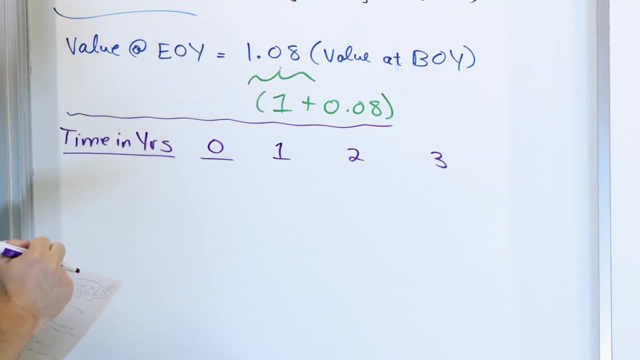 year number three, and I'll go on after that In just a second and show you what that is. But basically, this is year number one, year number two, year number three. What is this calculation going to look like? Okay, So this is going to be. 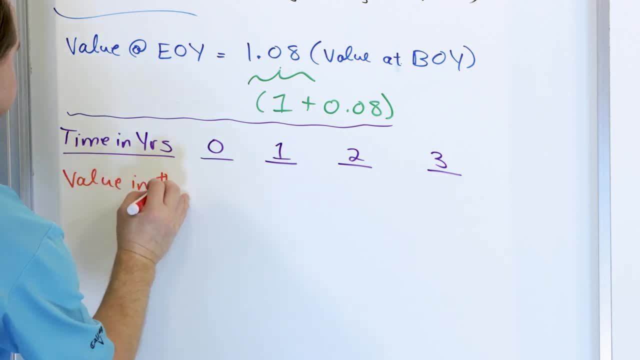 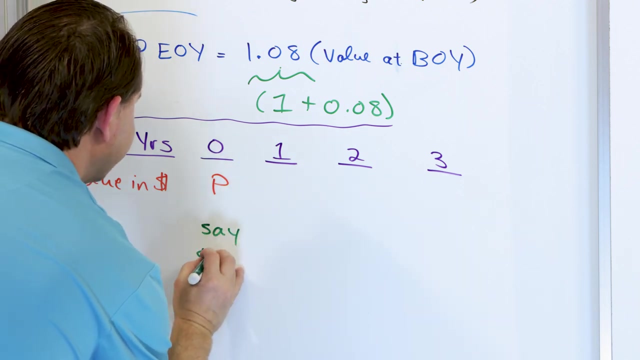 the value in dollars. All right, So what's the value in year zero? at the beginning, so to speak? It's just going to be. whatever the principle is, whatever that number is, Let's pretend that we've invested a thousand dollars. Okay, So let's say that this number is actually $1,000.. That's what. 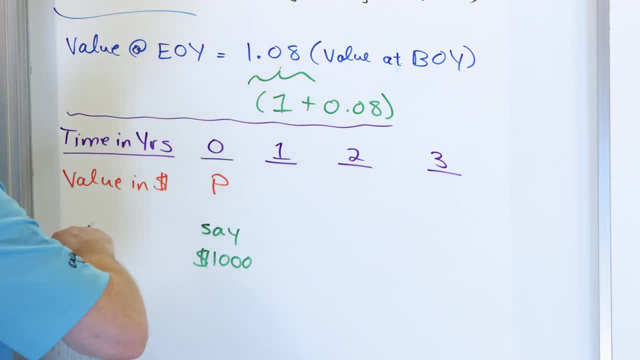 is going to happen at the kind of the beginning of the next year, after one year has passed. Well, what's going to happen is I'm going to take this principle and I'm going to multiply it by 1.08.. The one means: 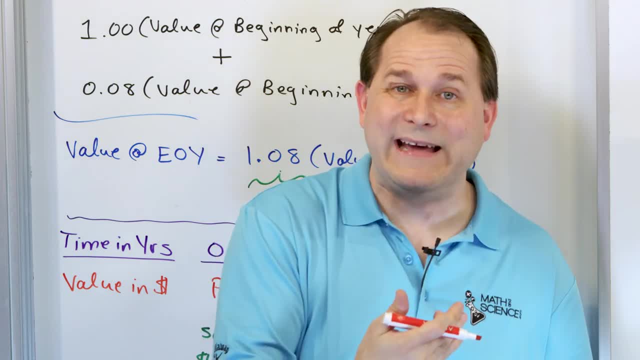 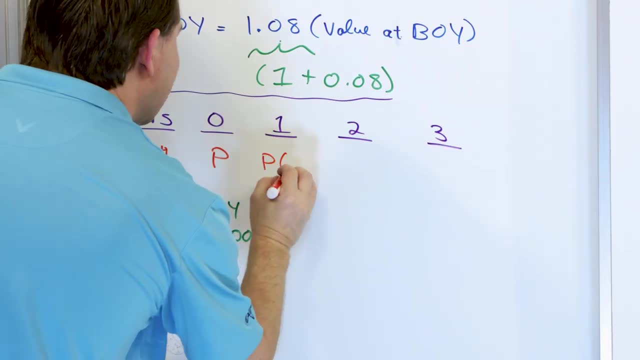 that I'm kind of carrying over what I started with. but the .08 is the free money I'm getting there. So ultimately I multiply by 1.08.. So what do I have here? I have the principle times 1.08.. That's how much money I'm going to earn. So if I started with $1,000 and I multiply by, 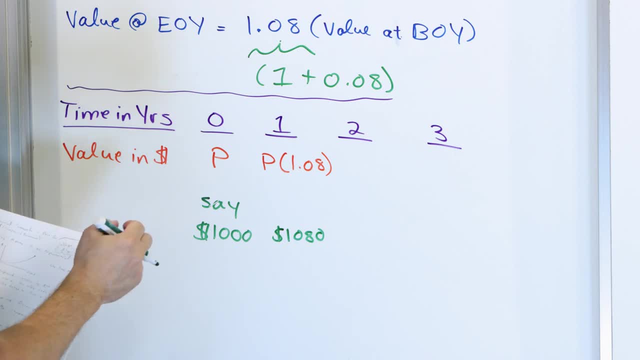 a number: 1,080.. So at the end of year, at the beginning of the next year, once the first year has happened, I no longer have $1,000 in the bank. I have $1,080 in the bank. The 1,000 is the money. 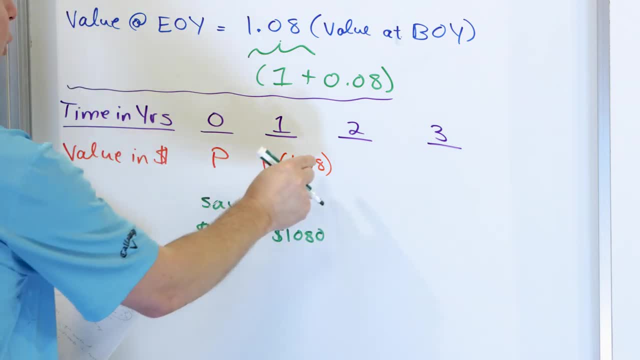 I started with and the $80 is the free money, right? .08 times 1,000 is 80.. So the free money is the 80 and I add them together and I get $1,080.. Okay, What is going to happen at the? 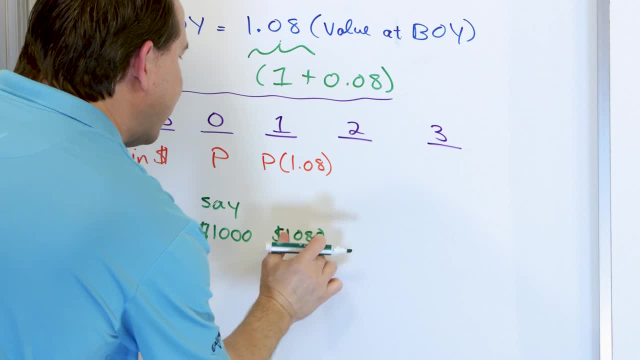 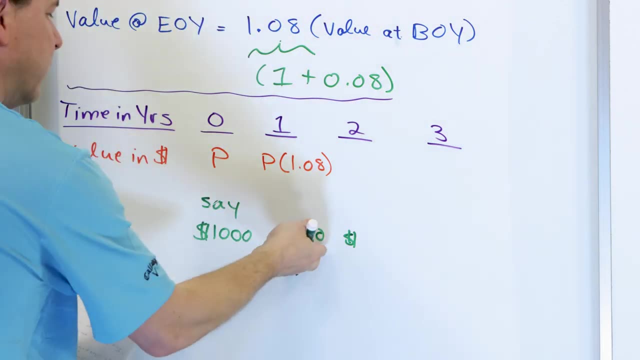 beginning of the next year. Well, I'm going to take this balance- the $1,080, and I'm going to again by 1.08, because the next year I earn again 8% interest and I can still keep what I had. 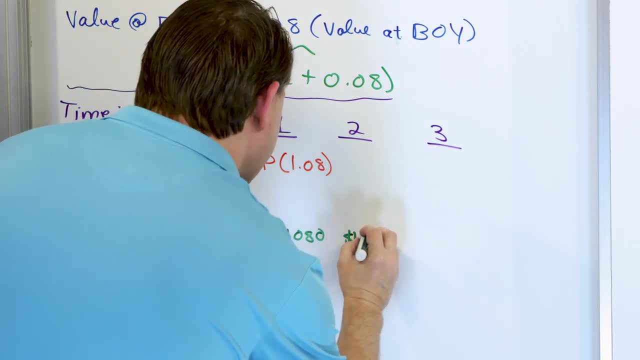 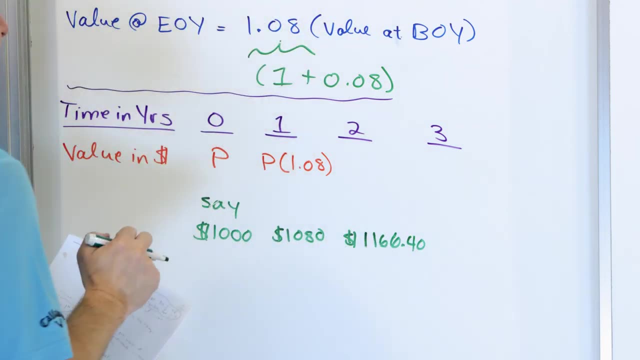 started with there to begin with. So that's going to come out to 1,166.40.. So 1,166.40 on $1,000.. Now, in terms of math, what's going to happen is you're going to take that principle. 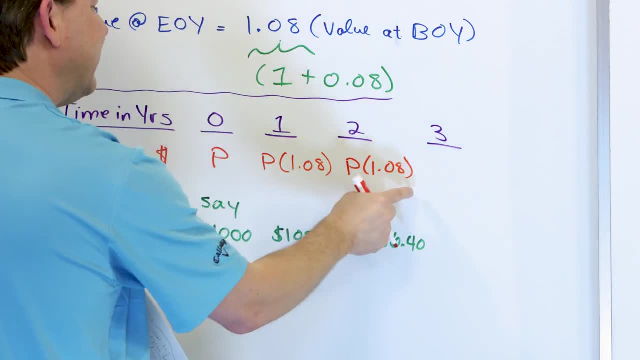 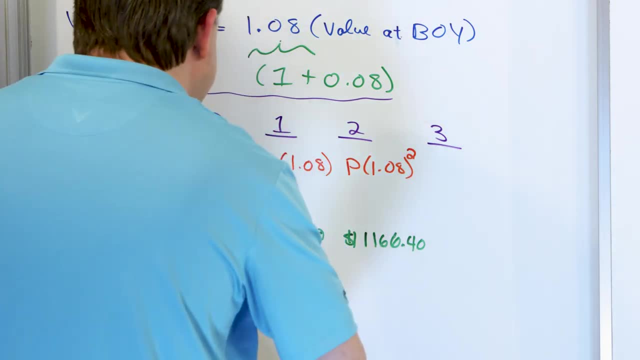 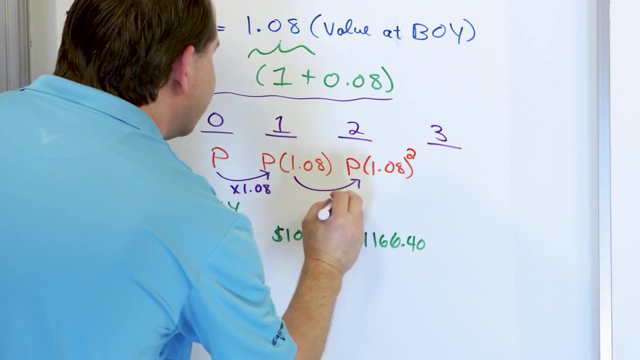 squared. okay, Because what's happening is: between this step and this step, I multiply by 1.08.. But between this step and this step, I again multiply by 1.08.. So this is times 1.08, and that's why it's. 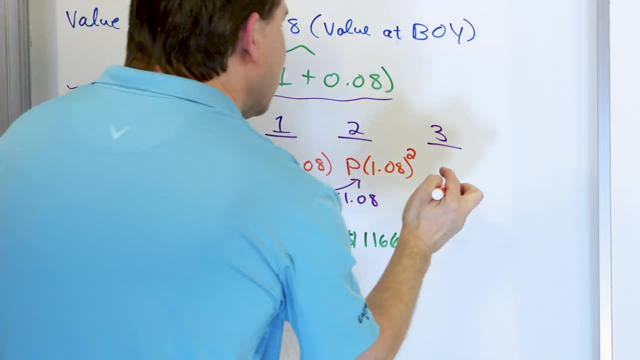 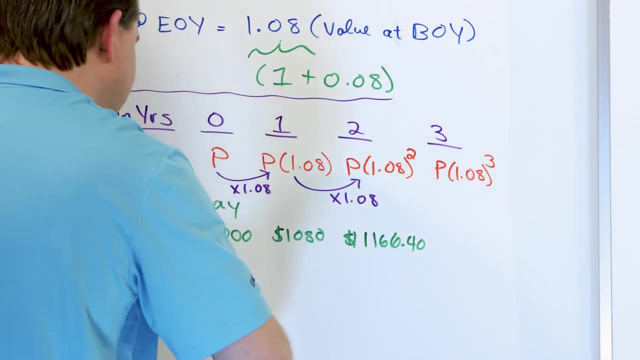 squared right here. So what do you think is going to happen over here? Well, I'm going to have, for year number three, I'm going to have 1.08.. It's going to be cubed. Why is it going to be cubed? 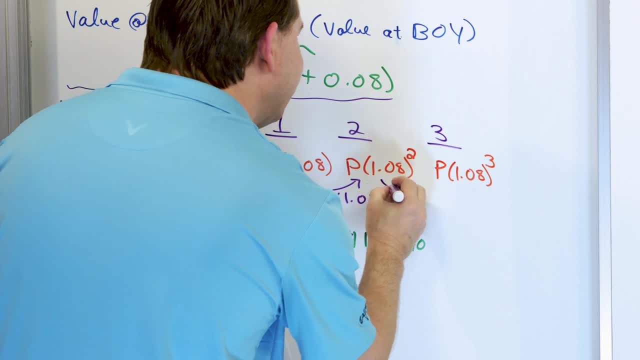 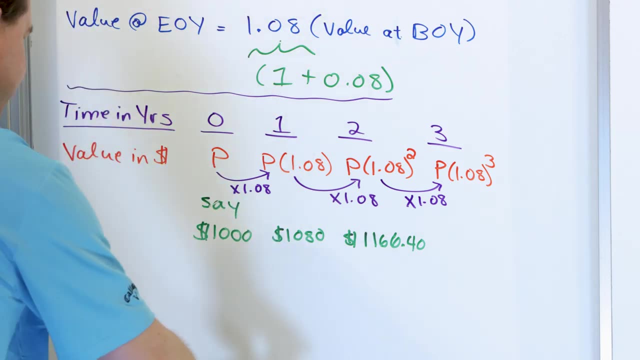 Because what I do is I take the money I had in year number two and again I multiply by 1.08.. So every year you're multiplying by 1.08.. And if you're going to do this kind of pretend on $1,000,. 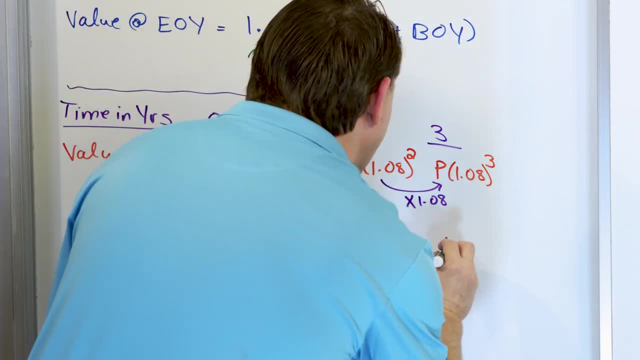 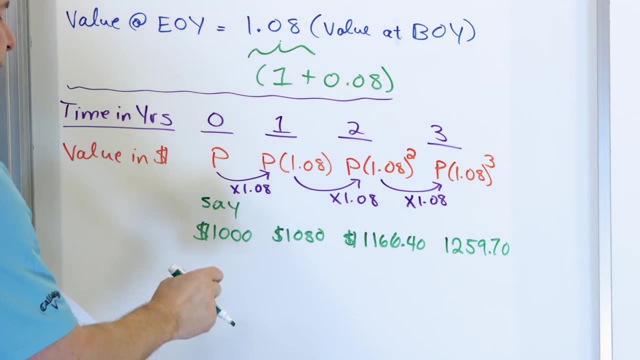 I would take this number and multiply by 1.08, and I would have 1,, 2,, 5,, 9.70.. I could be rounding here, So the exact number may be not quite right, but you see I started with 1,000.. Then I went to. 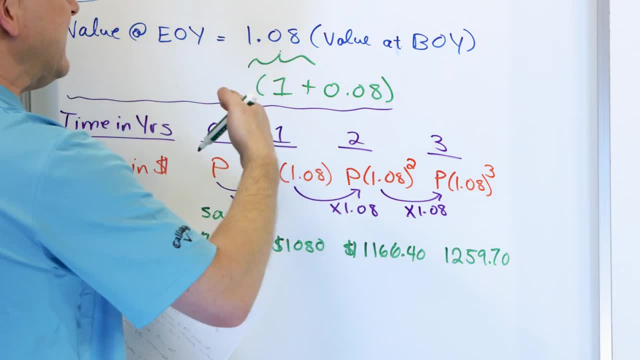 1,080. Then I went to 1,166. Then I went to 1,259. And so I continue this process every year. On the end of the first year I multiply by 1.08.. I get some number. Then the next year. 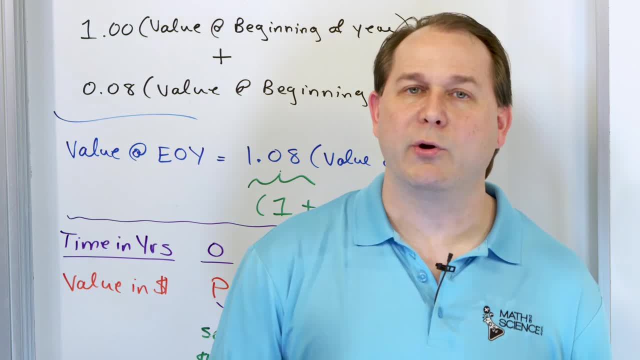 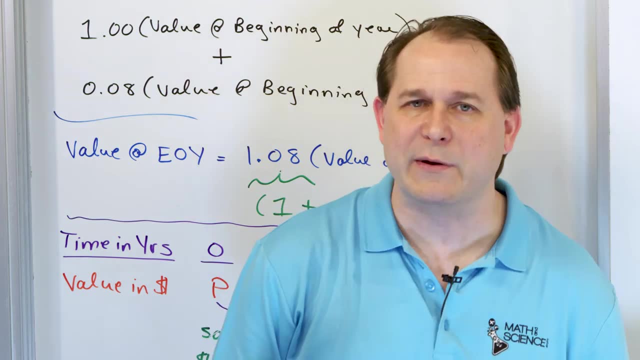 I multiply by 1.08.. I get some number. Then the next year I multiply by 1.08.. I get some number, Just like we were multiplying by twos over and, over and over again for that ridiculous example where I was giving you so much free money. it's crazy. Before this is a much more realistic. 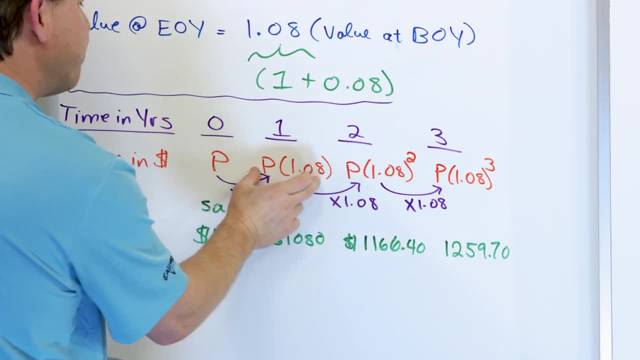 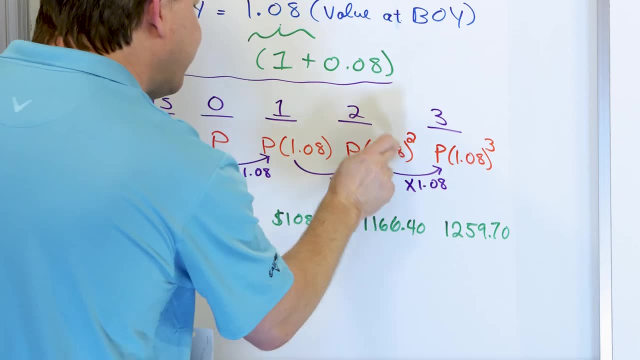 thing. But notice what's happening: It's P times 1.08.. But in year number two, because you multiply by 1.08 again, it's really P times 1.08 squared, because it's multiplied two times. In the next year it's P times 1.08 cubed: One, two, three, because I'm multiplying it again three. 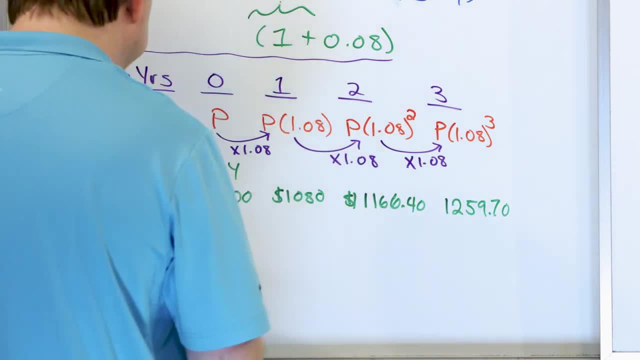 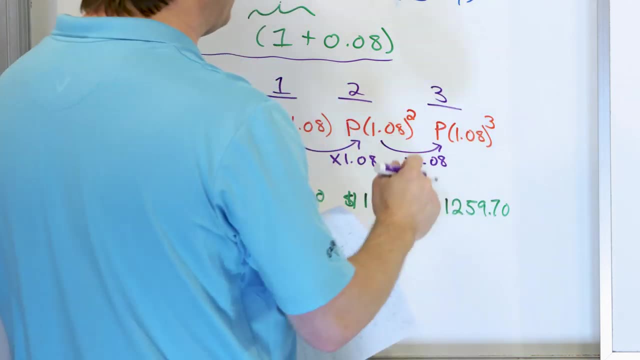 times, because I'm taking the previous number and multiplying it again there. So what is going to happen? if I extend to year number four, Then it's going to be P times 1.08 to the fourth power, Year number five, P times 1.08 to the fifth power, and so on. So instead of going in there and 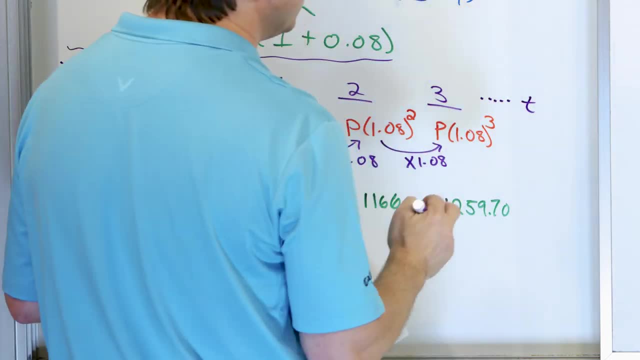 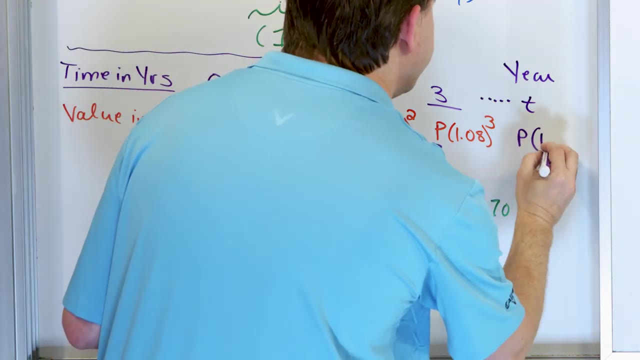 talking about year number four and year number five. let's go down the road to year number T. Let's generalize it to year number T. So then, this is going to be P times 1.08, cubed, It's going to be P times 1.08, not to the fourth, not to the fifth, not to the sixth. We're. 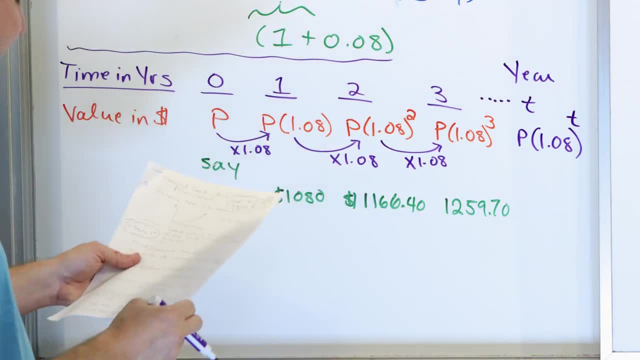 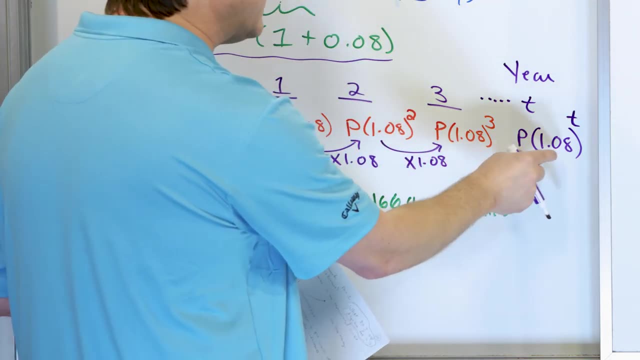 generalizing it. so it's going to be to the teeth power. That's what that means, because every year you're multiplying by 1.08.. So the exponent goes up and up and up and look at what this is: P times 1.08 to the power of T. That is an exponential function. Remember exponential. 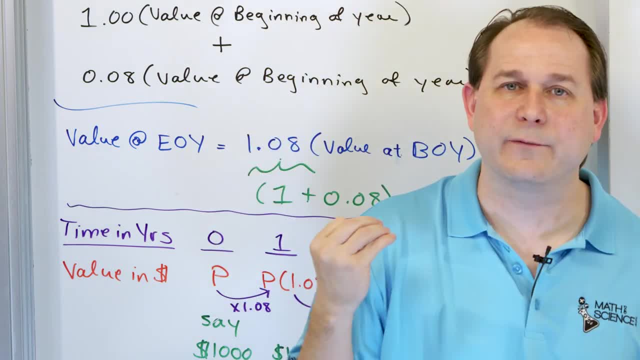 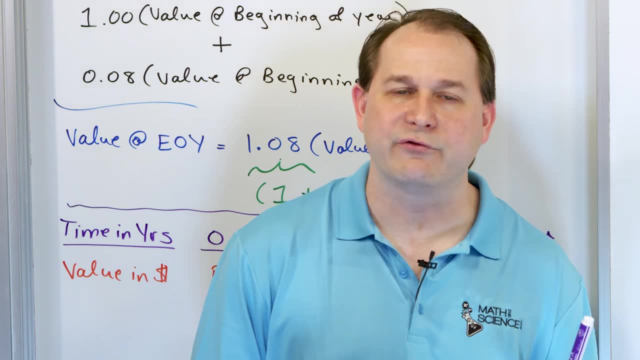 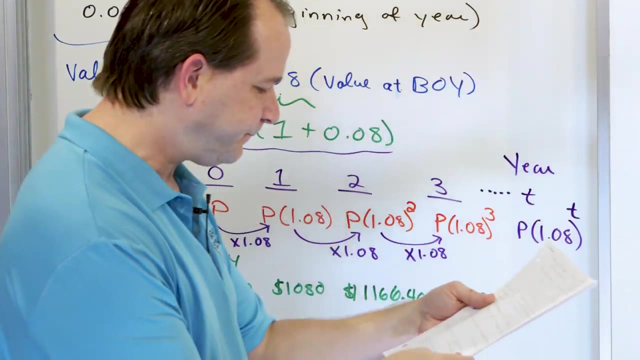 functions have the variable in the exponent. That's what it means. The time in years is a component here. That is why compound interest is an exponential function. That is why it grows so rapidly, like these exponential functions that we have been studying. Now one more definition. 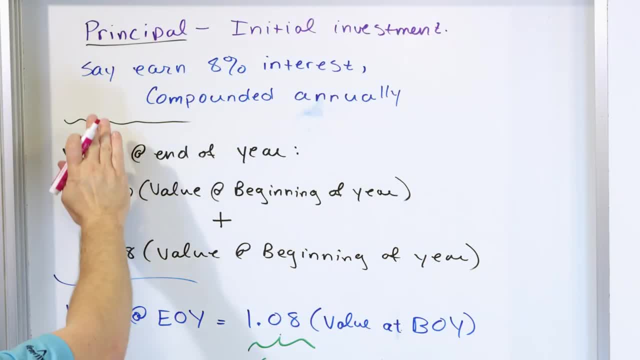 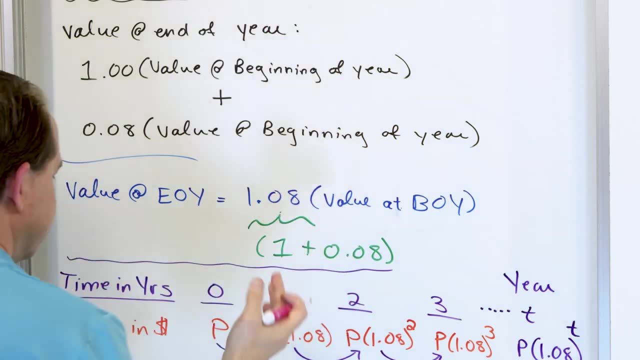 I want to give you before we go on to the next board is for this example, we were saying that we earned 8% interest compounded annually. So what this means, the actual term that you're going to see in your problems. this is called an annual interest. 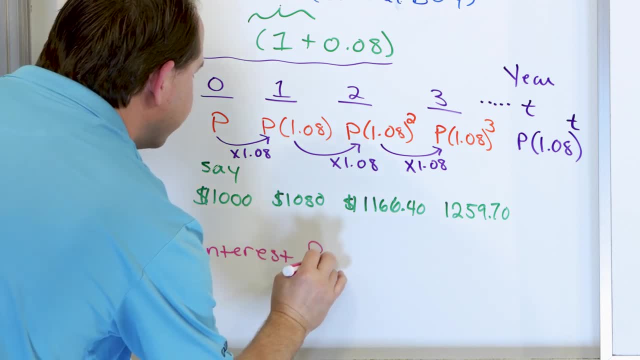 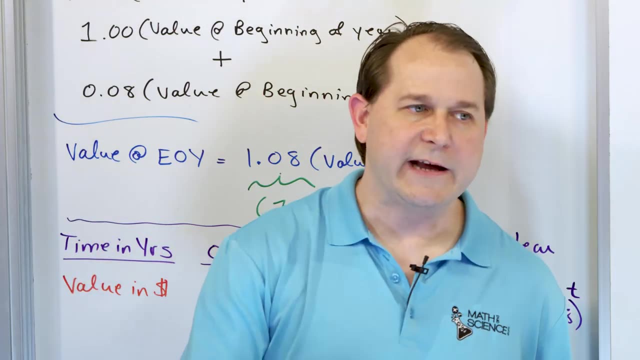 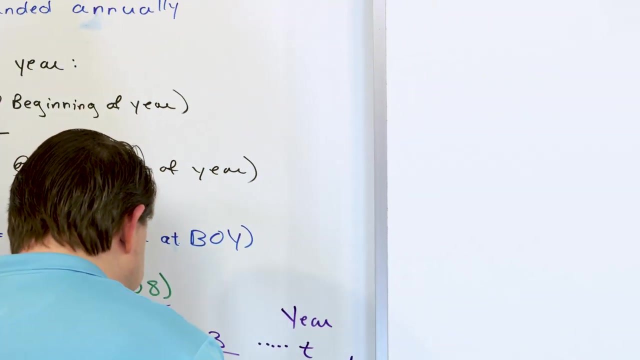 Rate. It's an interest rate because it's the percentage you multiply by, and it's annual because it means you do it every year. Every year I get another 8%, Every year I get another 8%, and so on. All right, So we want to talk about this in the most general form. So what this means is: 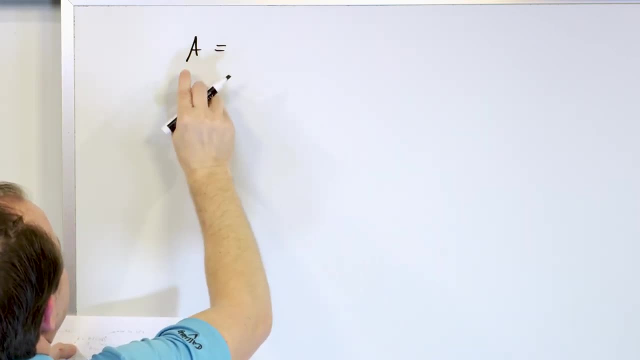 that if I'm compounding annually like this the amount of money I'm going to get- A- this is called the amount of money I'm going to have- It's going to be equal to the principal. However much money I put into this, it's going to be equal to the amount of money I'm going to get. 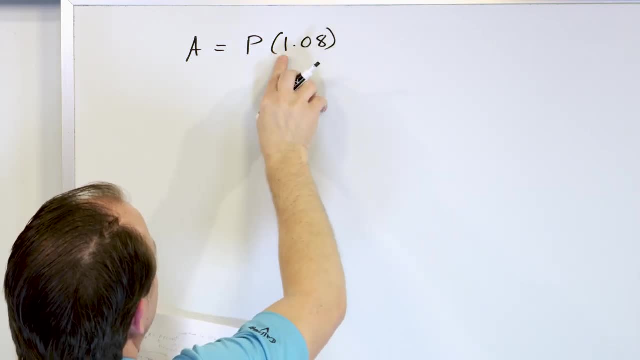 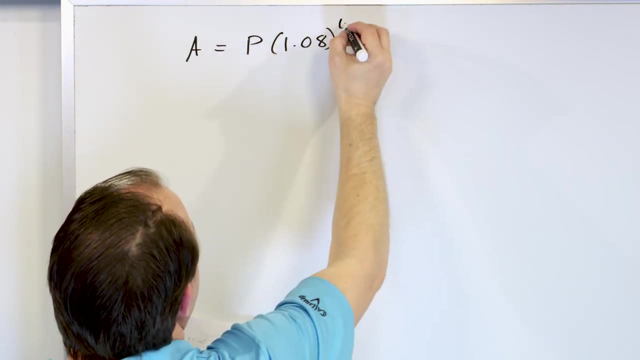 So I'm going to multiply this thing times in this example, 8%. The 1.08 means I'm multiplying by the full balance of what I had before, plus 8% free money to the power of t. So it's: 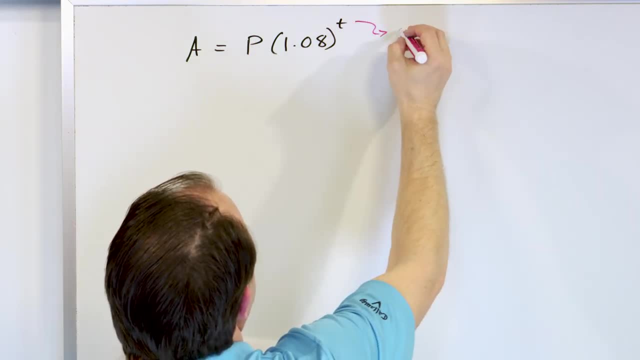 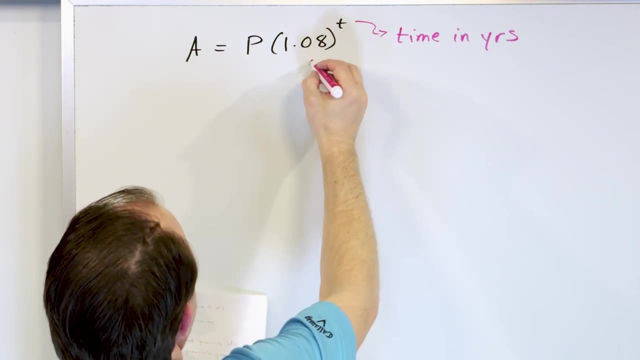 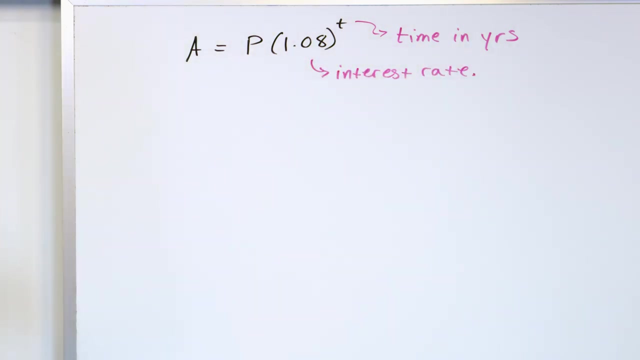 really important to study this. This t is time in years, Right? This is called the interest rate. Specifically, the .08 part of it is the interest rate. The P is called the principal And the A is called the amount. That's the amount of money I'm going to have total. 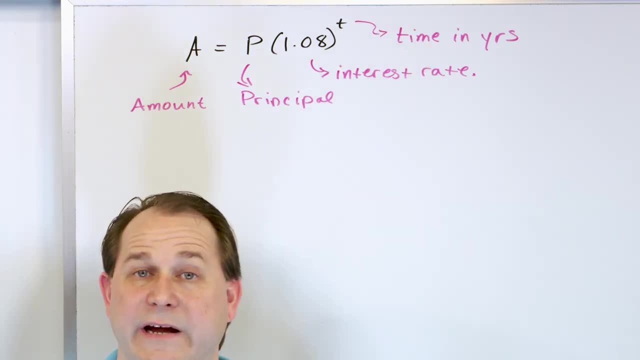 So I can do this as an annual compounding where I get 5% a year, 5% a year, 5% a year over and over and over, And this is going to be the equation that governs it. However, in real life, this is where it starts to get a little bit. 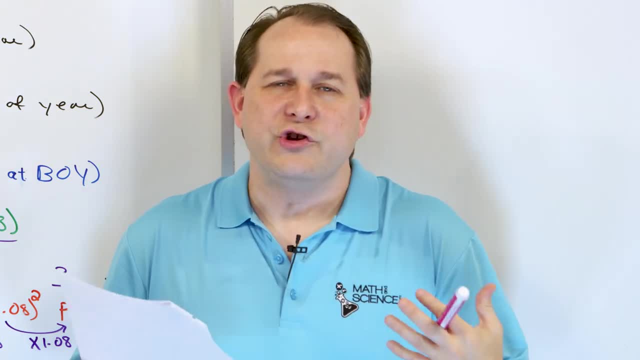 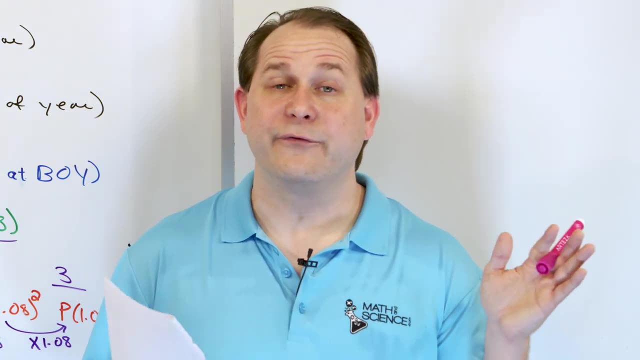 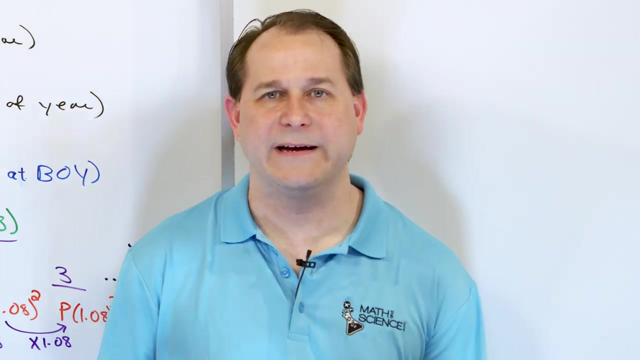 confusing, but I'm going to make it very easy to understand for you. Usually we don't compound interest every year. Usually interest is compounded quarterly, which means four times a year. There's four quarters in a year. You know four quarters in a year, Just like there's four quarters of a peanut butter and jelly sandwich when you cut it in four places. Right. 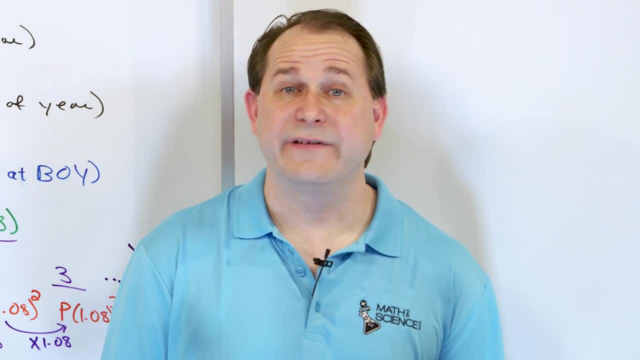 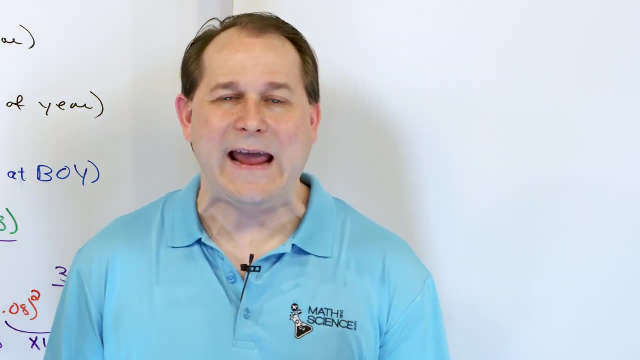 Sometimes you even have loans where the interest is compounded monthly or daily or something like that. So we need to talk about what does it mean when you compound something other than annually. So when you have annual compounding it means every year. That's when you do the calculation. 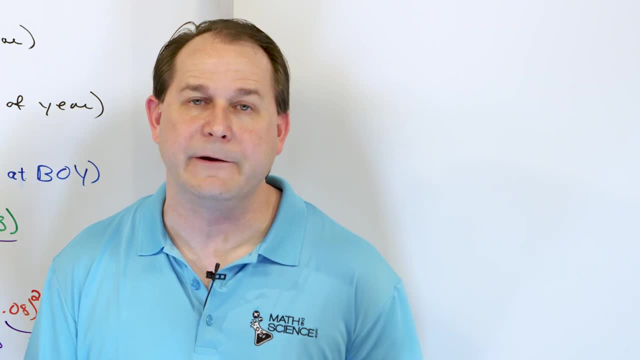 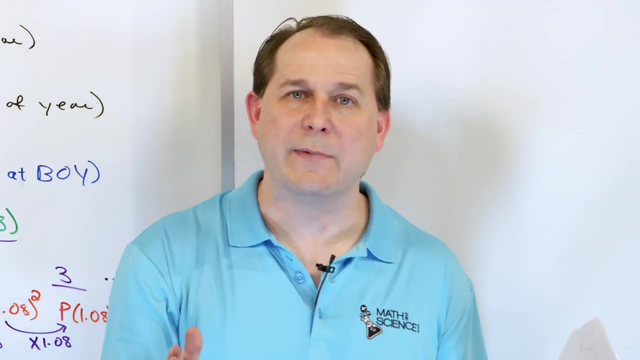 Year number one. year number two: That's the only time you get the free money Is every year, But when you compound quarterly, you get the free money every quarter. That means four times a year. So after three months that's a fourth of the year. 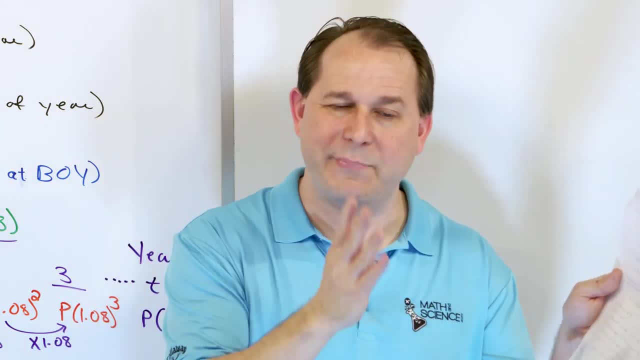 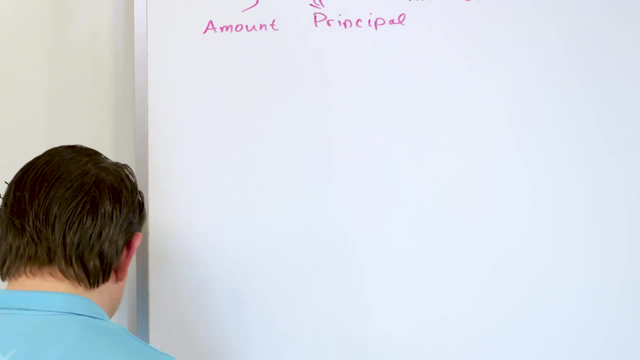 Bam, You calculate the free money, Then, after three more months, bam, You calculate the next amount of free money. Then, and so on and so forth. you do it four times a year. That's what it means. But what happens is when you compound quarterly. let's talk about this, Let's just write it down. 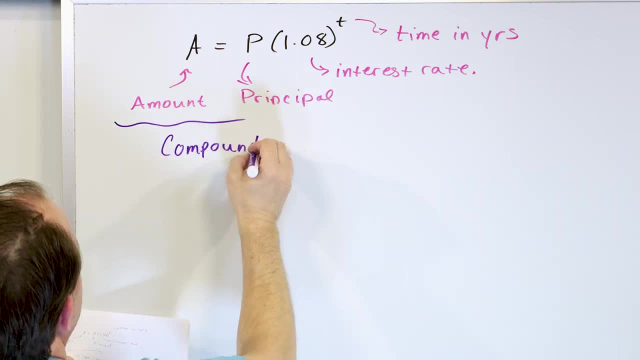 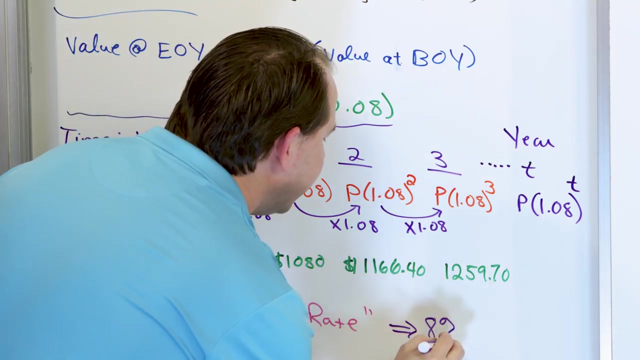 Compound quarterly. All right, What does it mean? What it means is: if I take that annual percentage- Remember, the annual interest rate in this example here was eight percent- That means I get eight percent a year The annual interest rate. But when I compound quarterly I'm not going to give you eight percent every quarter. 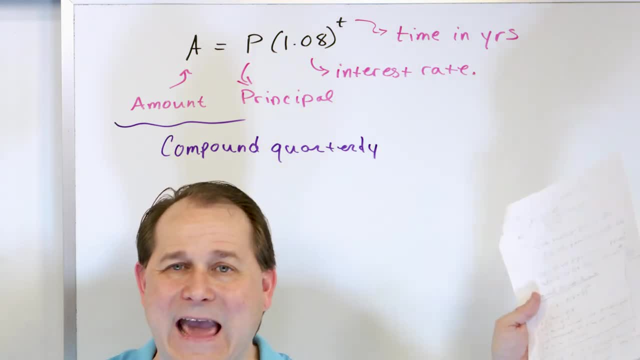 That's crazy. That's too much free money. What happens is you take the eight percent over the year And since I'm doing it four times a year, I just divide that eight percent by four. That's the amount of interest I'm going to give you every quarter. 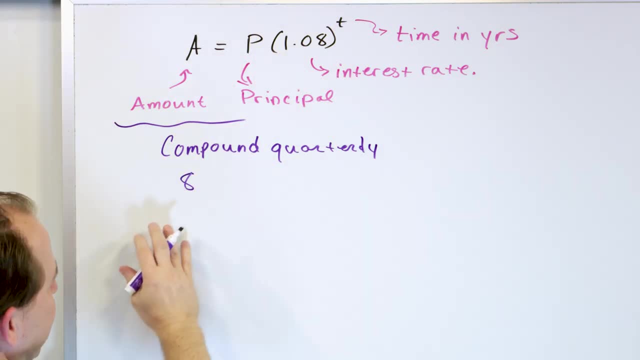 So what happens is I take the eight percent that I'm doing on an annual basis, But instead of doing it every year, I'm going to do it every quarter. That means I'm going to take this thing and divide it up into four pieces. 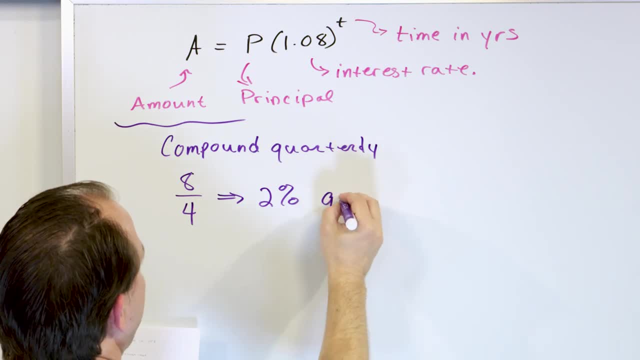 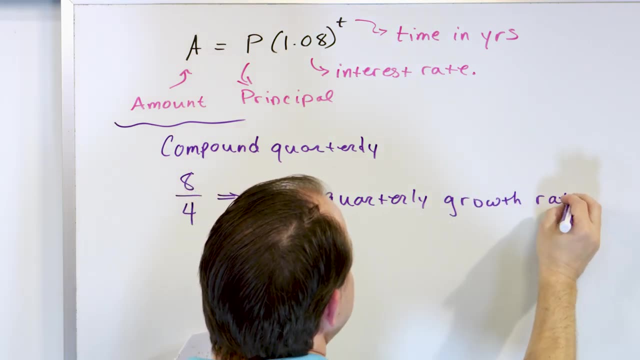 And I'm going to give you two percent interest as a quarterly growth rate. And again, this is where a lot of students get confused. because it is confusing, What happens is if I give you eight percent a year, this is easy to understand. 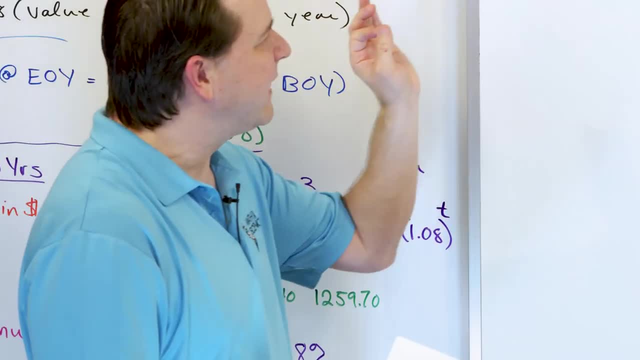 Every year. eight percent. a year: Eight percent, eight percent, eight percent. But if I compound it quarterly I'm not going to give you eight percent because that's an annual rate. So I take the eight percent, I cut it into four pieces. 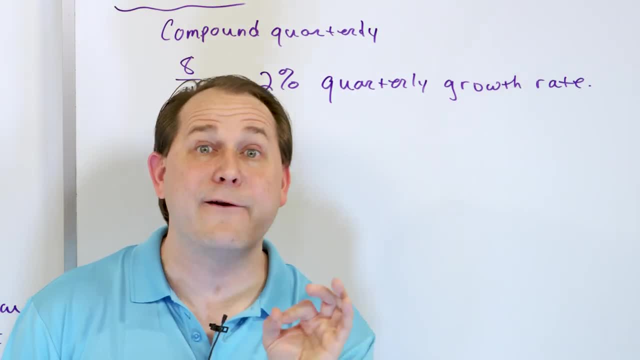 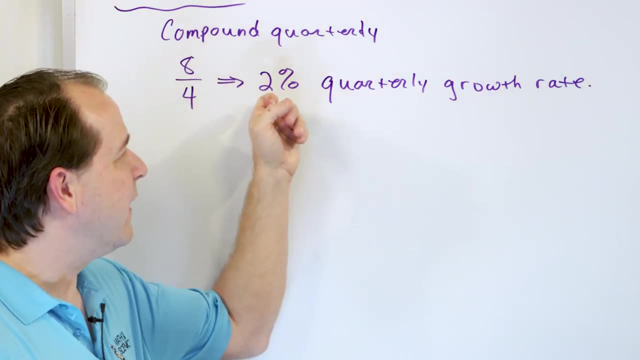 That means it's two percent. I'm going to give you two percent every quarter. That will add up to eight percent over the year. But I'm going to do the calculation on the free money every quarter. So I'm going to give you two percent every quarter, four times a year. 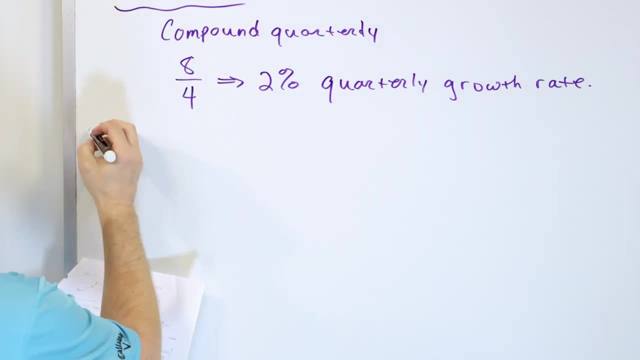 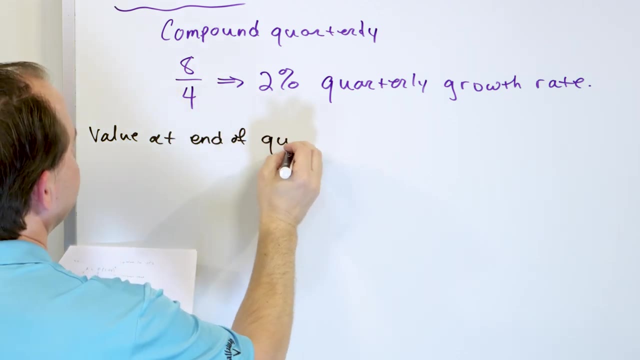 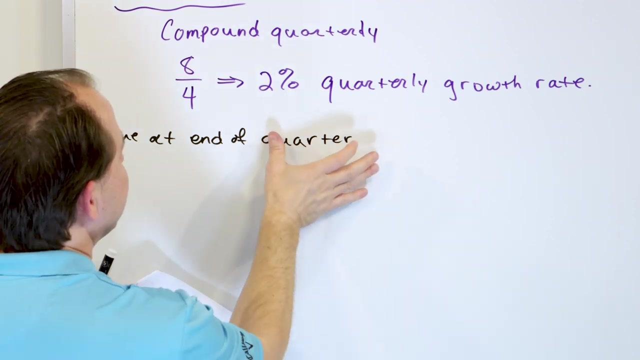 OK, so then what you would have is that you would have the value At End Of The quarter. Remember, I'm doing the calculation now, every quarter. Well, actually, the way I want to do it- at the end of Q. 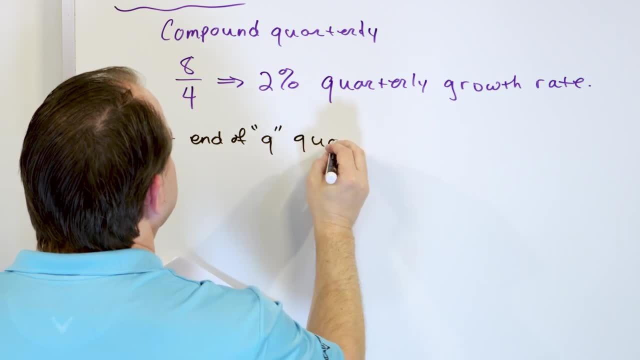 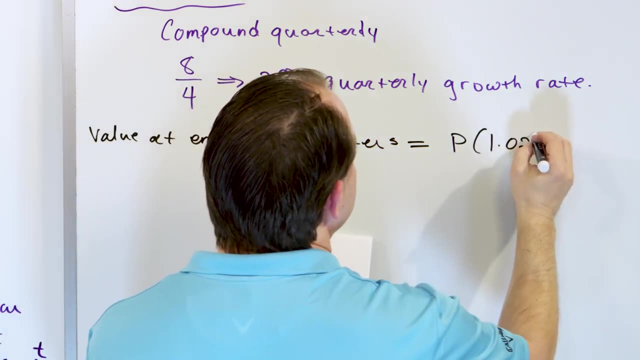 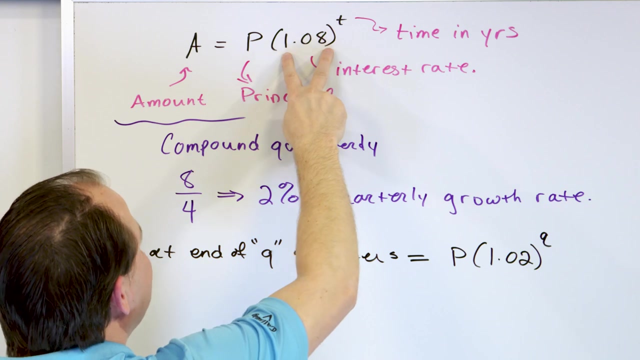 At the end of Q quarters Is going to be equal to P times one point, oh two, To the power of Q. Make sure you understand that it's exactly the same formula as this. This was the principal times: the interest rate raised to the power. 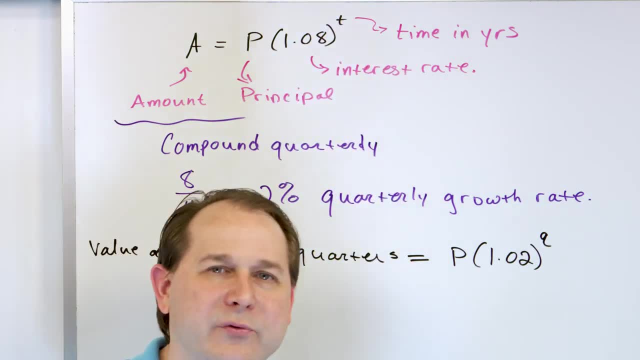 Of T in years, But now I'm not compounding yearly, I'm compounding a lot more often Quarterly. There's four quarters in a year, But still after Q quarters I'm going to multiply this balance by one point, oh two. 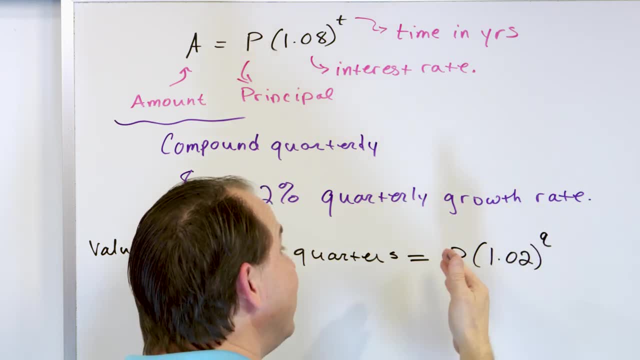 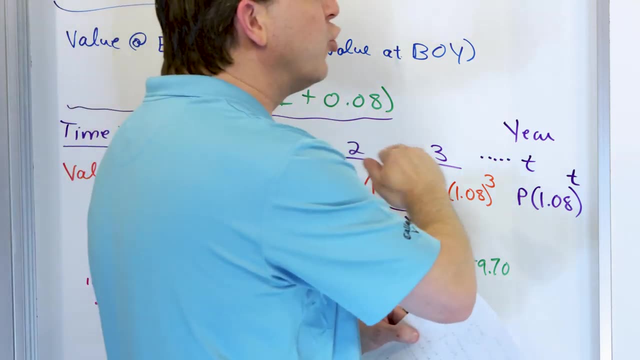 Then times itself one point, oh two. Then times itself one point, oh two. But I'm going to do it every quarter, Every three months. I'm going to do this thing. So it's going to be the exact same table, Except the numbers up here are going to be in quarters and not in years. 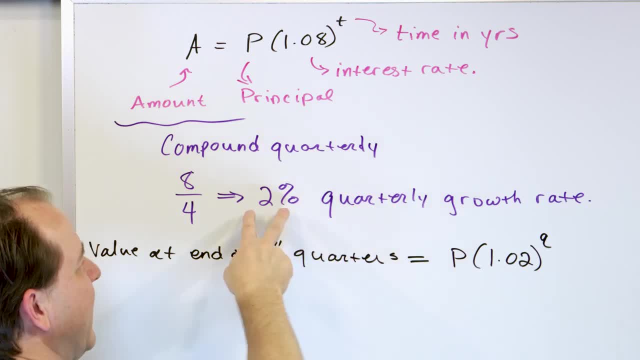 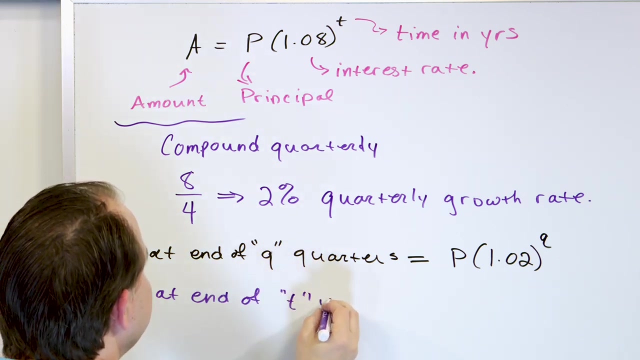 And the interest rate has to be smaller because I'm doing it more often And if you take the annual and divide by four to get that number, Okay. So then you can say the value At the end Of T Years. 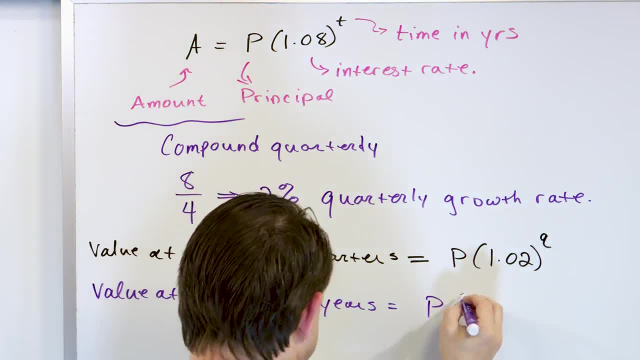 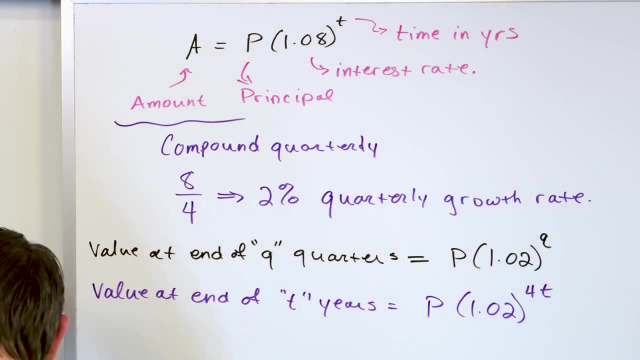 When I'm compounding quarterly like this Is going to be equal to the principal Times. one point, oh two. Now, instead of Q, you're going to have Four times T. Why are you going to have four times T up here? Why is this four times T? 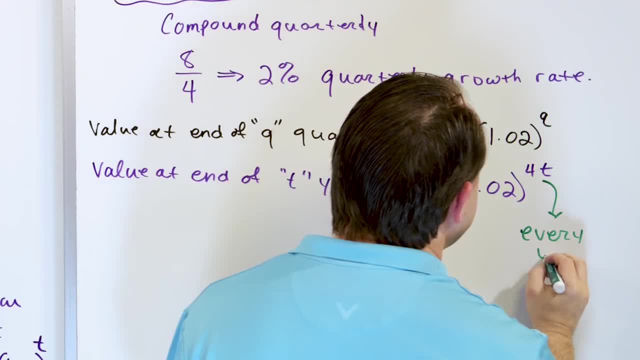 Because Every Year Has Four quarters. So this is where it gets a little confusing. You see, what happens is that I'm really doing an eight percent annual growth rate, But I'm going to compound it quarterly, So I'm really going to make it two percent. 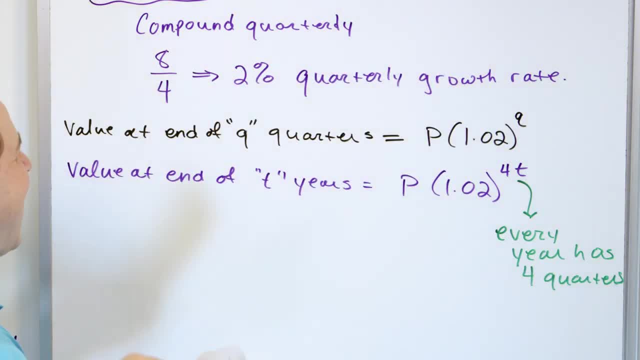 I'm going to give it to you every quarter. So this principle is time, this interest rate every quarter. So at the end of Q quarters. This is what it is. But the difference between this and this is, if I want to calculate it in years. 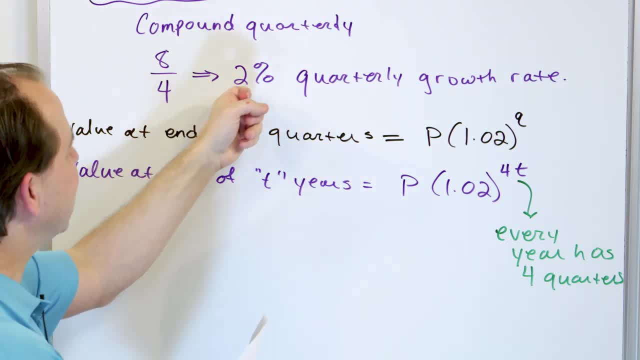 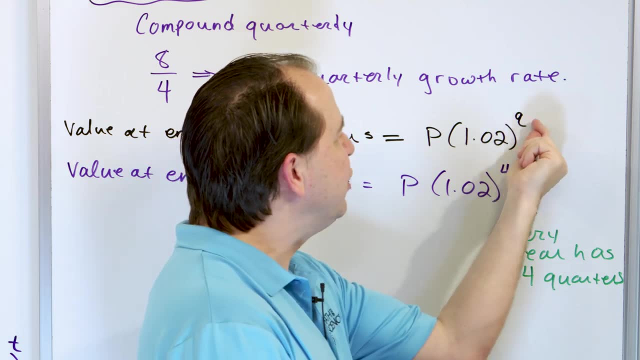 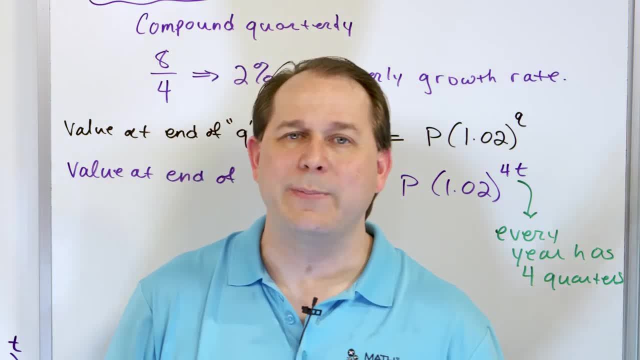 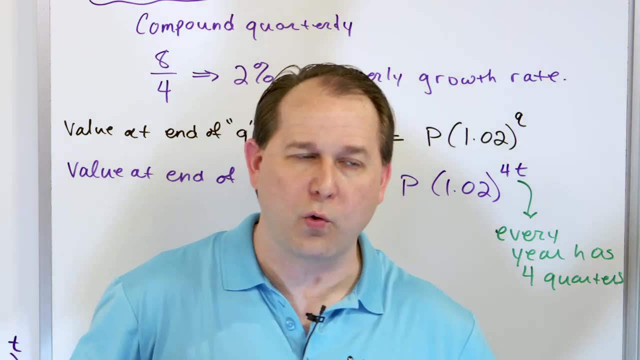 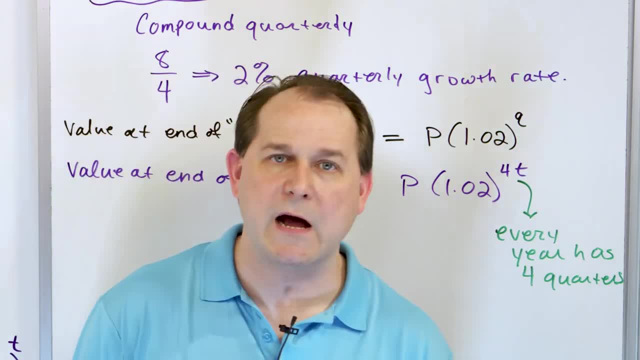 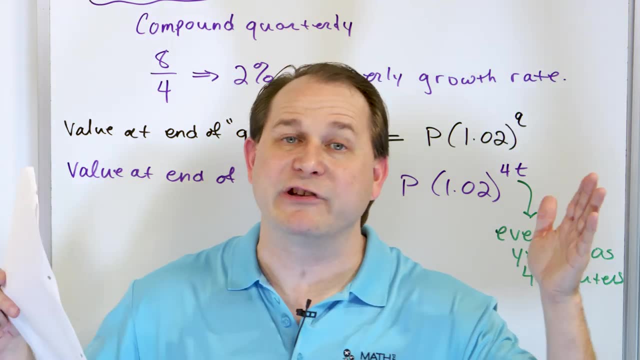 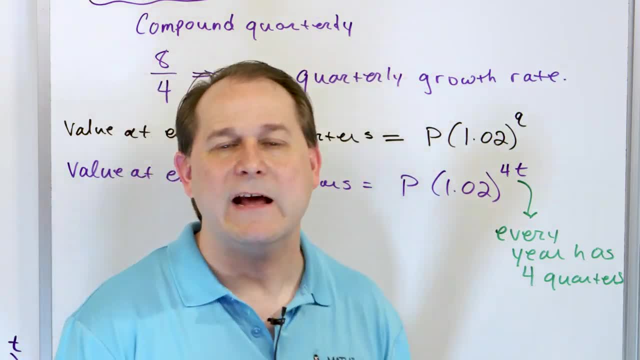 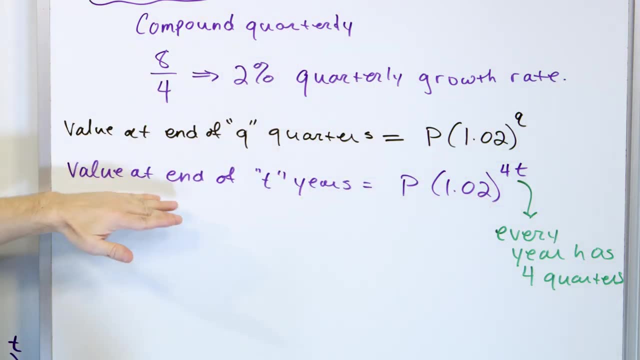 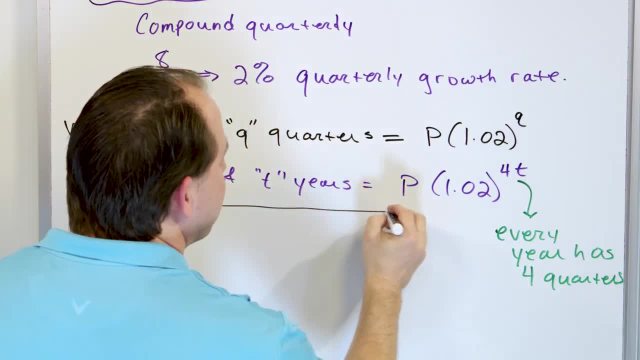 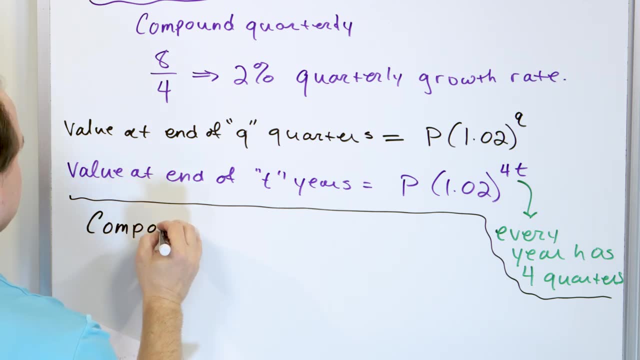 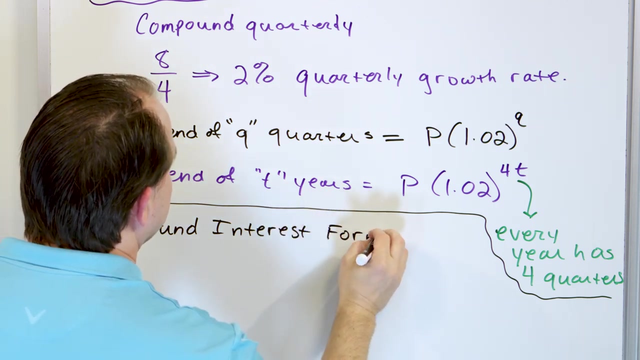 stuff. Because in every algebra book or every math book, finance book, whatever that talks about compound interest, you are going to come across the compound interest formula And, to be honest with you, I thought about just writing this equation down in the beginning and 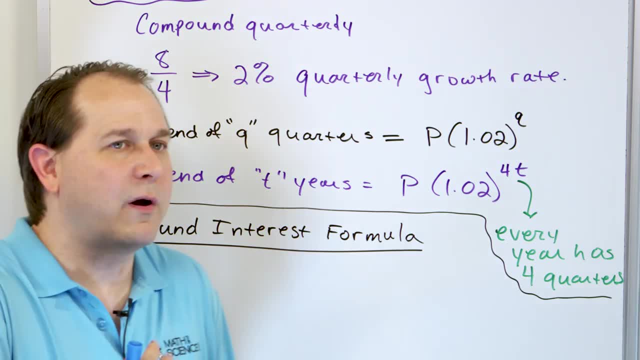 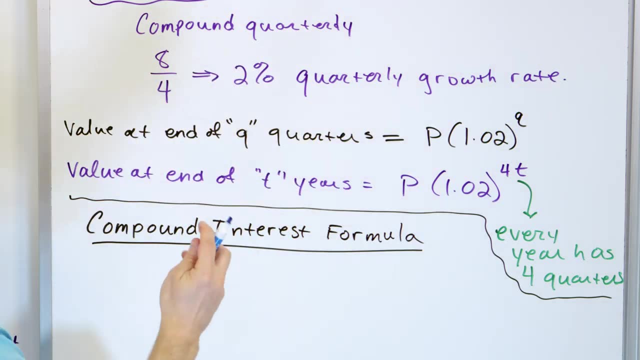 just being done with it. But the idea. the problem is, if I just throw it at you, you're not going to understand where it comes from. Now I'm going to write it down and you're going to very quickly understand exactly what it's saying. The compound interest formula goes like this: The value of 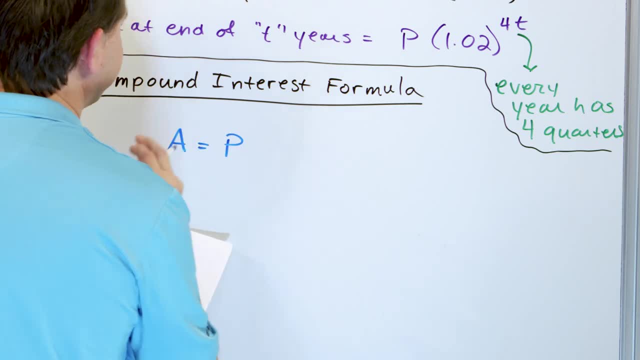 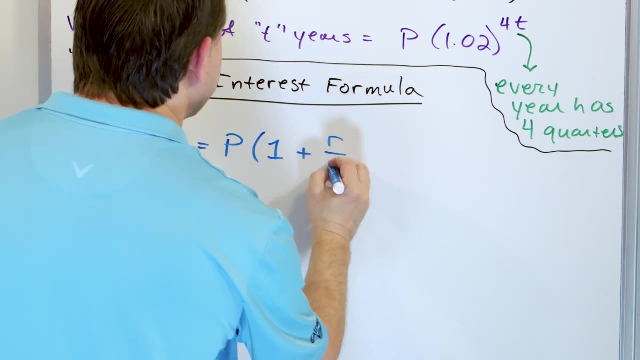 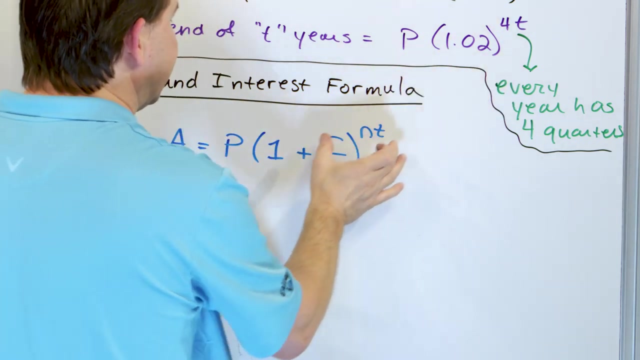 money that you have some point in the future is equal to the principle, which is how much money I put in to begin with, times a number One plus r over n, raised to the power of t. So I'm going to raise to the power of n times t. Look at how this thing compares with something like this: The one 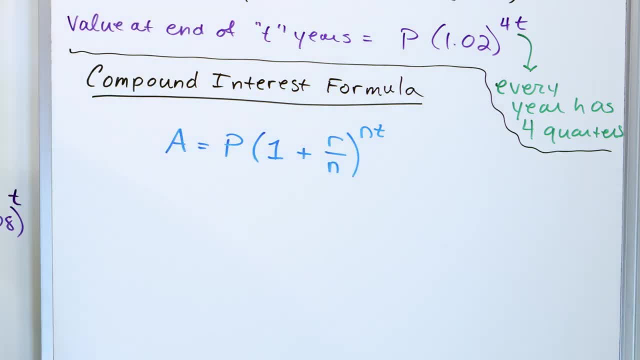 plus r over n is what's happening here. Let me write a few more things down here. Okay, The a is the amount of money that I have. The p is the principle. right, That's easy. The r is the annual interest rate. 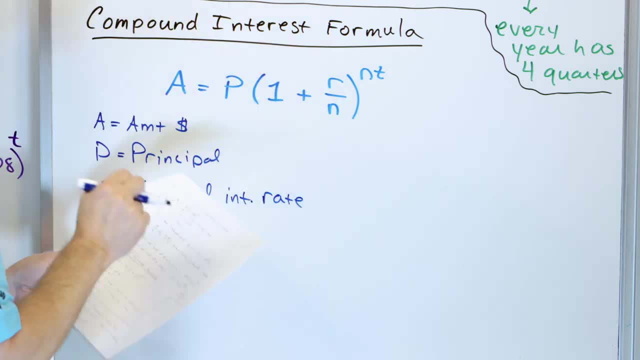 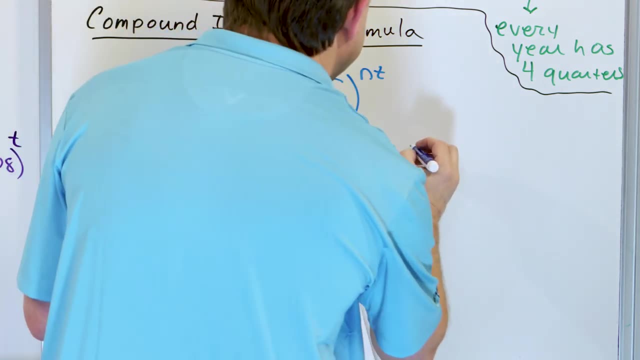 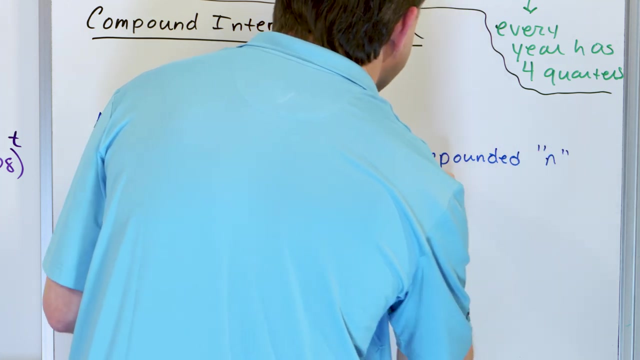 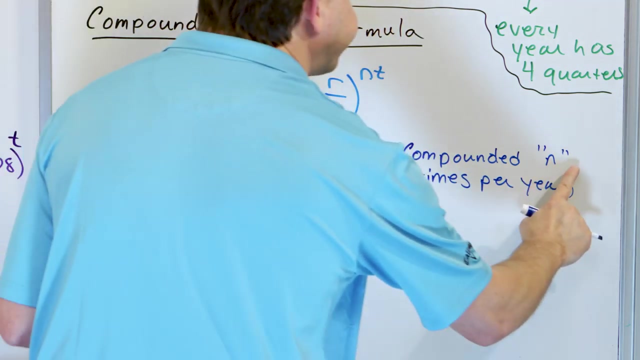 Right, That's the r. This is the number that goes in there for the annual interest rate, as a decimal expresses a decimal And the n means compounded n times per year. right, N times per year. So if I'm compounding quarterly, then I'm going to put a four here, and so on. 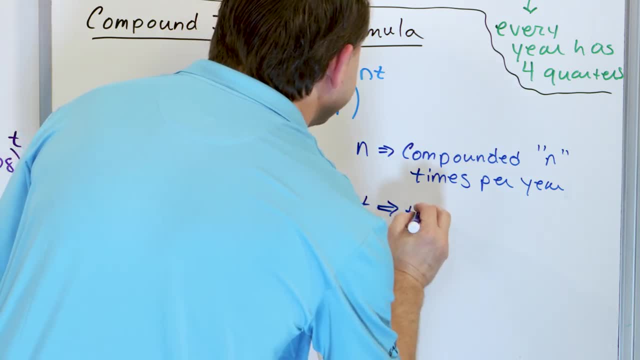 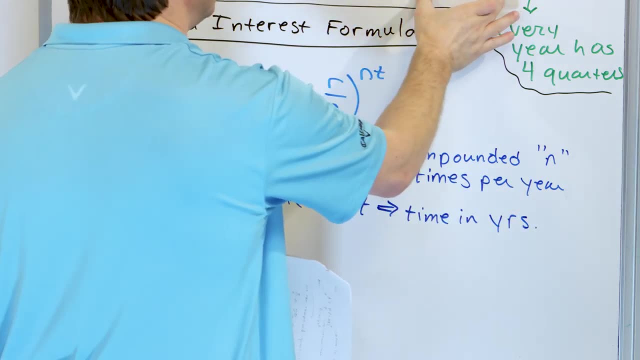 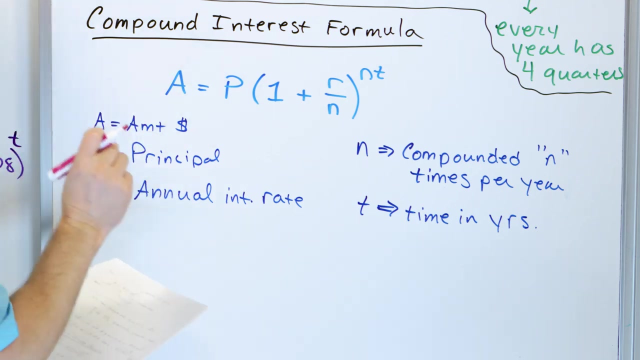 And then t is the time in years. All right, This equation actually gives: you can get this and you can get all these other ones from it. So I need to show you where that basically comes from. Okay, Let's say that I'm compounding annually. That means once per year, right, And the interest rate is what it. 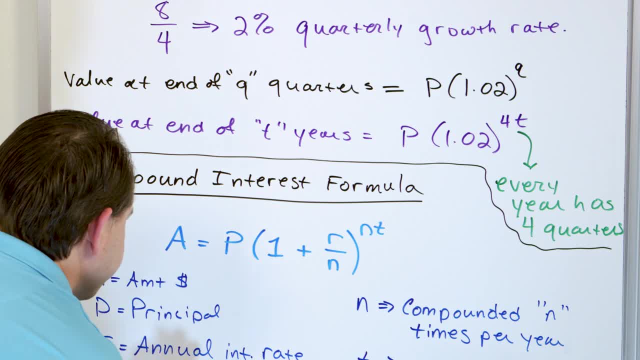 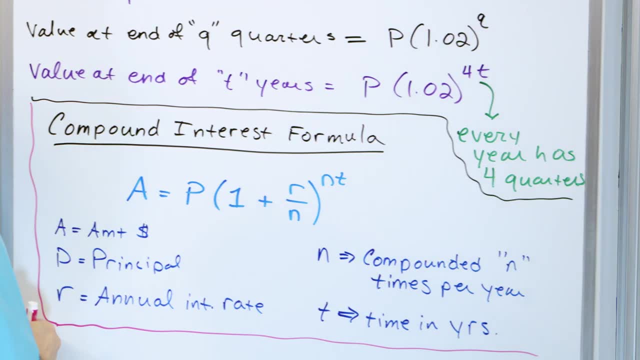 is. So let's just say that let me go ahead and box this. actually, Something like this: Actually, do I want to do this on this page? I think I want to do it on the next board. Let's say, let's first. 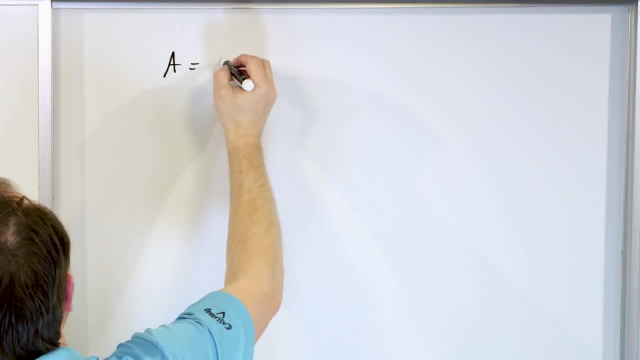 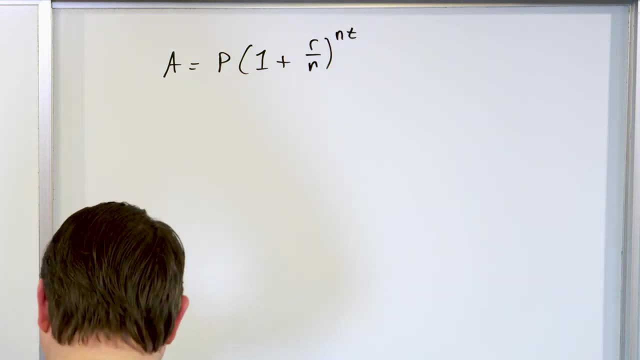 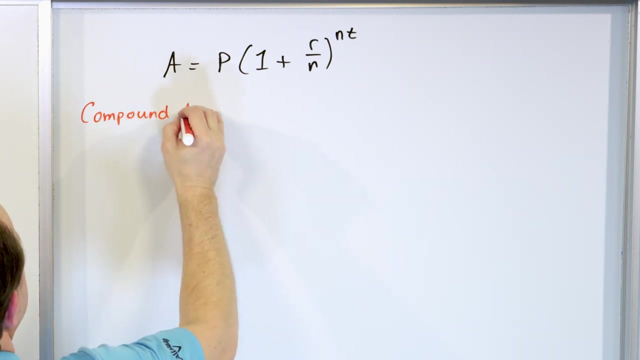 write down the compound interest formula. The value is the principal one plus r over n to the n t. All right, Let's say we compound annual, annual, annually, right? So the interest rate was 8%. Ah, I can't even write eight. It was 8%, which means the rate that you put into this. 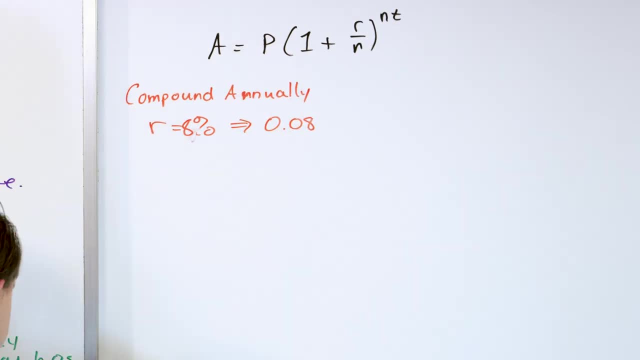 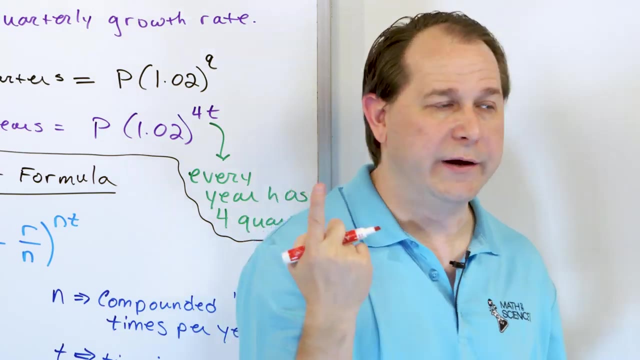 equation is 0.08.. But since I'm compounding annually, remember how it goes. N means it's compounded n times per year. So if I'm only compounding one time per year, then n is one right. So that means that n is equal to one. This is what we started the whole lecture with. 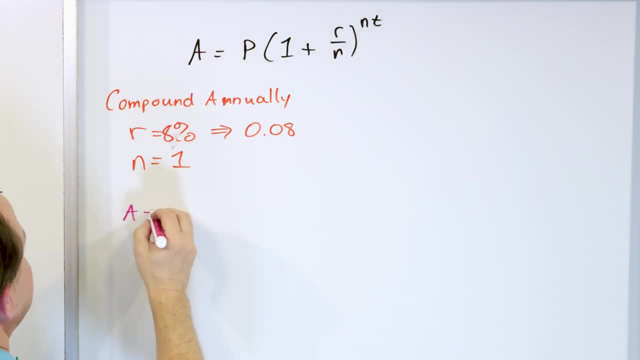 right. So if all this is true, how would this equation look? The rate is going to be the principal times one. So if I'm compounding annually, how would this equation look? The rate is going to be the principal times one plus one. plus, the rate is 8%, which is 0.08.. Always. 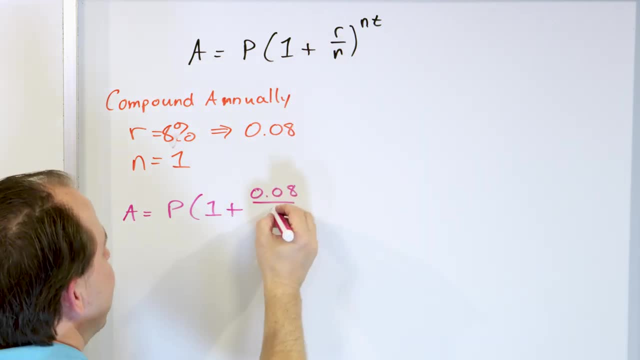 put it as a decimal divided by n times per year. I'm only compounding once. So it's divided by one and then raised to the power of n times t. n times t. What does this equation come out to? It's p times. when you divide this, you get 0.08.. It's 1.08 to the power of t. This is just t. 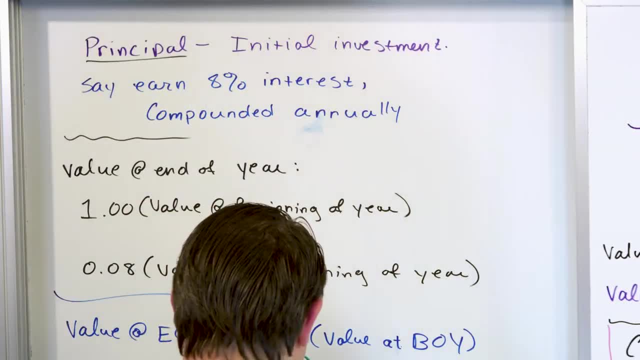 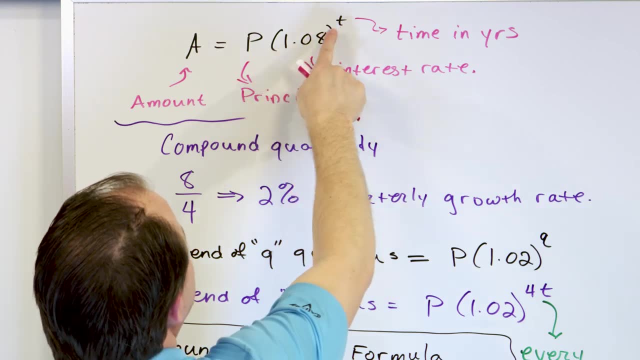 This thing is exactly what we started the whole lecture with. You see what I mean. Where is it out here: 1.08 times this. So then, yeah, here it is. It's p times 1.08 to the power of t. That's what it is. 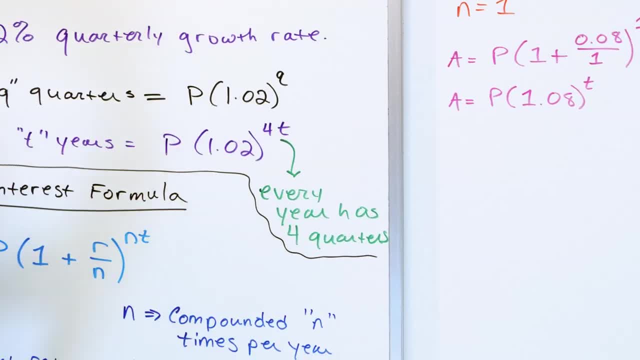 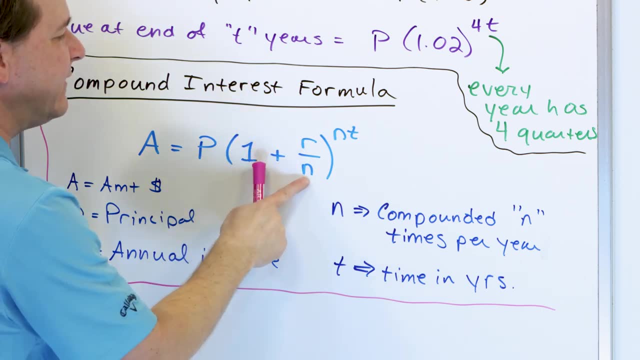 So all that's happening in this equation? when you look at this in your textbook, a lot of students do not know what this is saying. All this is saying is: I'm taking that annual interest rate and I'm dividing it by however many times a year, I'm compounding. 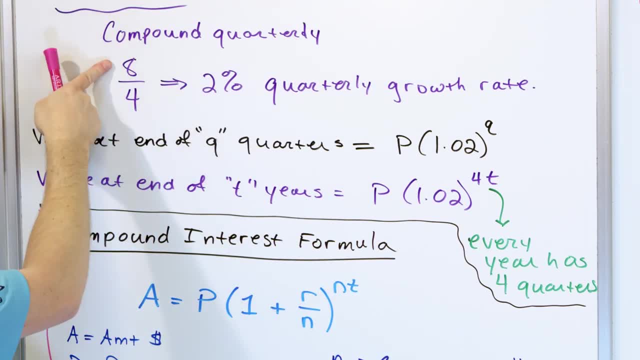 Because, just as I showed you right here, if I'm compounding four times a year, I'm not going to give you 8% every three months. four times a year, I'm going to only give you 2%. So this division. here is telling you what the rate is. So if I'm compounding four times a year, I'm not going to give you 8%. So if I'm compounding four times a year, I'm not going to give you 8%. So if I'm 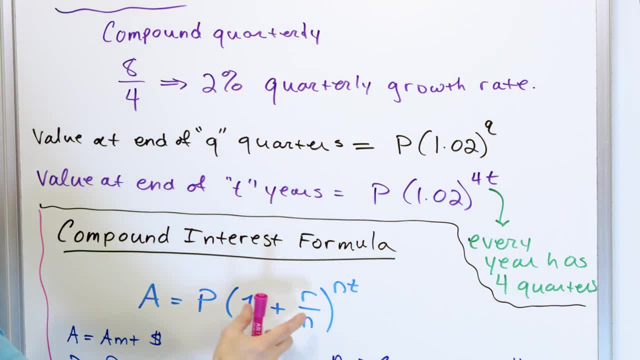 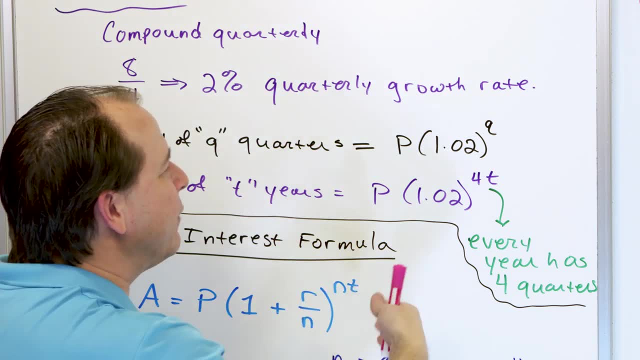 compounding four times a year, I'm not going to give you 8%. So if I'm compounding four times a year, this quarterly growth rate is. then I'm adding that here to get the new multiplier factor, the 1.02 in this example, And then the exponent is telling me how many compounding periods I have. 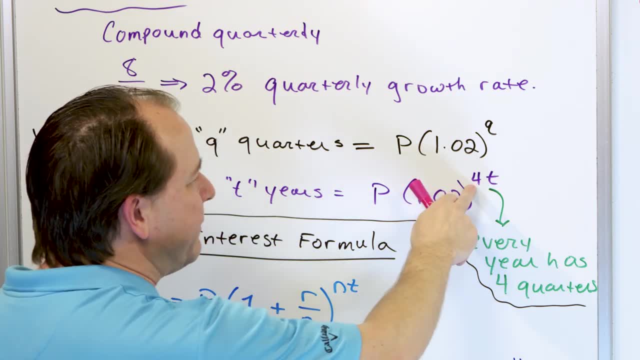 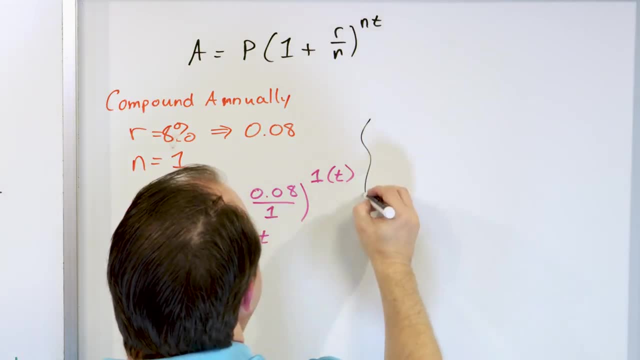 If I'm putting years in and I'm doing it quarterly, then what's going to happen is I'm going to have four compounding periods, So it has to be raised to the power of four. So let's go over here and see what happens if I compound quarterly. 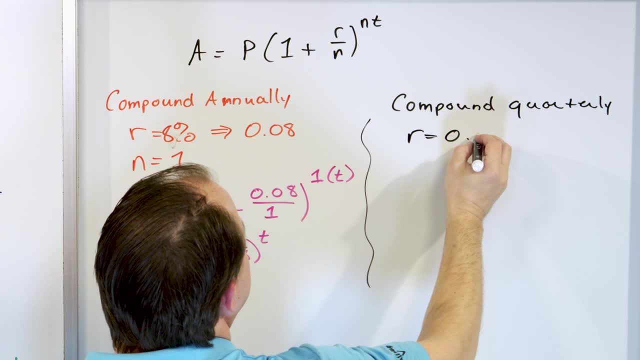 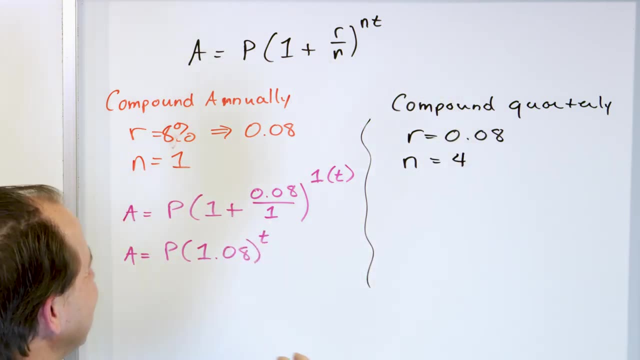 Right, It's the same sort of thing. The rate is 0.08.. But now I'm compounding four times a year. So I'm compounding where n is equal to four, It's compounding n times per year. So what it's going. 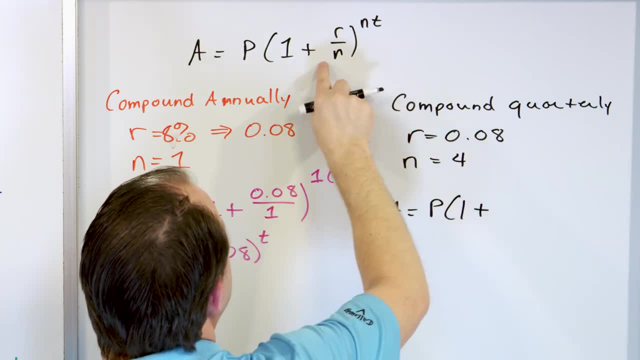 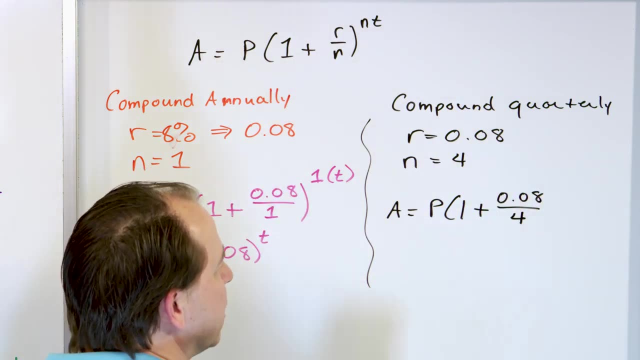 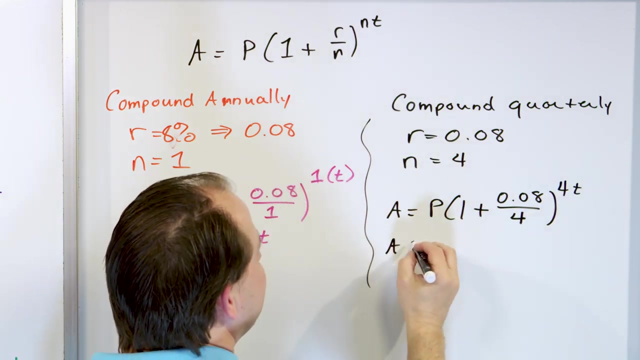 to be is the principal times one plus what do I have here? The rate 0.08.. That's the annual rate compounded four times a year. This is doing the division, giving me that smaller percentage. And then the exponent here is n times t. This is four times t. Notice, this is exactly what we said. 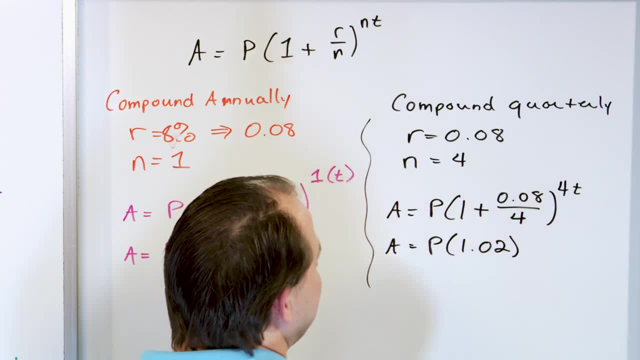 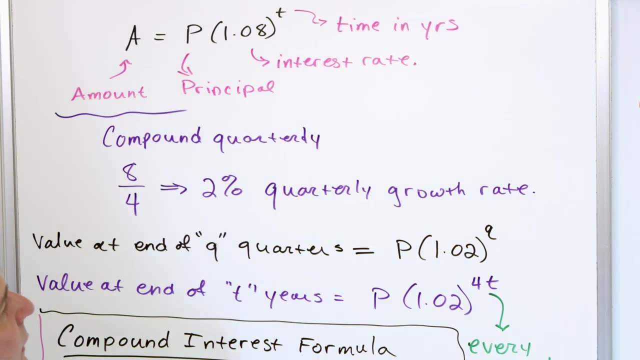 this is p times 1.02.. Then you divide this out here You get 1.02 to the power of 4t. That's exactly what we talked about. Where was that Compounded quarterly? What was it at? Yeah? 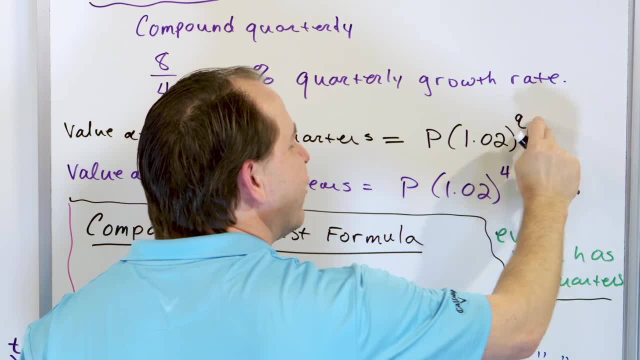 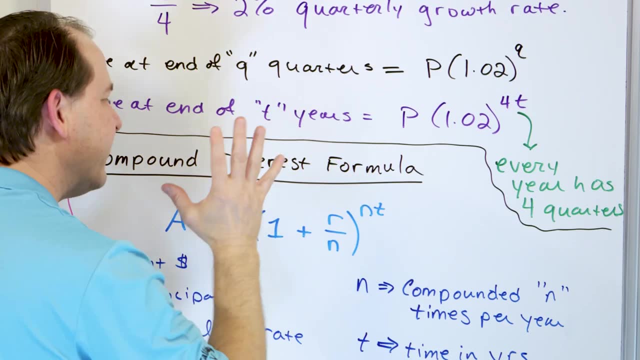 right here. Compounded quarterly. This is if you're just going to talk about it in terms of number of quarters. This is going to be what happens if you talk about it in terms of the number of years. Okay, So when you see the compound interest formula the way you should, 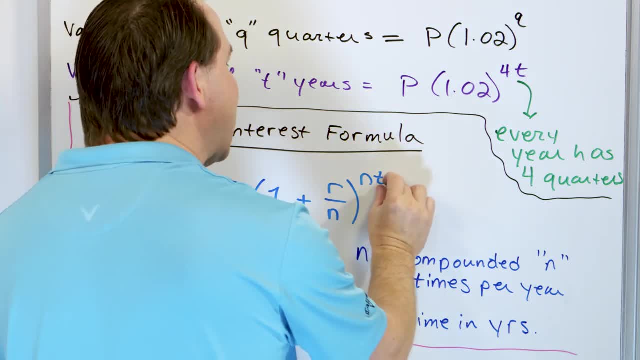 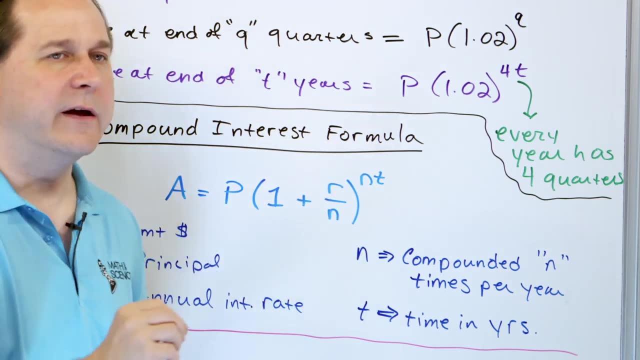 read it as follows: The exponent up here has the time variable. That means it's an exponential function that's going to grow like an exponential function. The division here is just because if I'm not compounding annually, I need to figure out what. 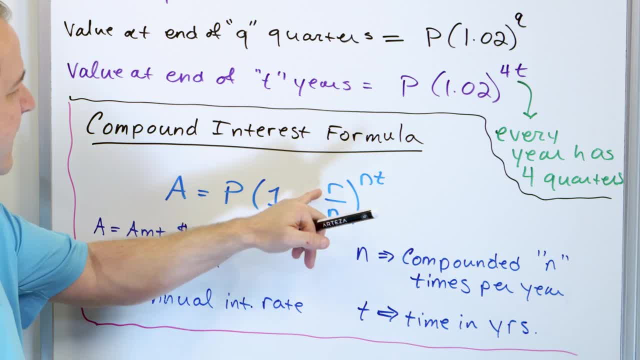 the new rate is that I'm giving you quarterly. So I divide it by the number of compounding periods to get a smaller interest rate. Then this one plus ends up giving me the multiplier factor. in here The exponent has to have the number of compounding periods per year times the number. 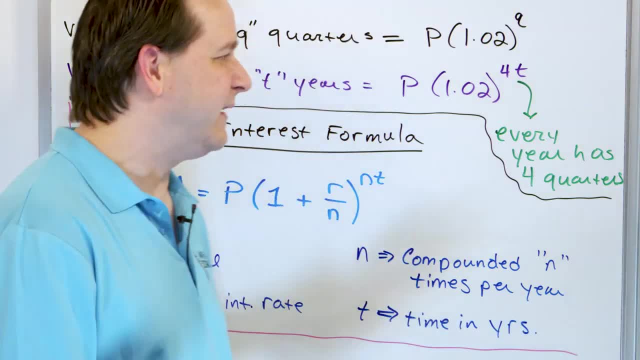 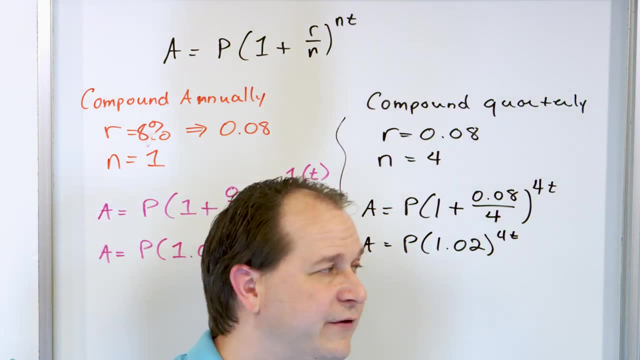 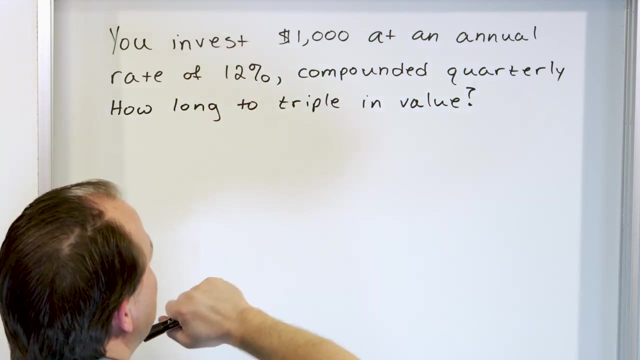 of years. So this exponent is just how many compounding periods I have altogether. All right, that's it. That's all you have. So what I want to do is at least work. one problem here, to give you a little bit of practice. Okay, Here's the problem. You invest $1,000 at an 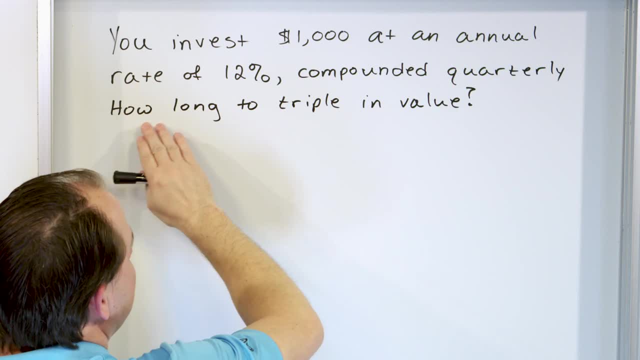 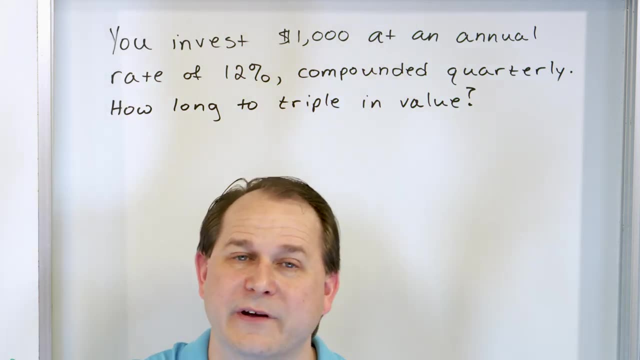 annual rate of 12% compounded quarterly. Compounded quarterly: There should be a period right here. How long does it take to triple this thing in value? So what you have to do when you're confronted with a compound interest problem is to first write down the compound interest. 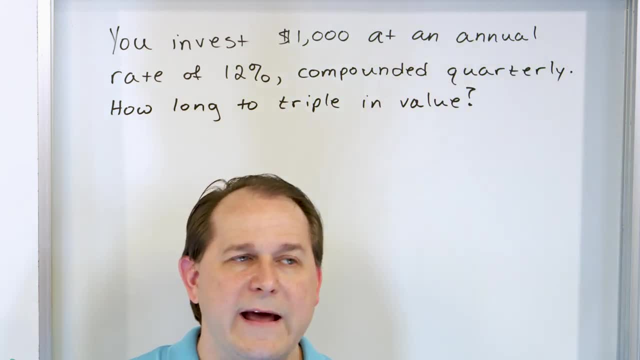 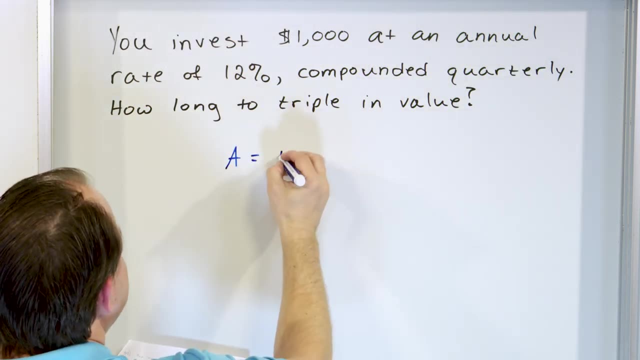 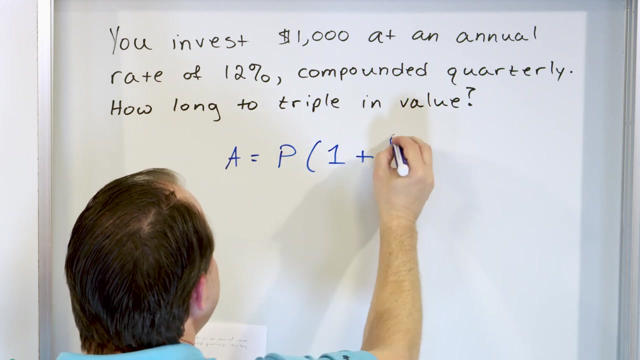 equation and then identify what in the problem you're given, and then the rest of it will fall out. So let's start by doing that. The value of my money in the future is going to be equal to the value of the money that I start with. times some factor, The factor is one plus, whatever the 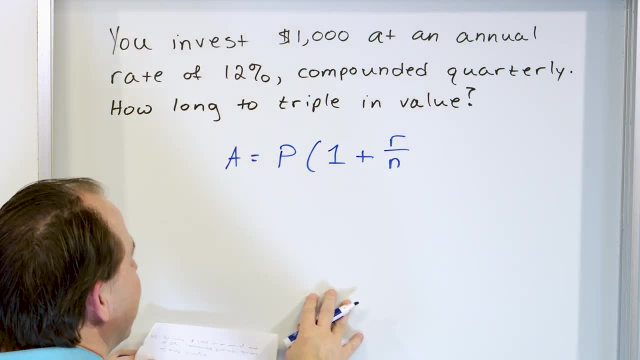 interest rate is divided by however many compounding periods, I have to give me kind of a new lower rate raised to the power of n times t. This exponent is the total number of compounding per year times the number of years. So when you multiply you get the total number of compounding. 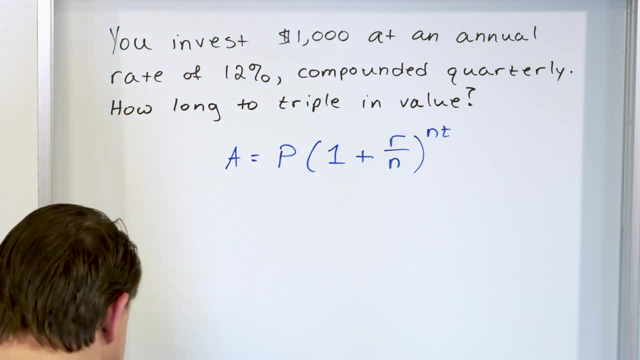 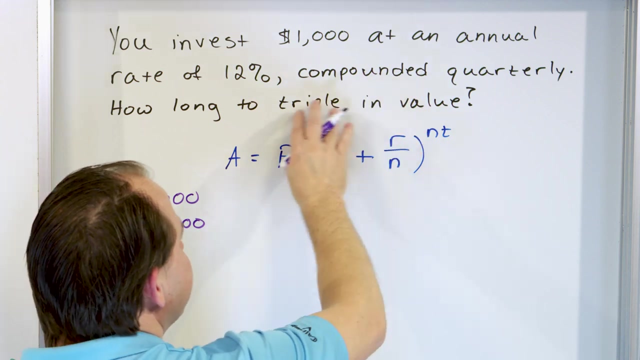 periods I have Now. in this case, we are given that the principal is $1,000. But we're trying to figure out how long it takes to triple in value. So the amount down the road that I care about is three times that It's given to you by telling you it's trying to triple in value. 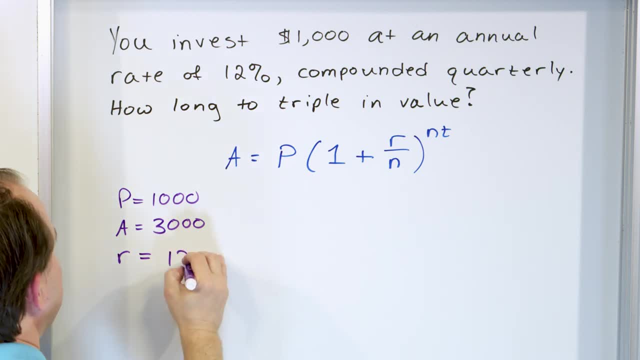 The annual rate, which is always r, is 12%. But you never, ever want to put a percent in a math equation ever. You never, ever, ever, ever, ever put a percentage in like that. You always convert it to a decimal 0.12.. And then it tells you it's compounded quarterly. 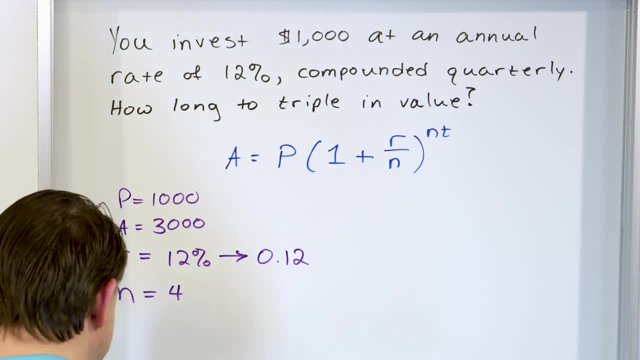 That means n times per year. So n is equal to 4.. So now, at this point, we have to go and put everything into this thing. Let's see what it looks like. The amount that I'm going to have down the road is $3,000.. The amount that I start with is $1,000,. the principal. 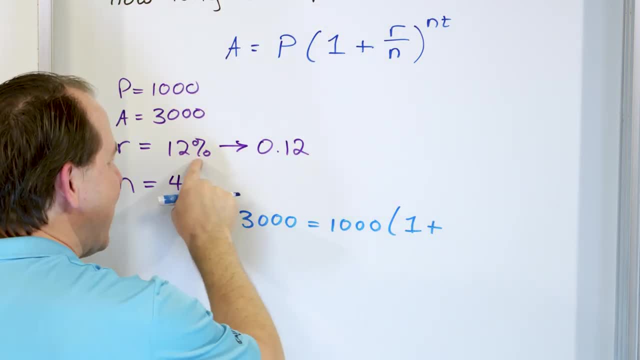 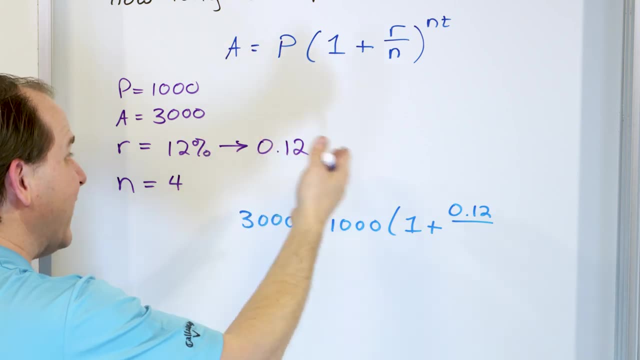 Inside of here I have one plus the rate, which is 12%, but I never, ever want to use this. I always want to do 0.12.. I'm dividing it by 4, because I'm actually compounding this four times a year. So I'm going to actually have a smaller interest rate than I'm compounding. 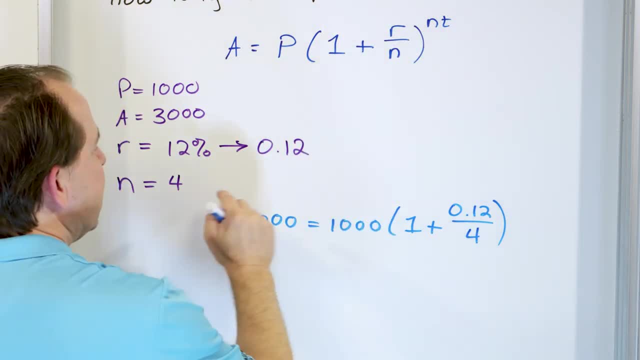 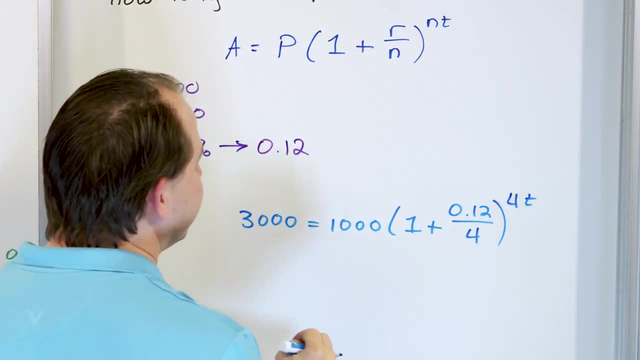 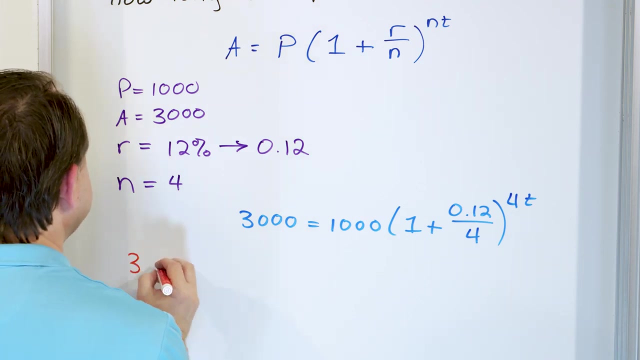 more frequently. And then the exponent n is 4 times t, And I'm trying to figure out: how many years down the road does it take to do this? So then what happens? I divide by 1,000.. And over on the right-hand side I'm going to have a 3.. And then, inside of 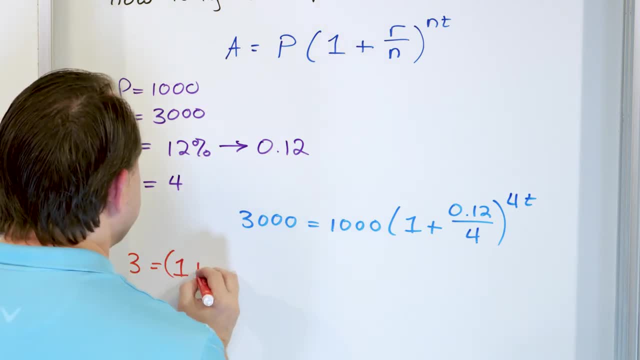 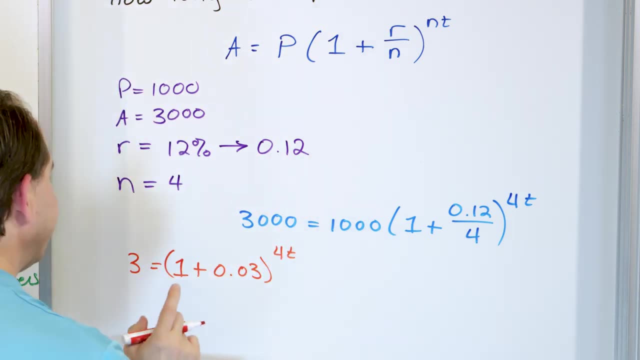 here it's going to be 1 plus when you divide this, you're going to get 0.03 to the power of 4t. So what you're going to have when you flip everything over here- a better way to. 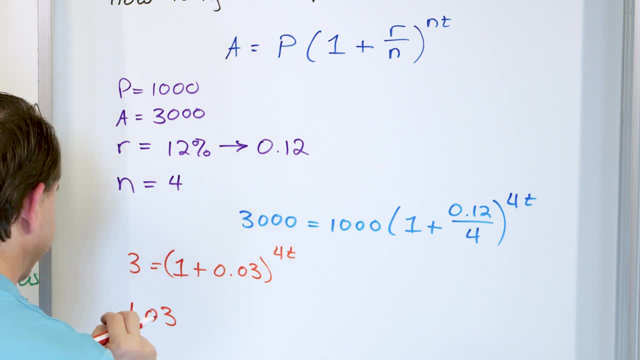 write, it is 1.03.. When you add these together you get 1.03.. That's kind of like the new effective number you're multiplying by every quarter to the power of 4t is equal to 3.. I just wrote this side on the other and moved the 3 to the other side. This is an exponential 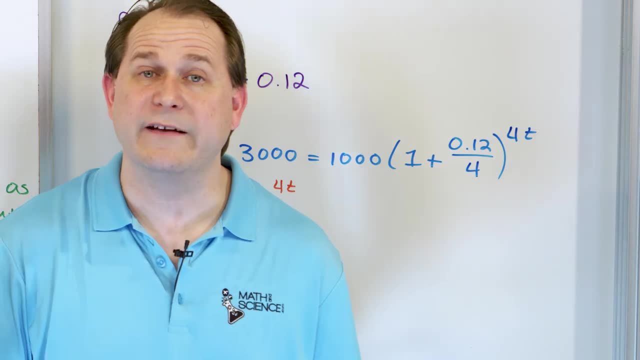 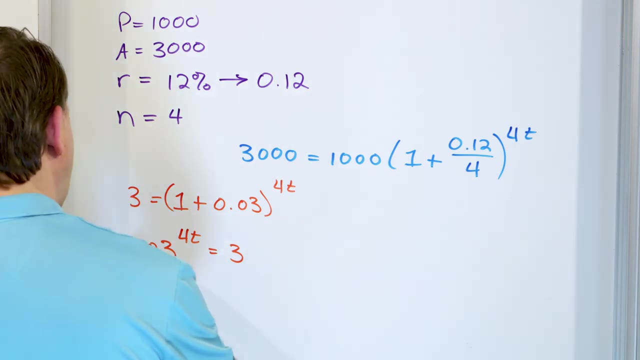 equation. We know how to solve exponential equations now. There are several different ways, but the easiest way is to take the logarithm of both sides. The logarithm of both sides Because when I take the log then I can pull the exponent. 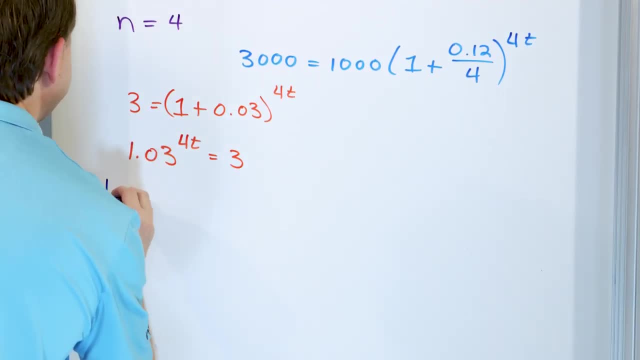 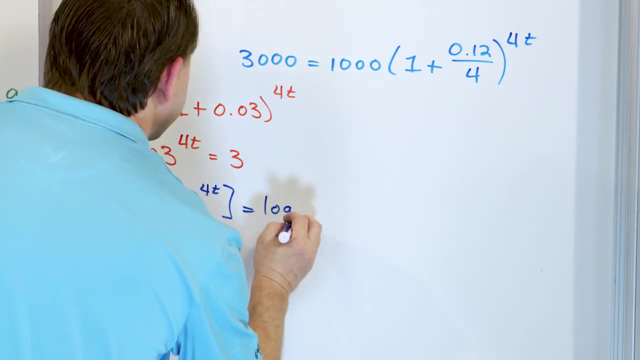 out. So you can do whatever base log you want. but I'm going to do a base 10 log of 1.03 to the power of 4 times t is equal to the log of 3.. Take the logarithm of both sides. 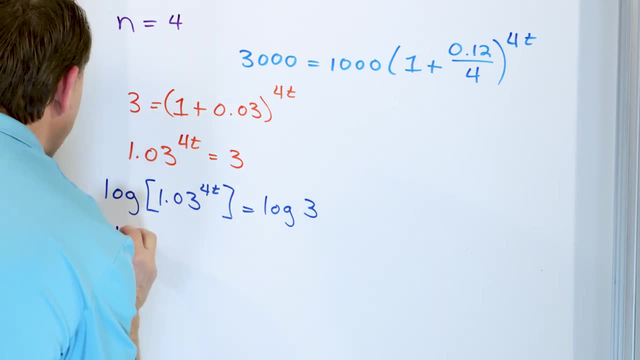 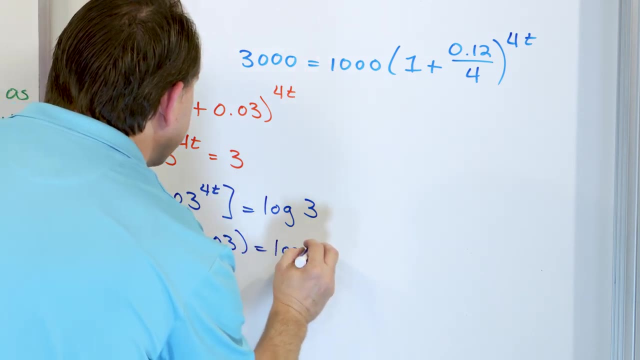 Now why do I do that? Because when I take the log of this, the exponent can come out, So I'm going to take. the log of 1.03 is equal to the log of 3.. So now I can solve for t. 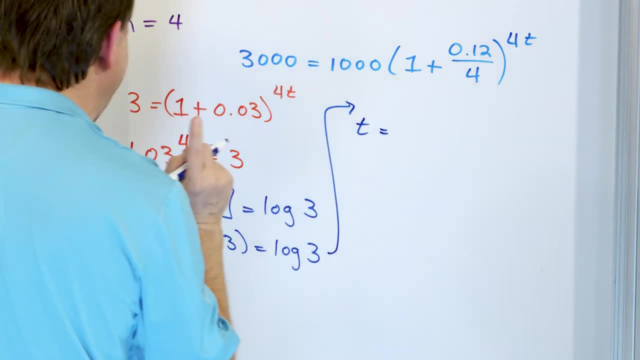 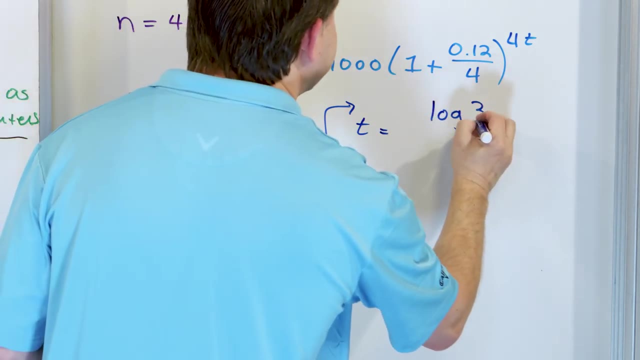 So what's going to happen here? let's go up over here t as an exact number. when I divide by the 4 and I also divide by the log, here it's going to be the log, the base 10 logarithm. 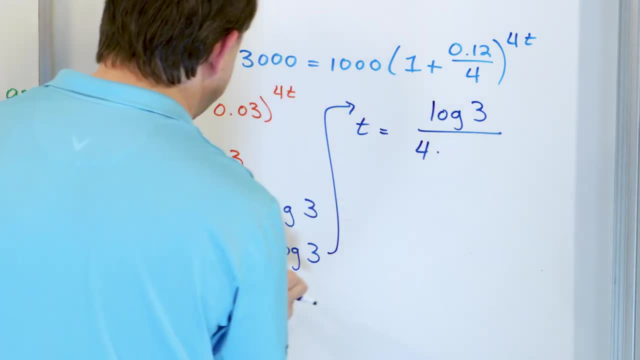 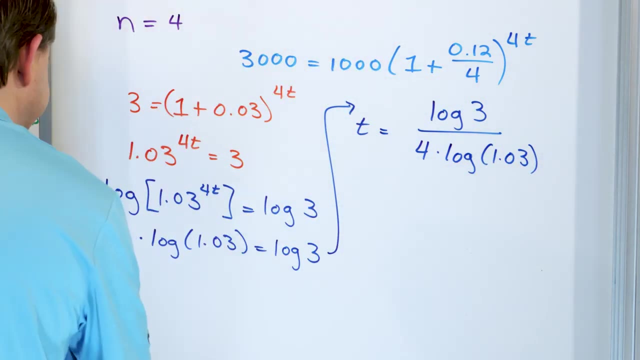 of 3, divide by 4, divide also by the log of 1.03.. So in your calculator you can go do a base 10 log Of 3 and a base 10 log of this, and you know what the number 4 is. so then you can calculate. 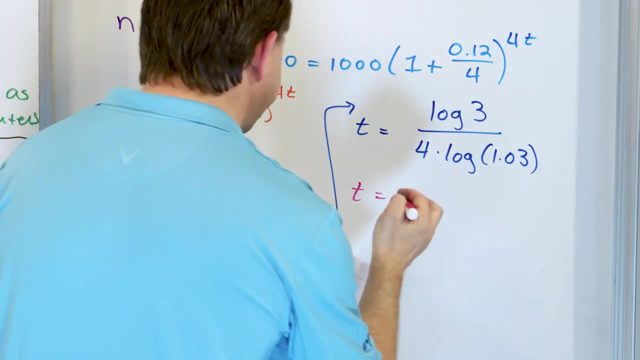 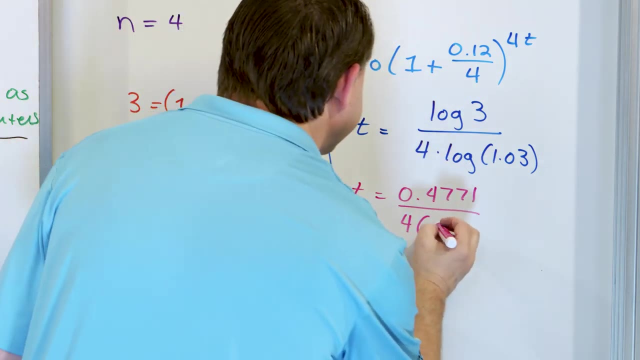 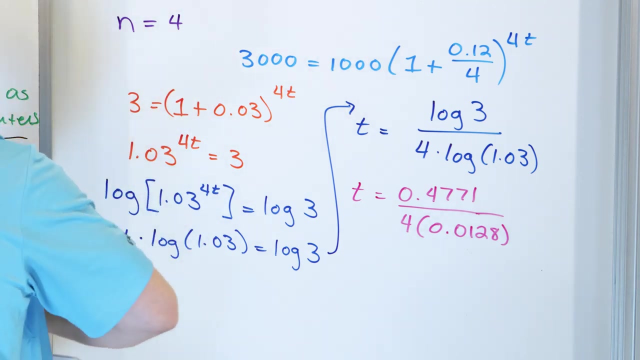 this. So what you're going to have then what is the base 10? log of 3? You're going to get 0.4771.. And then log of 1.03, you'll get 0.0128, like this, And then whenever you do the division. 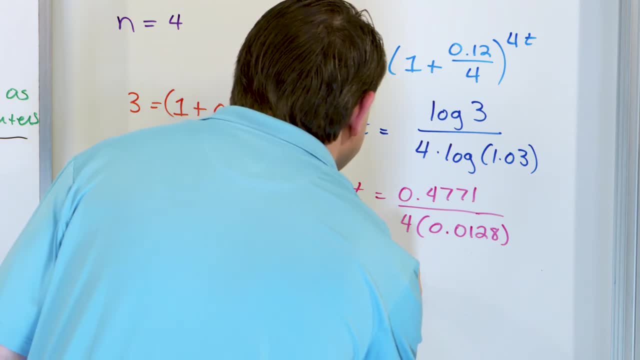 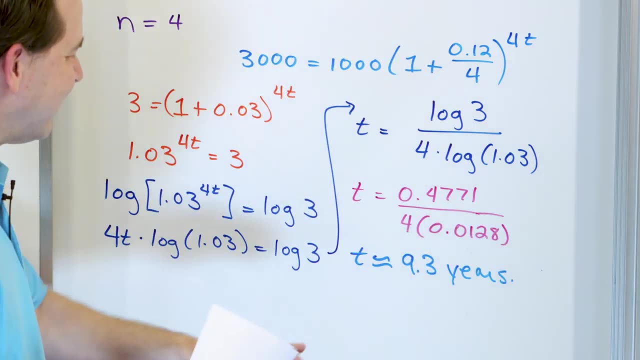 this divided by the multiplication of those two things you're going to get when you round the decimals here: 9.3 years. Now. you're tempted to circle this because that's how long it's going to take to triple in value. However, if you actually circle this, I'd probably give you full credit. However, 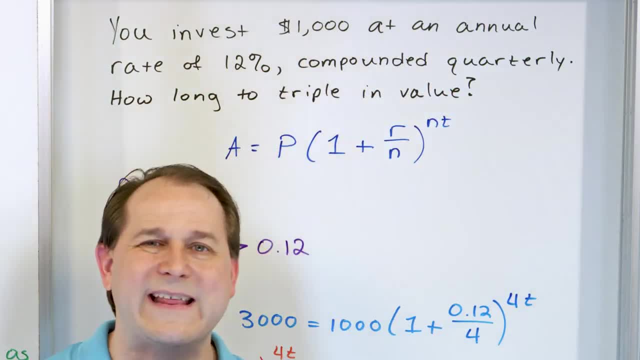 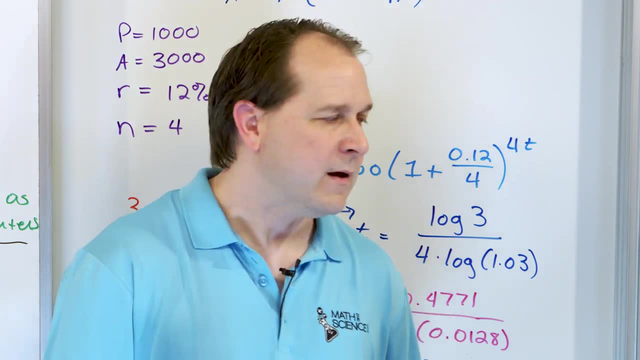 this thing is telling you that the interest is compounded quarterly. That means you only get the money every three months. That's when the new calculation happens. It comes into your account every three months, But the answer that I said is it's going to triple in value. 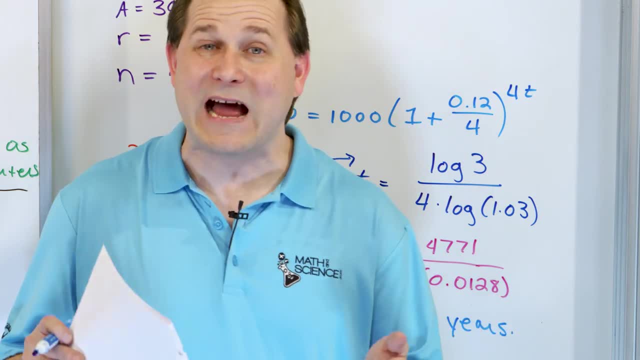 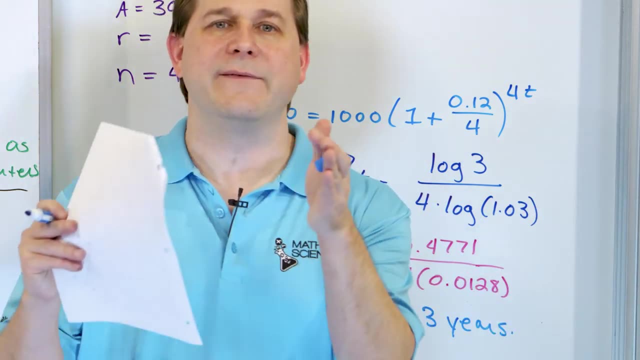 in 9.3 years. But a quarter of a year is actually 9.25. And then the next time I get money is another quarter, which is 9.5.. So it's 9.25,, then 9.5,, then 9.75,, then 10 years. That's when I get. 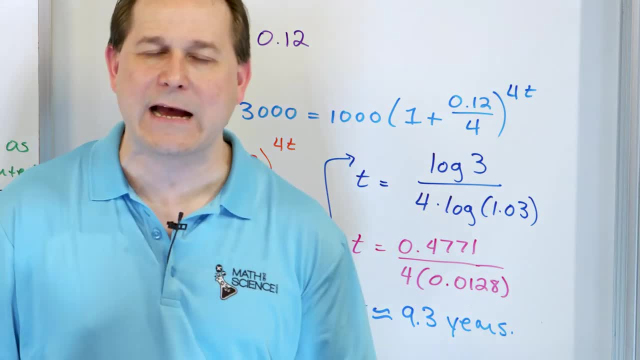 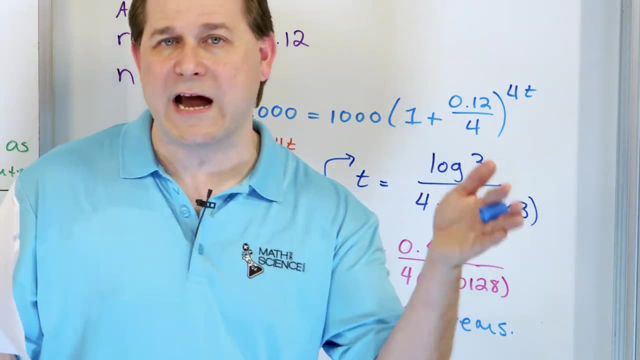 the money. So it really I'm not going to actually have triple the money in 9.3 years, because I don't. if I, you can really only get money at either 9.25 or 9.5.. But if I pick 9.25 as the 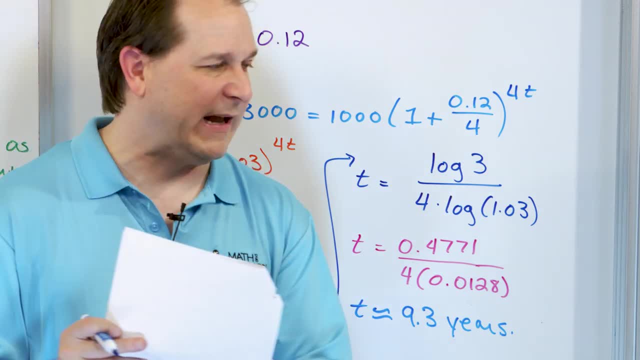 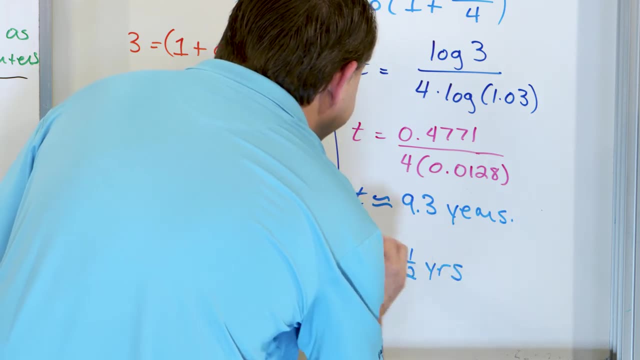 answer. I'm not going to quite have triple the money. I'll have a little bit less. So I'm actually going to say that it's going to be basically in 9.5 years. I think this is the best answer. You. 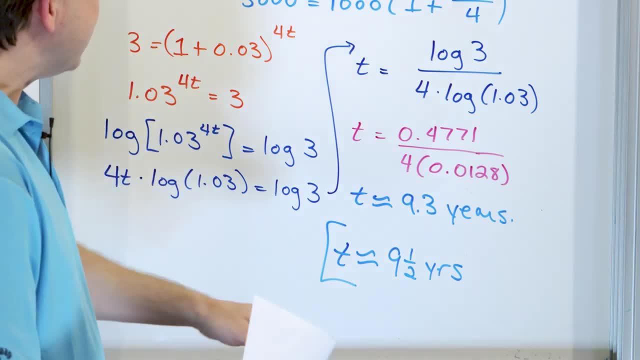 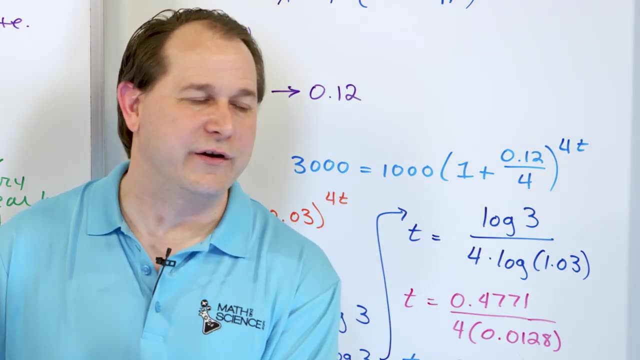 could say: this is the exact answer. but since it's compounded quarterly, if I wait till 9.5 years, I'm going to have slightly more than triple the value of this money. If I were to wait to just 9.25 years, which is actually closer to this number, I wouldn't quite have triple the value. 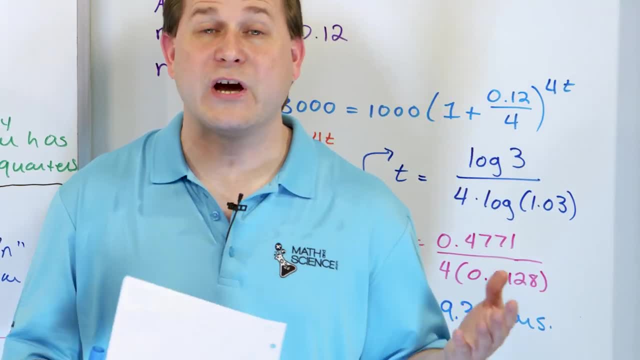 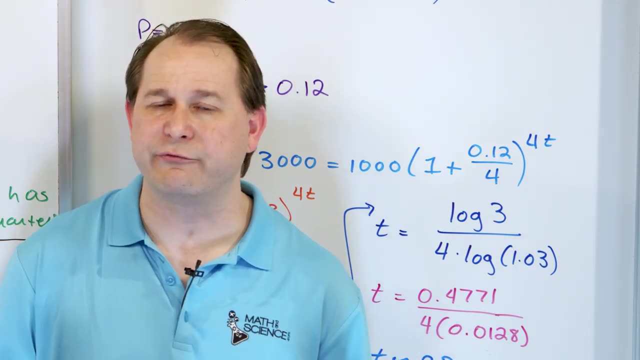 So I think this is the better answer. So we have covered one of the most important ideas in all of math. Einstein called it the eighth wonder of the world, Because if you understand how compound interest works, you can use it to amass great wealth and 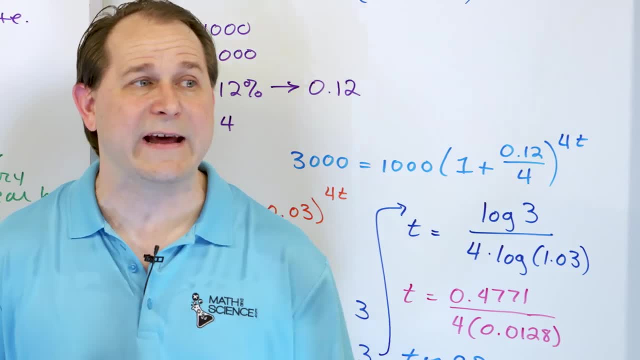 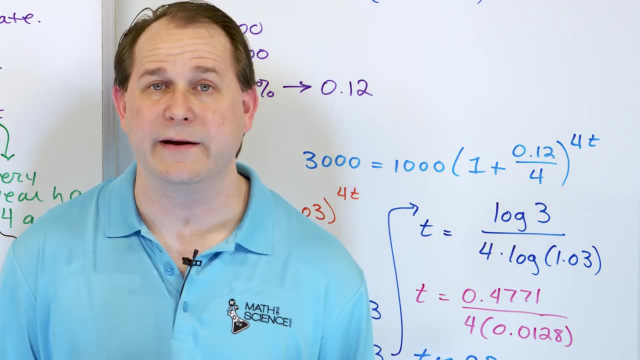 prosperity for yourself and your family. If you don't understand how it works, then you take out a bunch of credit cards and say, oh, I'll just pay them later. And then, 10 years down the road, you have so much crippling debt you can never ever get out from under it. So what I want to 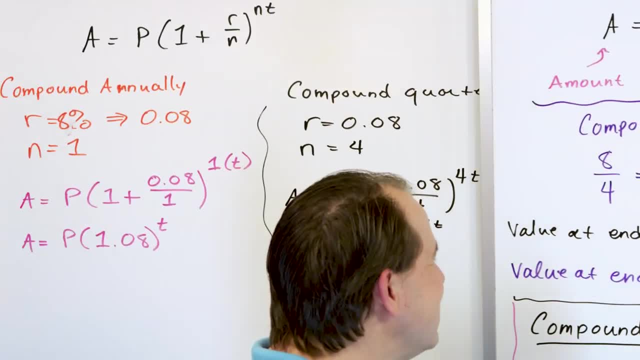 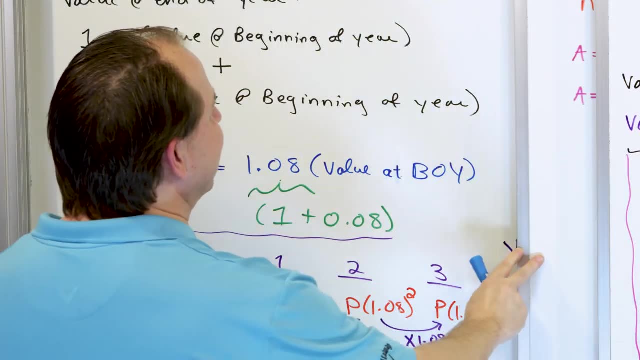 understand, and make sure you understand, is that the growth of money like this is not a straight line. It is not a straight line. It is an exponential curve that goes up. right. And the reason it's an exponential curve that goes up is because when you have a lot of money, you have a 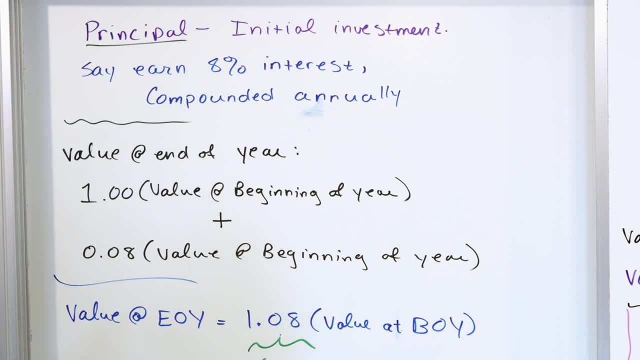 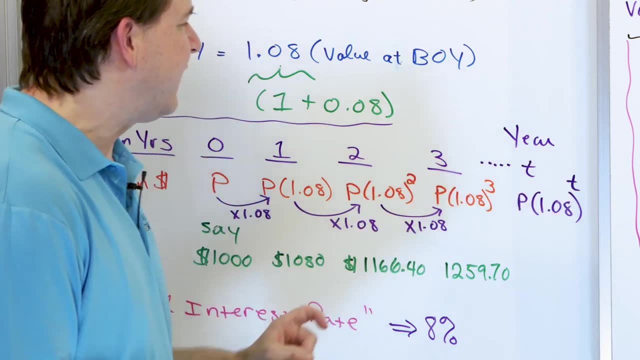 lot of interest. So when you take a principal and you multiply every year with some multiplier factor- that includes your interest rate- what's happening is you're increasing the exponent every year And that means it's an exponential curve, which means it's going to go up as an exponential. 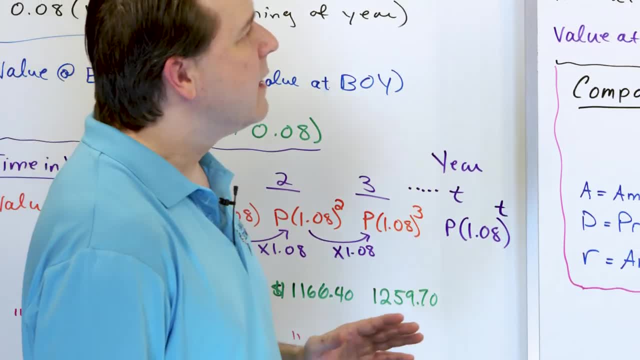 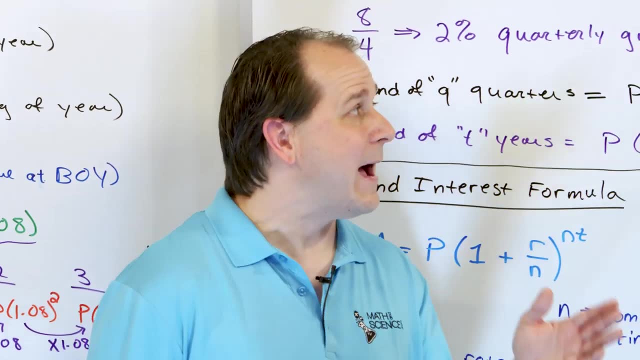 Now that's called an annual interest rate with annual compounding. But oftentimes interest is not compounded annually, It's compounded quarterly. But I'm still not going to give you that 8% every quarter. I'm going to take that 8% divided by four and I'm going to 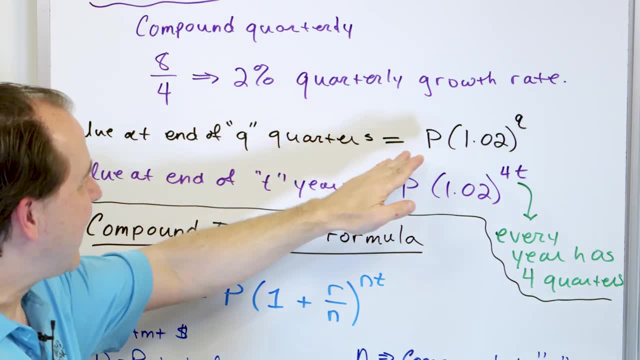 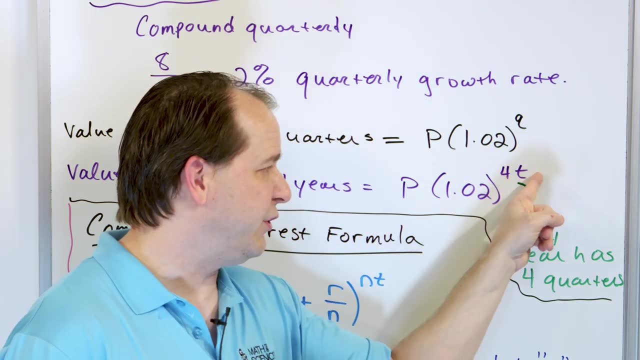 give you 2% every quarter. So that's going to go up as an exponential curve And that's going to. the formula is exactly the same, but the number in here is now smaller. but I'm doing it more often because I'm not doing it every year. I'm doing it four times per year, So the exponent is four. 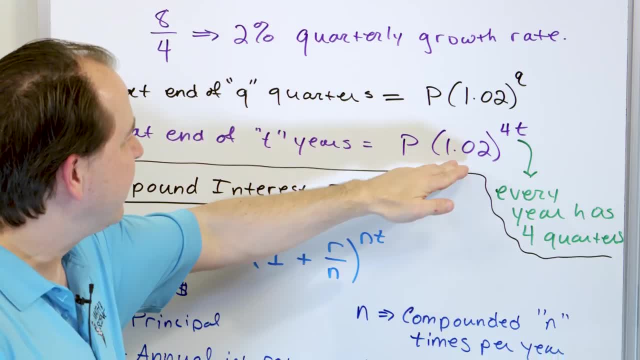 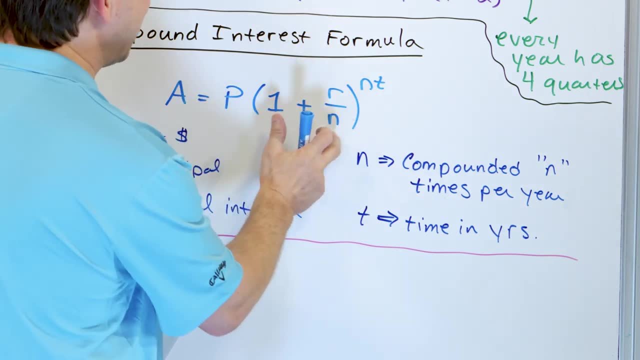 times bigger because I'm doing it four times more often. This is what I tried to do in terms of numbers, to make you understand what the compound interest formula is doing. Your principal times this multiplier factor. This is the new interest rate that comes from taking the annual rate. 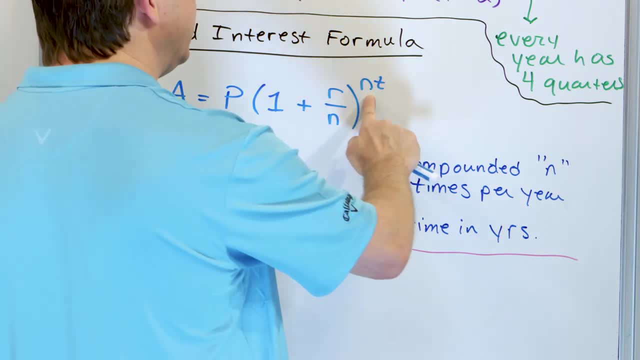 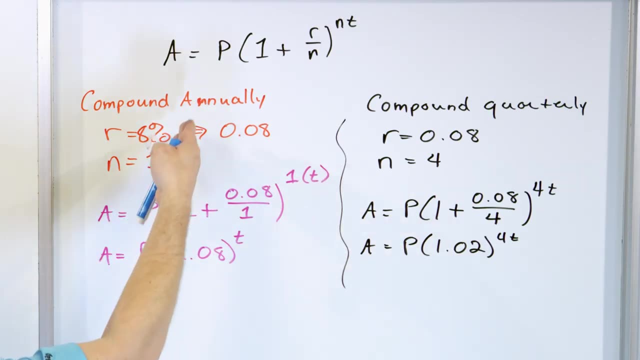 divided by how many times I'm compounding per year. The exponent is again how many times I'm compounding per year times the number of years, And that is how, if you're doing an annual thing, you can get exactly the same equation as we derived already. 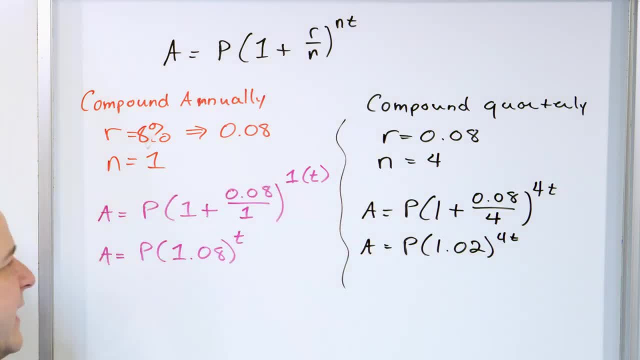 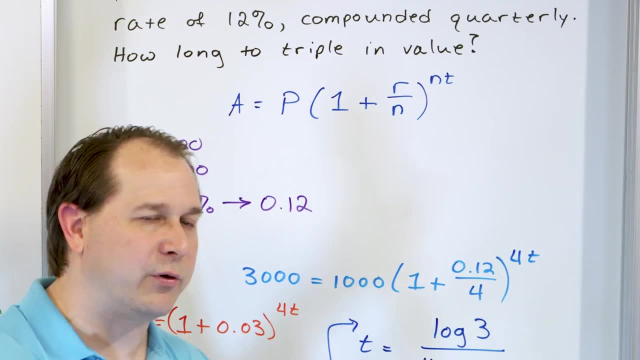 before. If you're doing a quarterly thing, you get exactly the same equation as we're deriving before. And then of course, we did our problem where we had to put in the value of money the value we started with and backwards calculate. So oftentimes you have to use logarithms to get. 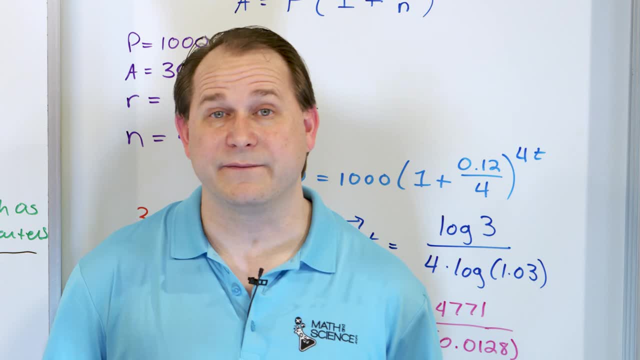 to the final answer. I would encourage you to watch this video a couple of times, because if I could put one piece of money in here, I would be able to do it, And if I could put one piece of knowledge in people's brains that could help them in their everyday life, it would be the 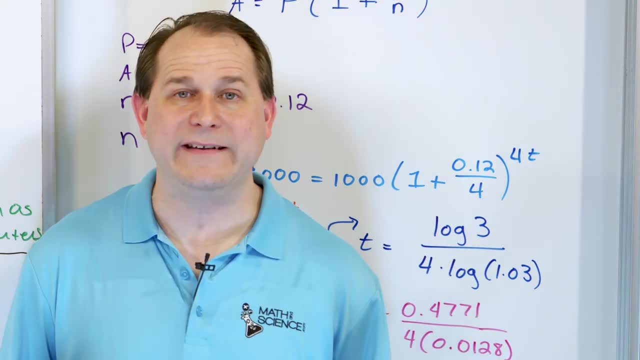 knowledge in this lesson. You don't know how many people out there have no idea how money actually works, And so when you go out and you buy a car or a house that's way more expensive than you can afford And you're paying that interest on a home that you can't afford, Then you may not understand. 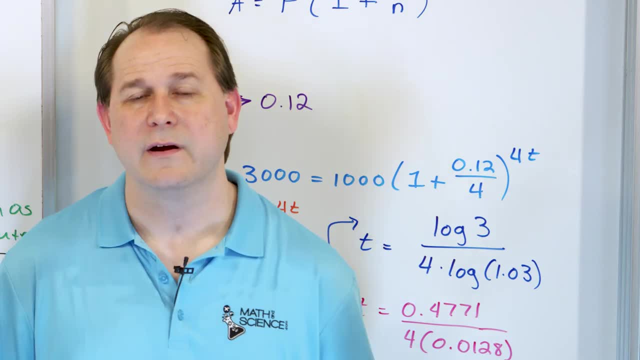 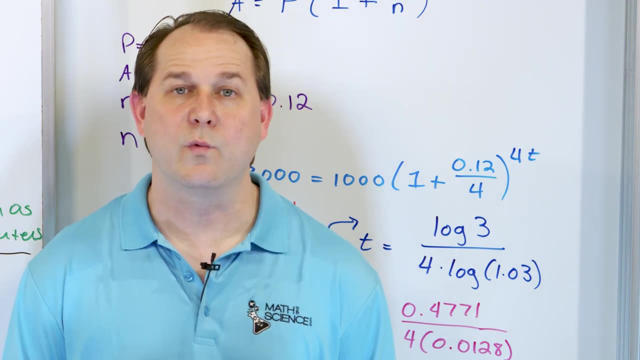 how in deep trouble you can be until much, much later down down the line. So I want you to understand, solve these problems, make sure you conquer this and understand it with me. Then go on to the next lesson, where we'll continue. 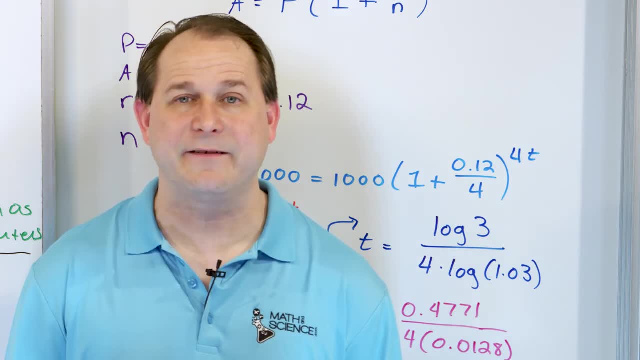 Continue working compound interest problems dealing with the exponential growth of money.